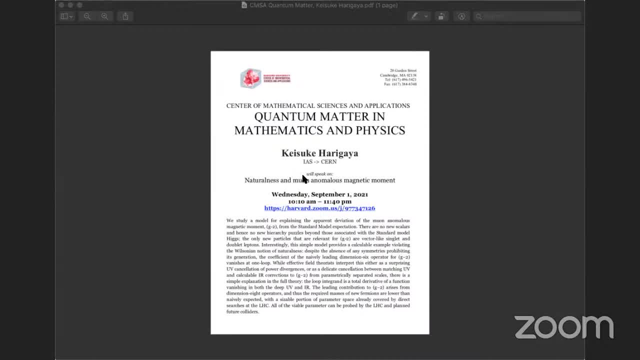 and when you're constructing these loops or effective operator, you can see that these indices between right and left are convoluted. So it's only spin zero there and it could not be a diaper moment- I mean magnetic moment at all- because it is convoluted indices. 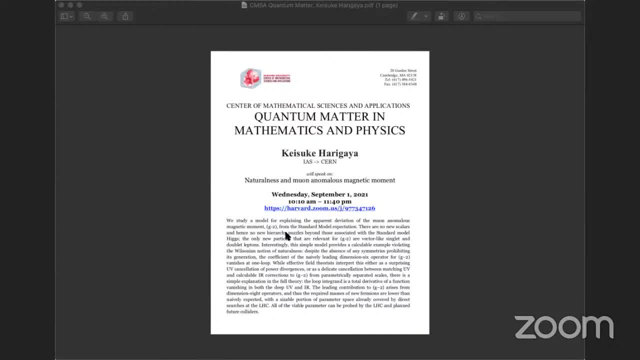 So it means that your integration bypasses Because it's already done and it is zero. So we still have the following operator. Let's see. Is this visible or should I turn on the? I agree, Are you talking about absence of? 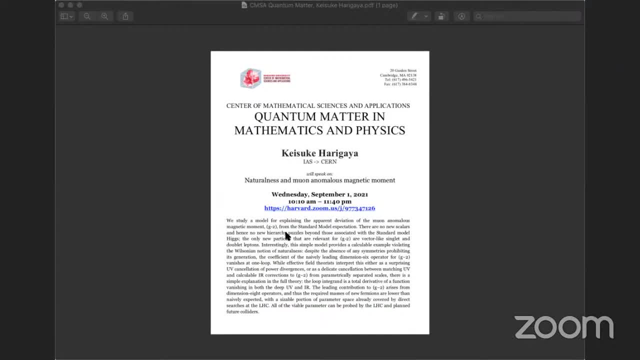 No, no, but look, you can write effective operator. This, for example: write a way and the effective operator would be containing a Higgs field: C time When you integrate. yeah, yeah, This one Right, but if we knew it should be convoluted with spinner indices, right. 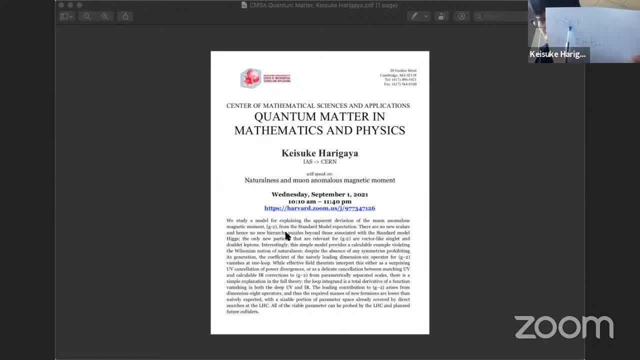 We have another operator here, So this also contributes to G minus two. Which one? This upper one, the one without the powering matrices? No, but you can rewrite the same way: Yeah, Yeah, Yeah, Yeah, Yeah Yeah. 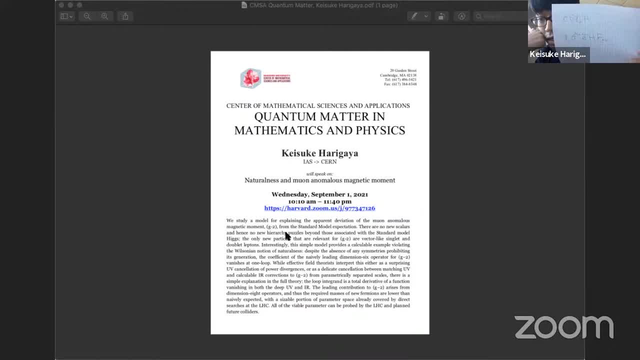 It's kinematical. I disagree. There is only one operator because they are dependent. So in this way it's not independent operator And when you're constructing you know your loop, or whatever. let's say that they're integrating over heavy quarks. 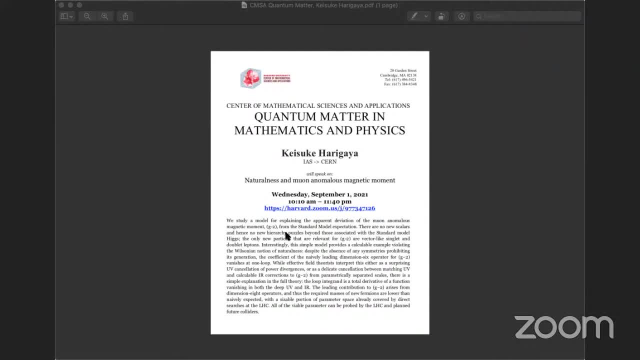 Okay, So what you will get? You will get a Higgs field C times right, But spinner indices of right and left would be convoluted. I agree, I agree, That's why we have this diagram. Yeah right. 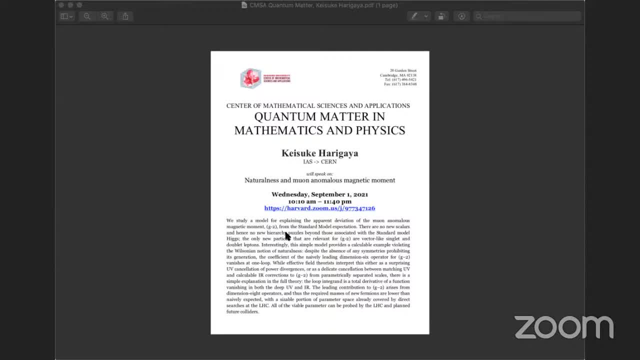 But then it doesn't contribute to the magnetic moment. No, no, this does contribute to magnetic moment. No, no, no, It's a, it is. look, if you have a psi alpha- in this sense, you know how to say- you have a convolution, the same as a mass storm. 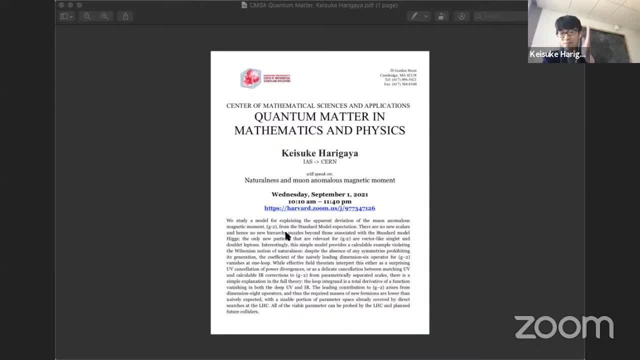 it is scalar. yeah, i, i, i agree, i completely agree. but my claim is that this operator contributes to gms2. i do not see it very clearly. okay, uh, because, uh, no, i mean, if you have a convolution of uh mu, bar mu, it is my storm, right? yeah, yeah, yeah, yeah and yeah, but do you agree that the 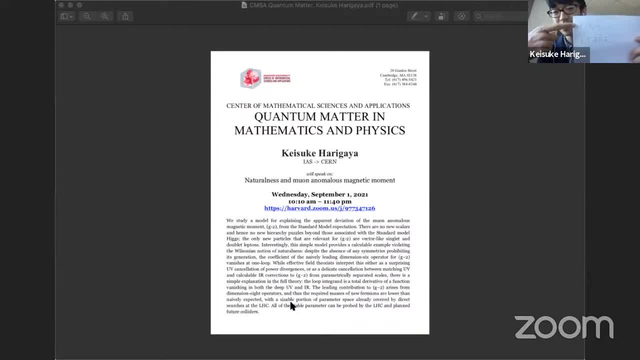 path of it that could be generated. yeah, can you read what is it? okay, just a moment. uh, yeah, so yeah, but look, uh, this one, uh uh, here it is. uh, it is a charge, right? so of course, gamma mu contains uh uh, contains. there is a tone which 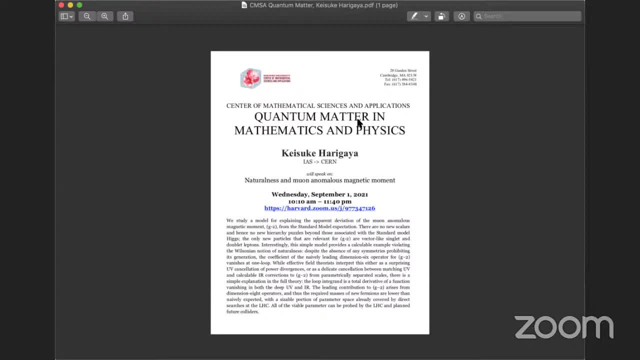 gamma mu, which is normal, uh, electric charge of muon, right, so, so, so. so, so, this normal magnetic moment, it's not g minus two, this contributed g minus two, no, but you can realize this as gamma mute at home. and f minute, oh, after. after you remove that, then using equation, then you obtain this. yeah, but, but, but, but, uh. 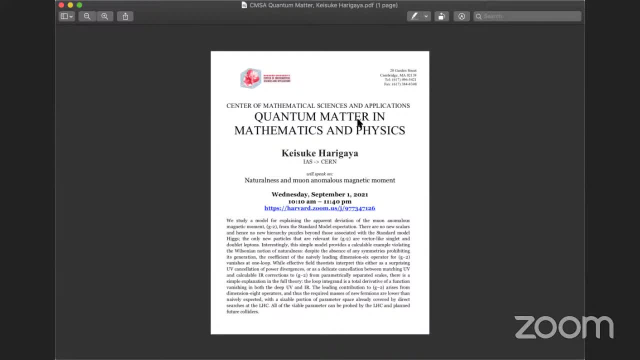 if you take uh, my impression is that if you, i do not see how you will get g. if you, if you integrate heavy quarks out what you will get, what operator, this operator, how you will get uh uh, how you have uh, this uh. caweian derivative. 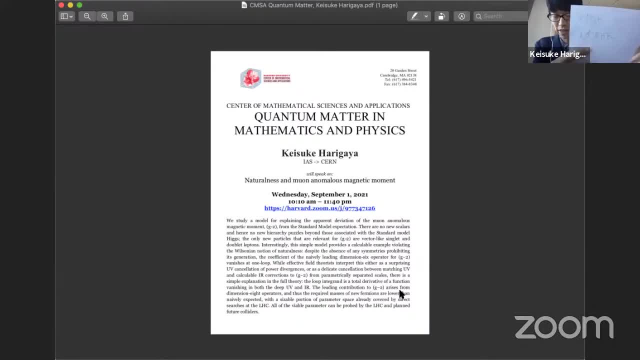 It's just a derivative, It's just a moment of dependence. No, no, But if I'm integrating heavy quarks, the main term would be the one where there is no derivative, Because you're just substituting heavy quark. I mean relating one over mass right. 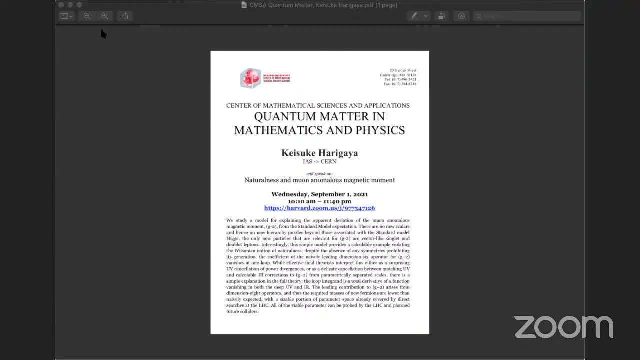 You're expanding it in mass Mm-hmm, It's before taking photon Mm-hmm, Before photon Mm-hmm, Okay, And then whatever you do with the loop, it doesn't help you. But no, no, no, no, no. If you have a diagram, so then if you expand with respect to the moment of the…. 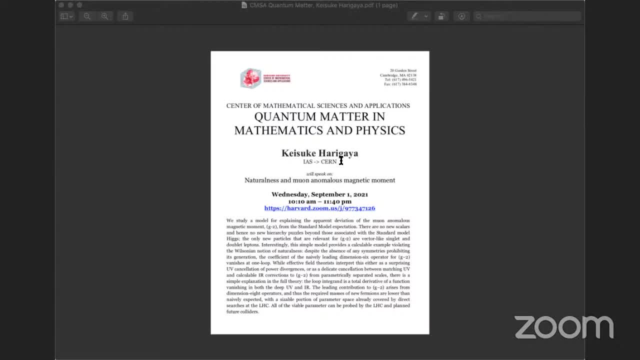 No, no, no. Okay. First of all, consider three diagrams, three level diagrams- Mm-hmm- And integrate out heavy quark Mm-hmm. Okay, Then, what is the leading term? The leading term one over mass of heavy quark, right? 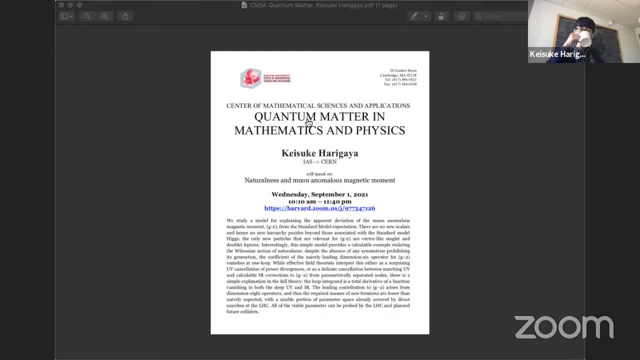 Mm-hmm. Multiply by something Mm-hmm And you can integrate both your L quarks and S quark. integrate both So you'll get one over mass and one over ML and then something there, And it's what I am describing. it is this sum and it is three level. It's not a loop. 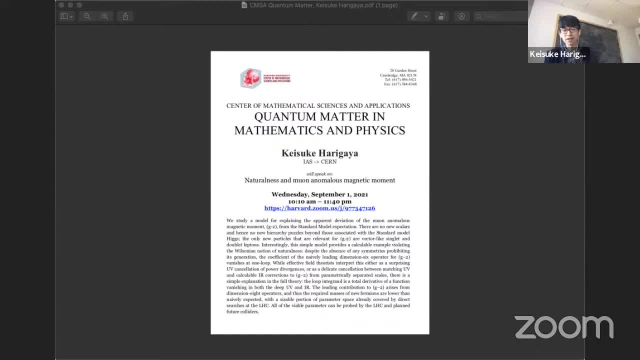 Yeah, yeah, At three level, Okay, And at this three level you have only spin zero, Mm-hmm. A spin zero between this muonic, no, I mean wave function. So then, whatever you do with the loop would not help you to get magnetic moment. 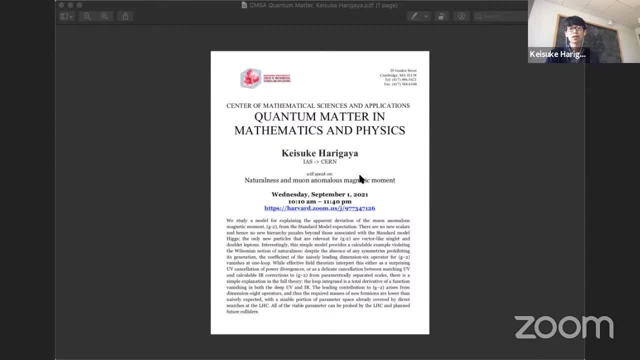 So… No, no, no, no. So then you must look at the next over that. you did that, But next it would be higher. And then I've already mentioned, I am talking about the… No, no, if you use higher dimensional operator, then we should take care of that. 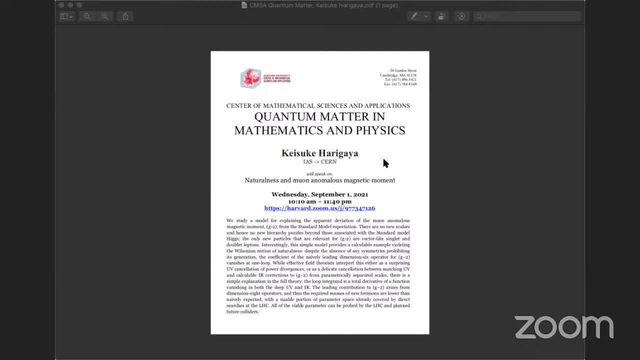 Okay, Take care of quadratic divergence, Okay, But this one loop vanishing is related to what I am trying to say, Mm-hmm, Because in this way you can consider not loop but this integration of heavy quark, And then, of course, once you get this spin zero, then loop would not help you. 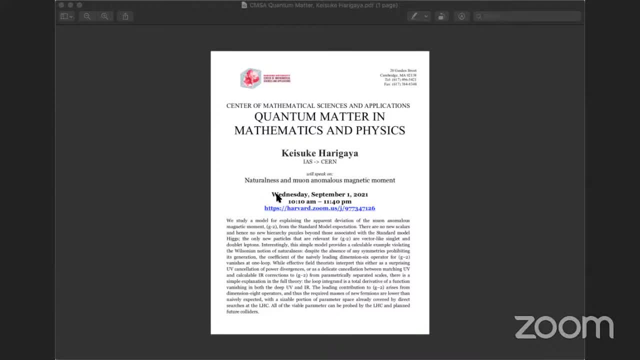 Mm-hmm, Mm-hmm, Mm-hmm. when we go further, when you expand further and consider derivatives, then it could be what you showed in higher orders. I'm not arguing about this. You use a higher dimension, higher derivative operator and now you have to deal with the 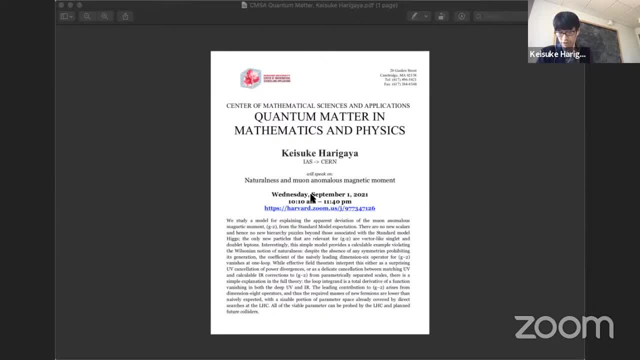 quadratic divergence if we want to use the low energy theory. So you can simply look at the leading lower dimensional operator to argue that d minus u should vanish. Yeah, yeah, yeah, Because you were discussing that. it's surprising. kind of no symmetry relation. 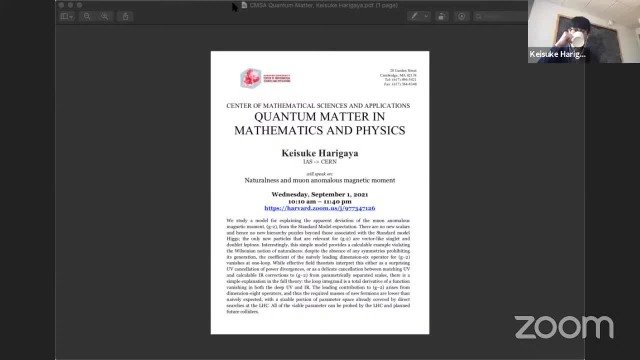 I'm trying to say just, it's not surprising. Okay, it's not about your higher dimensions, it's about: Okay, I'm sorry that I started to. Yeah, maybe they can start to share the story. Okay, okay, I'm sorry. 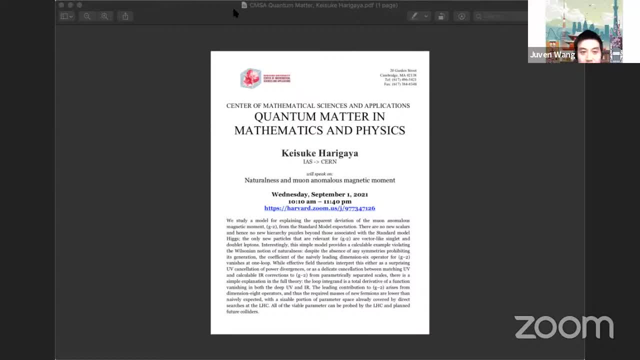 Yeah, yeah, And then you should ask during the talk. You can feel free to ask during the talk And you can share the screen. Okay, okay, yeah, Yes, Can I share the screen? Not yet. Okay, okay, okay, Can I see it? 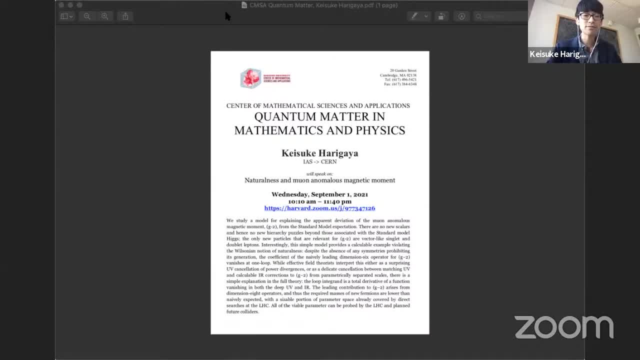 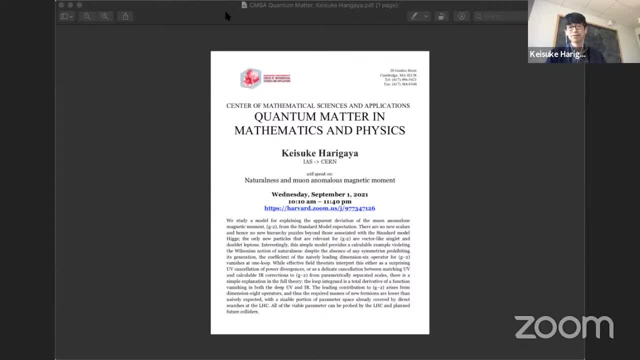 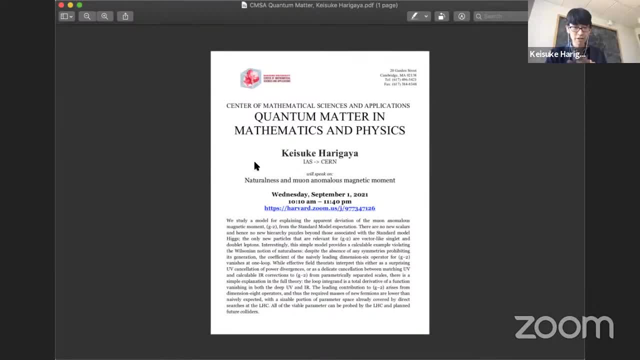 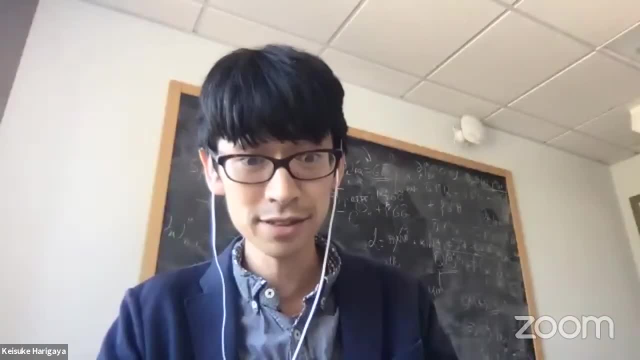 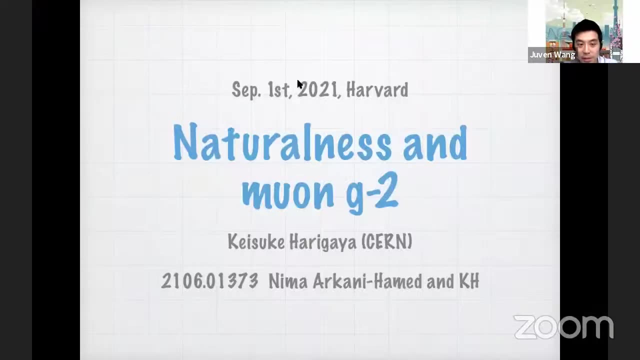 Thank you realizers. Thank youでき cross topic. Thank you, road 끝alos libre streaming Android. Okay, can you see my screen? Yes, now Can I start. By the way, are you leaving at some time? 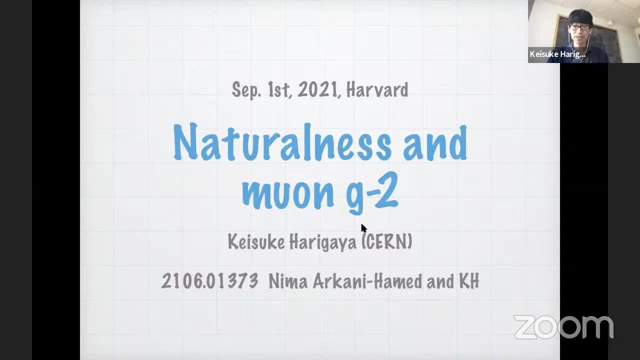 Yeah, I have to pick up my kids before 6pm. That's why I asked you to start a bit earlier. Okay, okay, Yeah, so maybe we can quickly start then. Welcome everyone. Welcome to Hover Quantum Math and Math and Physics seminar series. 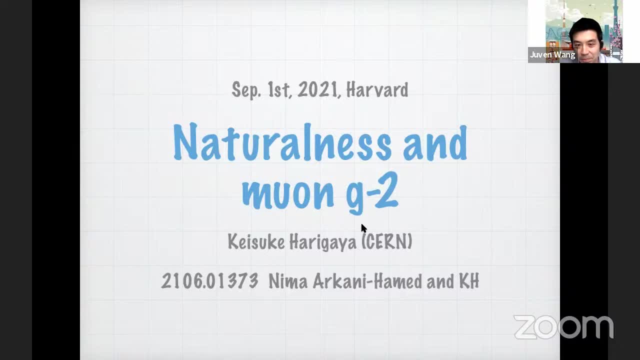 We are very honored to have a topic on again mu 1 to minus 2.. And it's a theoretical topic that Keisuke Aigaya will be presenting. Keisuke was a colleague at IAS a few years back. 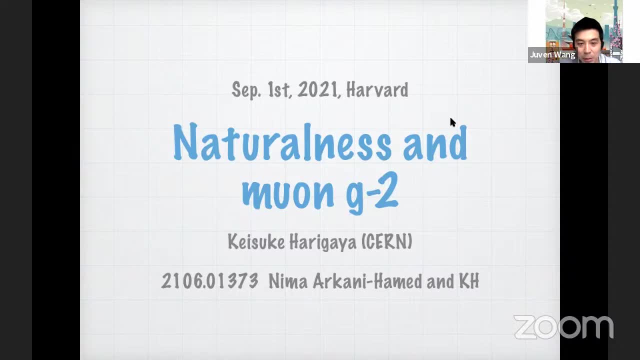 But currently he just moved to CERN And he will speak about naturalness and mu 1 to minus 2, worked on with Nima. Before I begin, I especially encourage the audience. presumably there will be more of this later. 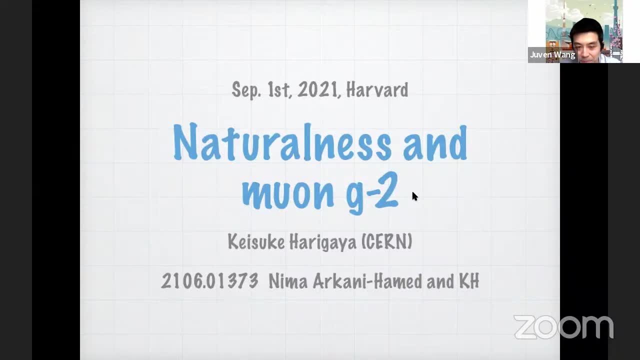 Please feel free to interrupt and ask questions And also welcome. Thank you, Okay, Yokozo, Please take over. Hello, I'm Keisuke Aigaya, So thank you for the invitation to this seminar series. So today I would like to talk about some naturalness and mu. 1 to minus 2,. 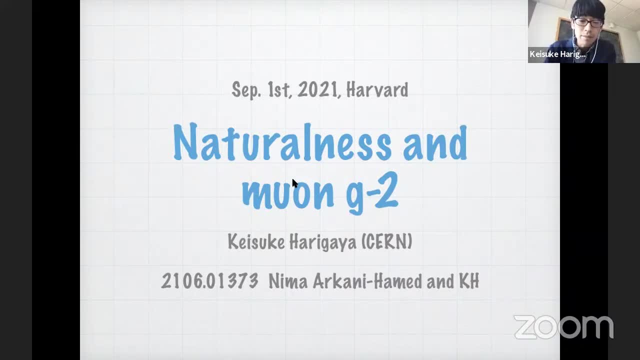 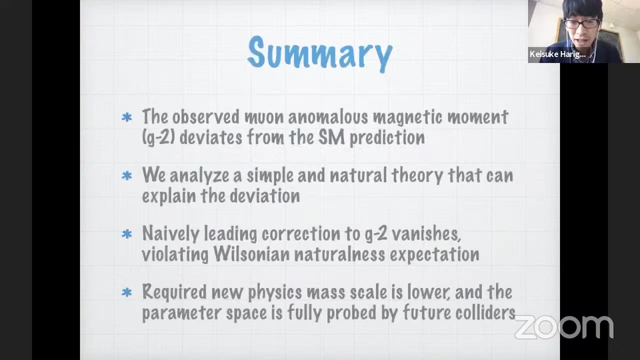 the anomalous magnetic moment, based on the paper with Nima Arkani-Hamed. So here's a very brief summary of my presentation. So one, the observed mu anomalous magnetic moment, which is called G minus 2, which I will introduce. 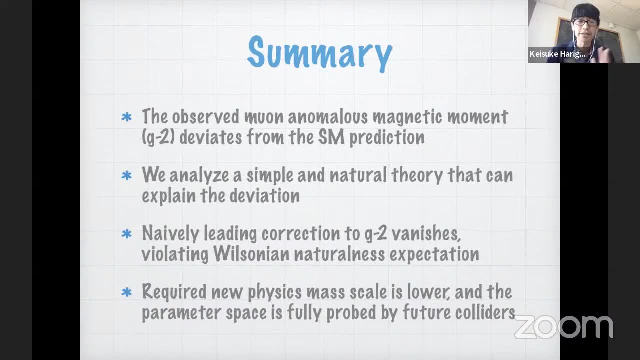 deviates from the standard model prediction. So two: we analyze a simple natural theory that can explain the deviation. Three, however, the naively reading correction to the G minus 2, the anomalous magnetic moment vanishes, so violating the naturalness expectations. 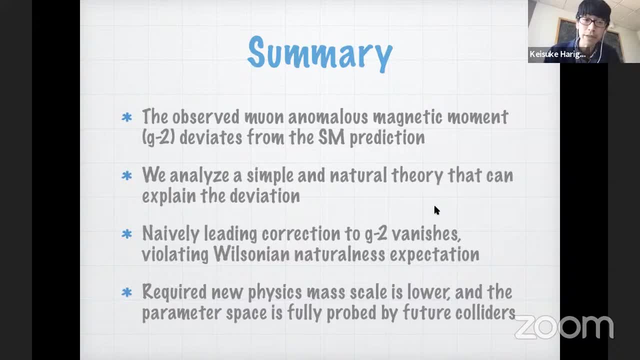 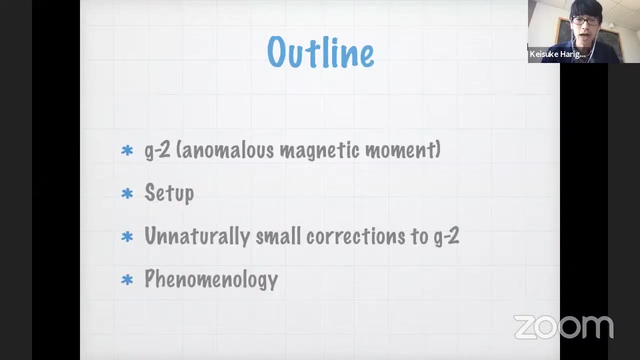 And four. finally, I will explain some phenomenological implications of this vanishing G minus at the reading order. So here is the outline of my presentation. So first I will introduce what the G minus 2 anomalous magnetic moment is And then explain the setup of our model. 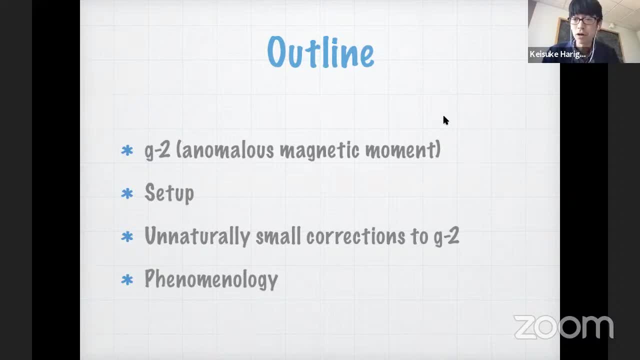 So then I will show the computation of the correction to the G minus 2 in that setup and show that the correction is unnaturally smaller than the naive expectation, And finally I will explain the phenomenological implications. So let's start from the G minus 2.. 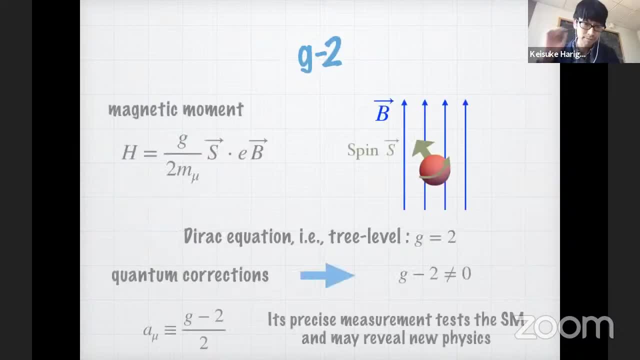 So G minus 2.. So the generically charged particle or the particle that has spin can interact with the magnetic field of the form. spin times the magnetic field. So its coefficient is often parameterized as G, So using the Dirac equation. so in another word: 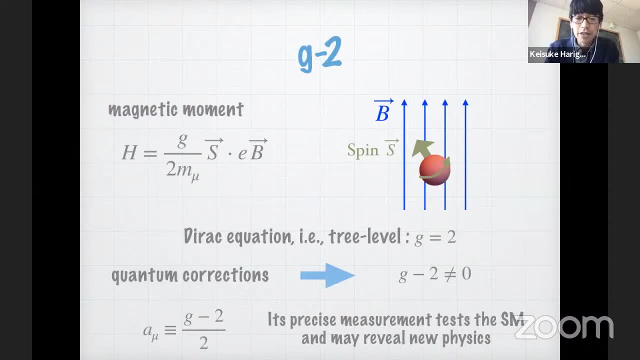 at the tree level for the charged particle, we can show that this factor G equals 2.. However, after including quantum correction, such as a QED or electroweak quantum correction, this G deviates from 2.. So we call this G minus 2, or anomalous magnetic moment. 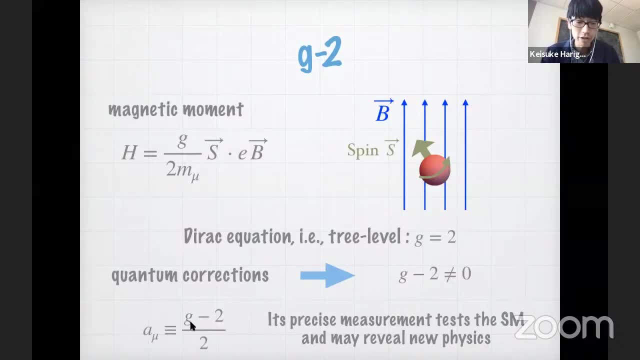 So we also use the notation G minus 2 divided by 2, which is denoted as a mu. So this G minus 2, or anomalous magnetic moment, is sensitive to the quantum correction. So its precise measurement can test the standard model or possibly reveals a new physics, if that exists at a low enough energy scale. 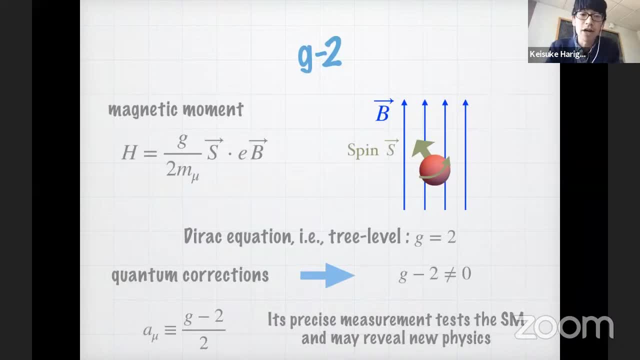 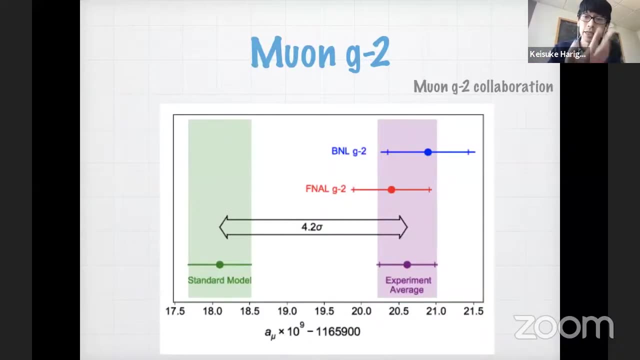 And, of course, people have computed this precisely and people have measured this precisely, So, as was explained by a seminar in this seminar series about two weeks ago, so there seems to be some tension between the standard model predictions and the measured value of the anomalous magnetic moment. 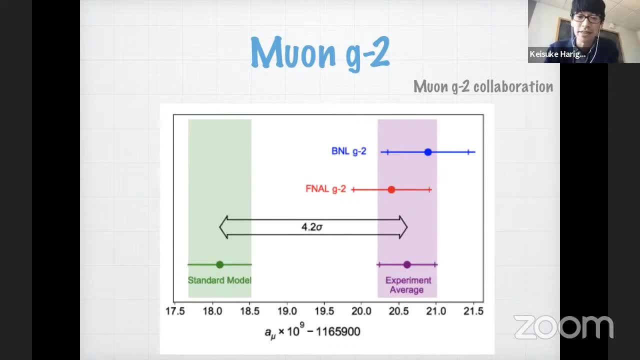 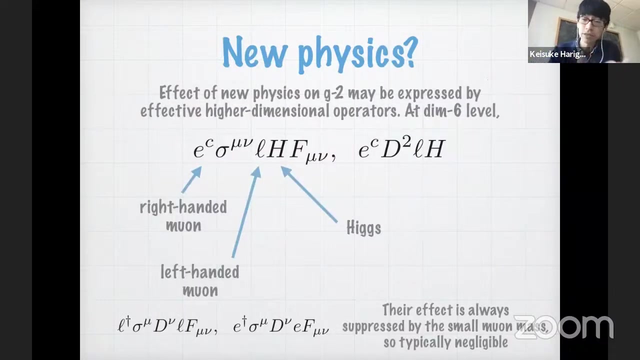 which is formally about four sigma. It just means that this is four times larger than the error. So this may be due to some deficit in the standard model computation or possibly some experiment. But today let's pass the possibility that this deviation is actually explained. 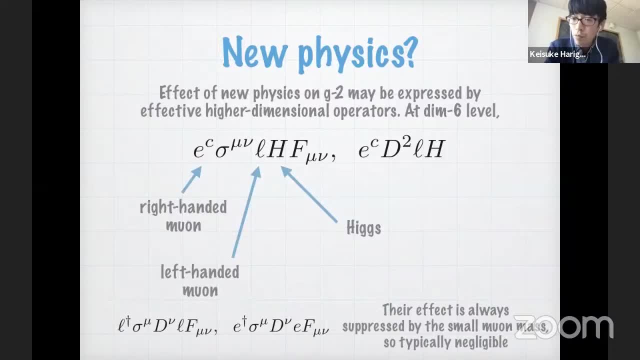 by some new physics beyond the standard model. So that's what we are going to do today. So first let's do some analysis based on this. So this is based on the effective operator, So the effect of new physics at low energy. 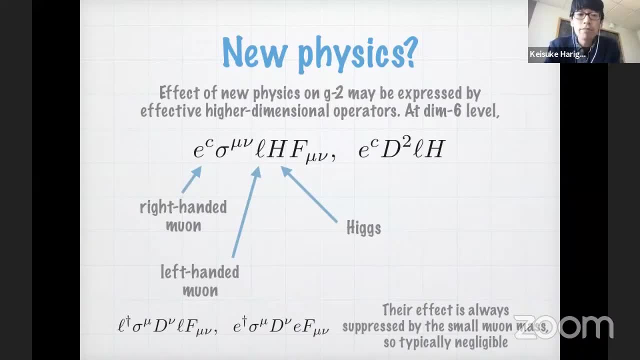 namely the energy scale at which the G minus is measured, may be expressed by effective higher-dimension operators. At the dimension 6 level we have the following two leading operators: So here can you see the cursor, I guess so. So here. 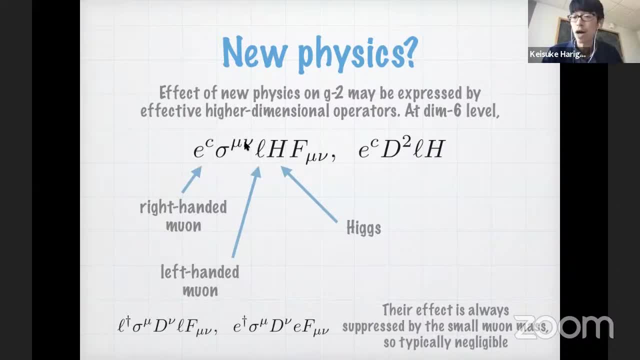 E is a right-handed mirror, A sigma is just powering matrices And L is a left-handed mirror That couples to the weak gauge border in the standard model, But here H is a Higgs. So we need this Higgs because right-handed mirror is singlet of SU2,. 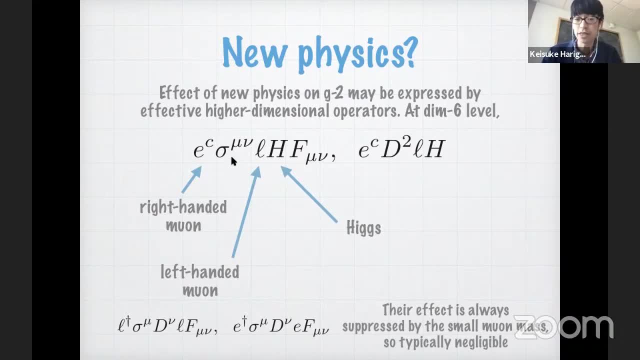 but left-handed, is a doublet of SU2.. So to compensate that we need Higgs And of course, to have a G minus we need a photon. This is one operator, So another operator. another possibility is the one we saw. 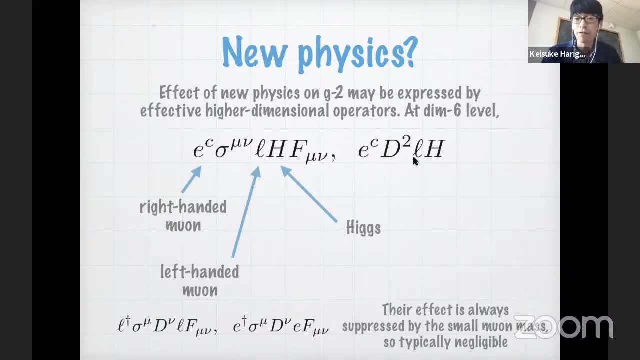 the powering matrix, but just derivative, covariant, derivative on the fermions. So these two are the leading operators. So we have another dimension 6 operator, shown at the bottom of the slide. but their effects are always suppressed by the small mu mass. 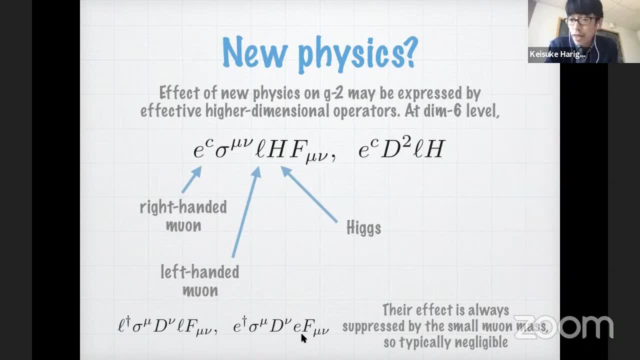 in comparison with the new physics scale. So these are typically negligible. So we will focus on these two operators shown at the top of that that slide. I'm sorry to interrupt, but d-square acts on what Sorry? d-square, d-square. 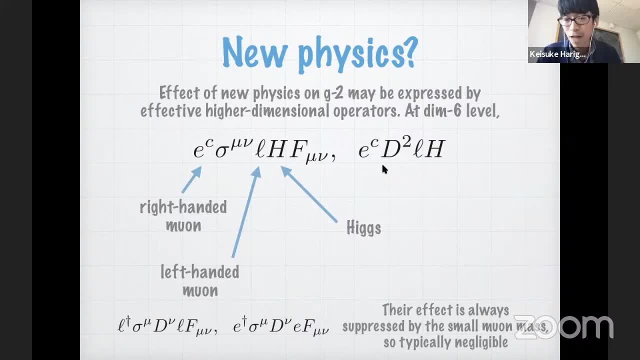 Yes, Could you say it? X on what d-square? X on the electron? Yeah, If you act by d-square on L, then it's equation of portion, right, It is d-slash-square. Yes, It's trivially balanced. 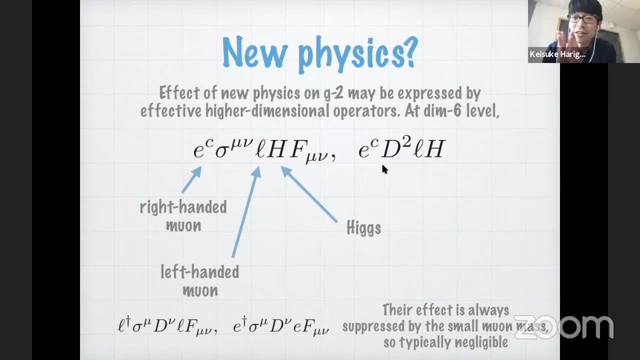 Oh, d-square d does not have a gamma matrix, It's really derivative. So what? So here d is not d-slash, but really d. Okay, But d-square acting on what? On L or on H, So it can act on both. 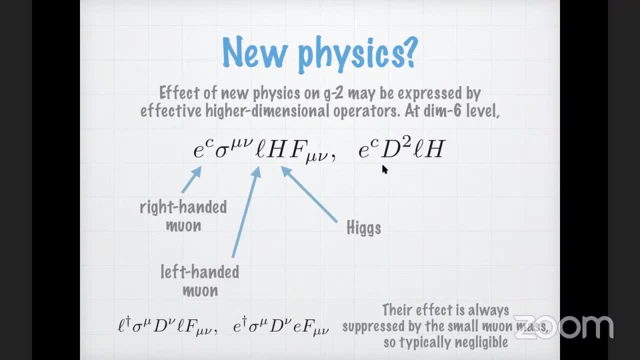 Okay, There's a better possibility about that. In low energy physics, acting on H is not a subject, True, true, Yeah, If you can just ignore Higgs When d-square act on L, you can use equation of motion to express this as a first operator. 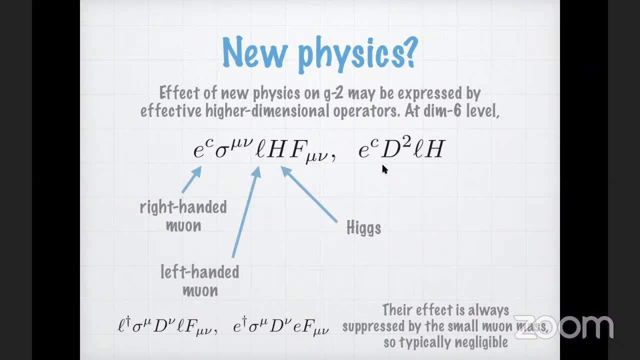 Mm-hmm, mm-hmm. So there is no two operators at low energy. So still, so that we have Okay, okay, yeah, In normal d-square without slash, it is still. you can rewrite it as d-slash. 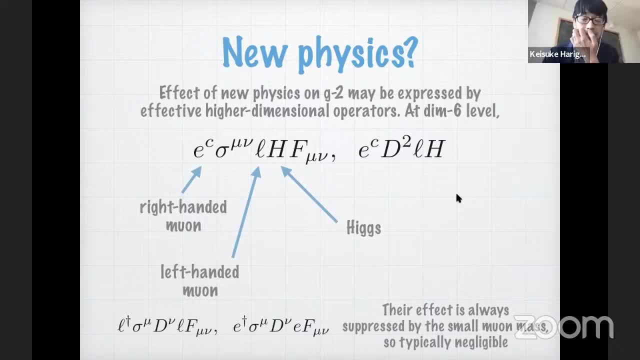 square minus mu, whatever Mm-hmm, And then you will see that it is the same operator as the first one and H should be substituted by mass of particle H, it is mass of mu After using equation of motion. 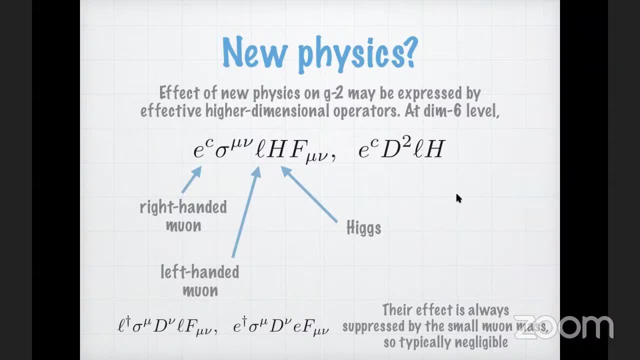 yeah, I think I agree. Okay, So then, statement about two operators is not relevant for low energy physics- Mm-hmm. But still, this d-square, after using equation of motion, contains the first operator, So it still affects the g-minus two. 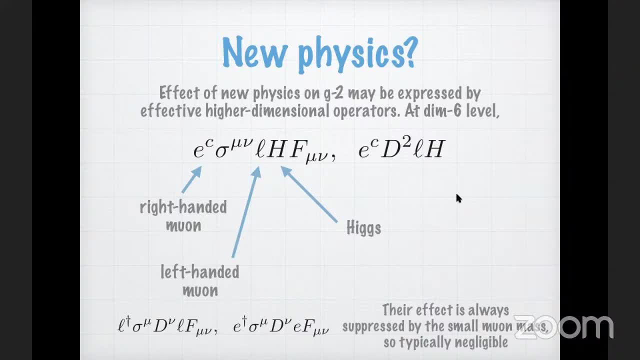 But it is the same operator, because equation of motion is supposed to be. Using equation of motion. yeah, yeah, yeah, All right, but At amplitude level. yeah, Okay, Yeah, yeah. So in this way I would say that: 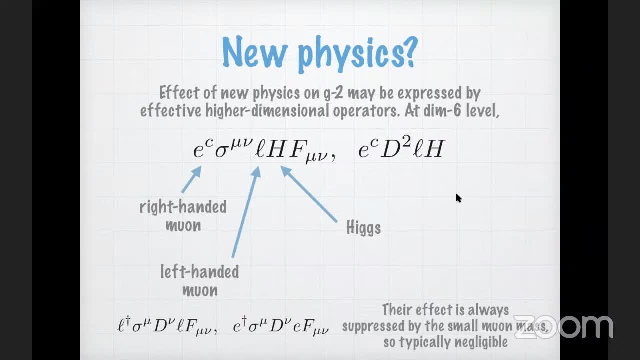 if you had to count operators, then I would say that it is dimension five, not dimension six. Mm, let's see, Because H is just a number. so I agree, But here I use this electric No, no, of course you. 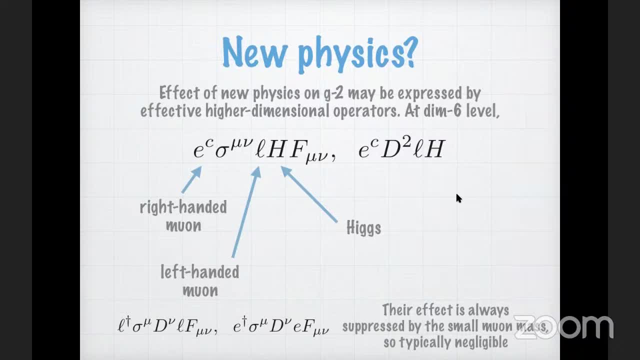 Yeah, yeah, yeah, You can say that it is six because it's multiplied by mass. Yeah, yeah, yeah. But I mean yeah, yeah, Typically I will consider. I will consider the theory where, when you think, scale is about electric scale. 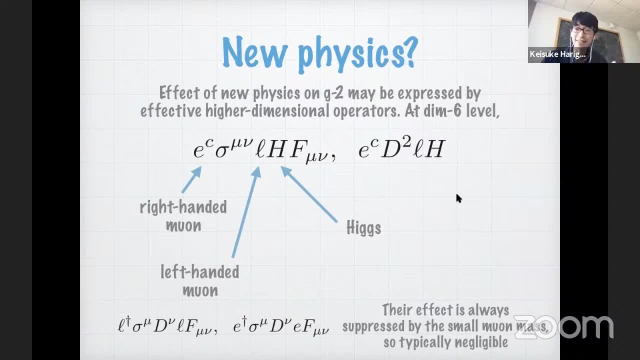 so this electric symmetric notation would be convenient. yeah, No, but still in the experimental way. you are substituting H by I agree, yeah, yeah, yeah, I totally agree with you. Okay, let's proceed. yeah. 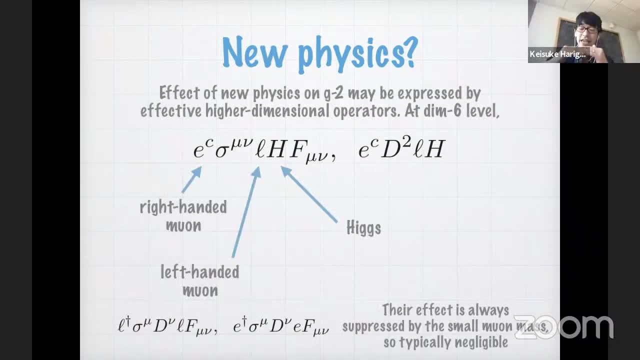 Okay, I agree that below the electric scale we can just put six at the wave and we can just use dimensional five operator. Yeah, I agree, yeah, Yeah, But later I will come to use a dimensional analysis to put the new physics scale. 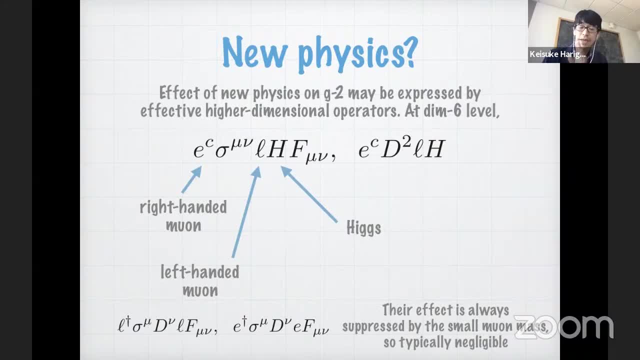 in the downstairs. So for that purpose, it is better to keep Higgs, as you know. Yeah, Okay, thank you, yeah Okay. can I ask a question also? Mm-hmm, mm-hmm, So what? 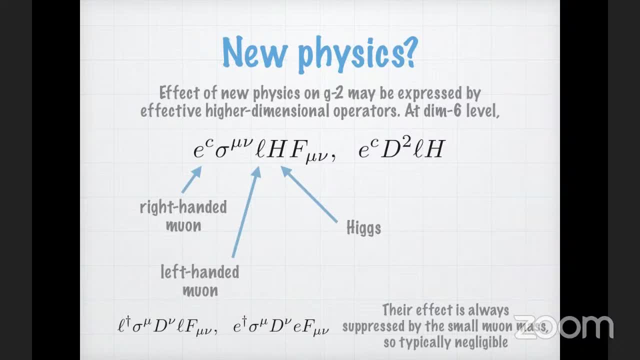 Mm-hmm, You said sigma is polymatrix, but you want like four by four. It looks like this first operator is spinful, no, So here. so So I use a two-component notation. So sigma is actually two by two matrix. 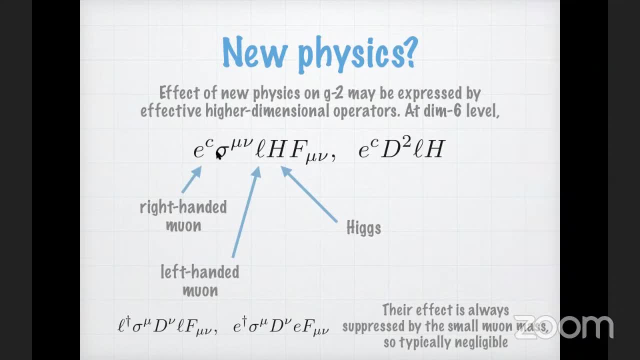 So does that answer your question or did I miss something? No, I don't understand what these indices are then. No, I don't understand how you get a singlet here, a spacetime singlet. So we have mu nu. 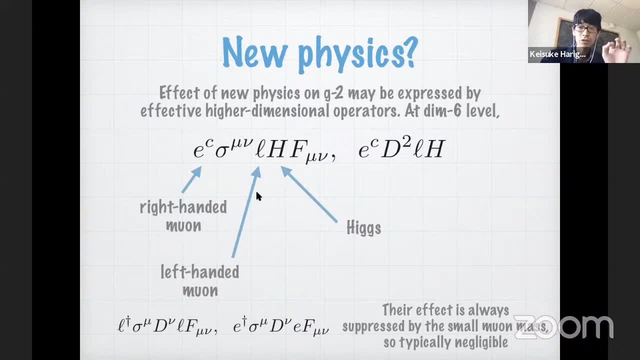 So this is the. This has a two-vector index. This is the just multiplication of the two polymatrix And we have F here. So that's how we obtain Lorentz scalar. Maybe the sigma mu nu is the. I forgot officially. 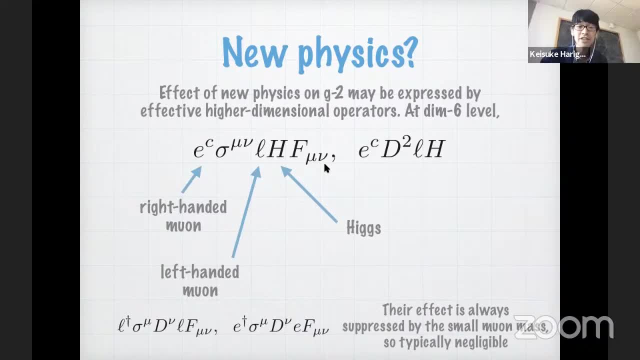 Doesn't mu nu range over four indices? I don't understand. Zero, one, two, three, Yeah, yeah, yeah, Actually, it's like here: the polymatrix plus the sigma zero, The unit matrix, Yeah, which I use to form: 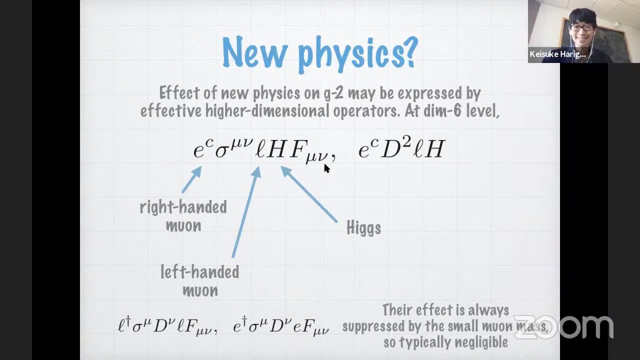 Lorentz, invariant quantities. Can you remind us just your notation of sigma mu nu written in terms of the sigma mu, which mu is zero, one, two, three. So sigma zero equal just unit matrix, And sigma one, two, three. 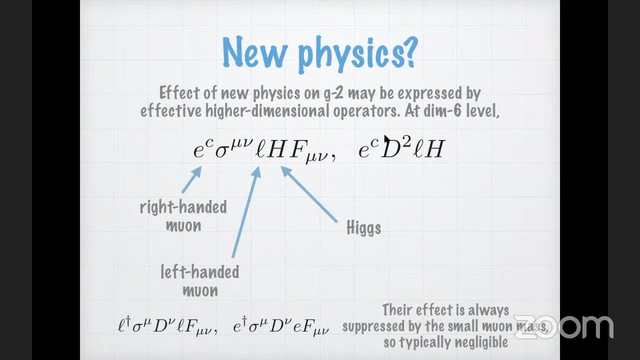 is proportional to sigma one, two, three, the usual power matrix. Yeah, that's no problem. But my question was: how do you write sigma up mu nu in terms of sigma mu? So it's just sigma bar mu. It's sigma bar mu. 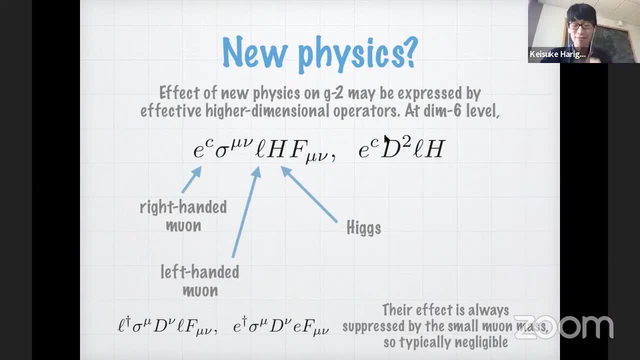 sigma mu minus sigma mu, sigma bar mu And the sigma bar is defined so that the sigma zero is Yes, no problem, But I don't understand, Like you shouldn't be. There isn't a spacetime two-form That you can use here. 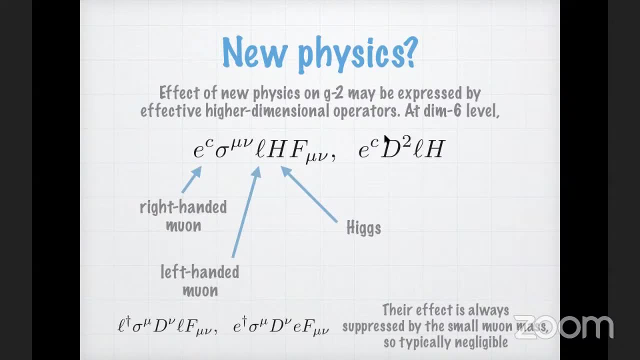 This doesn't look Lorentz invariant to me. No, no, But look the simple way to represent what Kishore is saying: use this spinor indices, Then you have E, c, alpha, L, beta. I mean spinor indices. 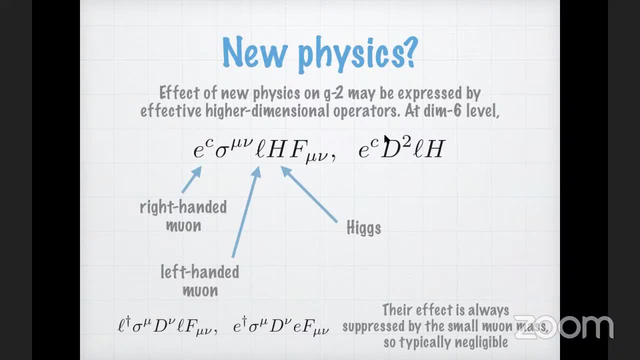 which one? two, okay, And F alpha beta Where? alpha beta? it is this supersymmetric form of, you know this, F mu nu Instead of F mu nu. the index is zero to three you can use. Oh, I see. 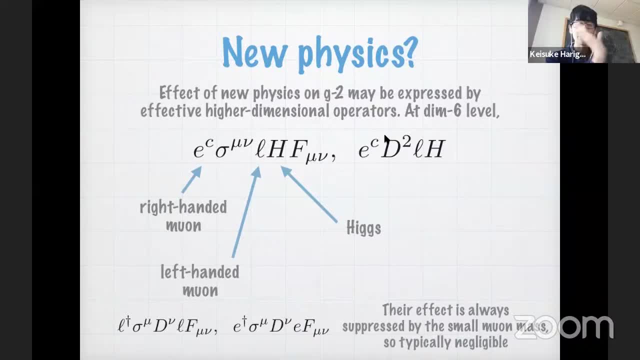 I see what you're saying. Okay, You prefer spinor, not this. And it is very simple form, because you can immediately see that you have, I am sorry, symmetric F alpha beta multiplied by you know this- E c alpha L beta. 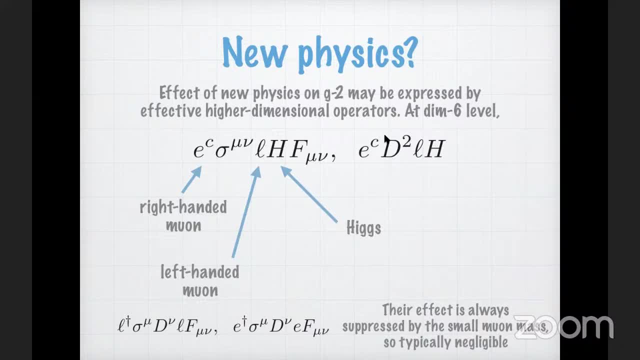 I agree, You can make it from the spinors. Okay, Yeah, But it is the same. But it is the same as you. as was said, It's just different notation. Mm-hmm, Yeah, Thank you, Thank you. 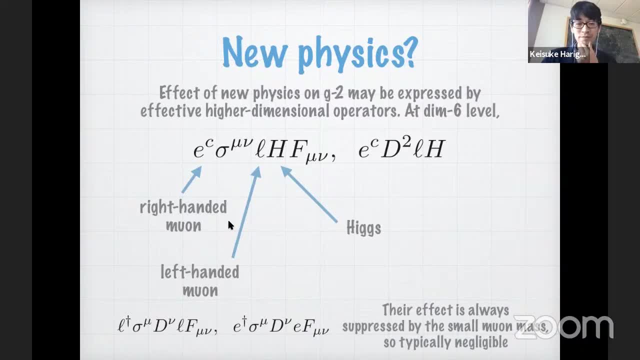 Yeah, So let's see Where are we now. Oh, okay, So let me proceed. How can I proceed? So then we tried to explain the deviation of G minus two from new physics. What we do is construct a theory such that a quantum correction 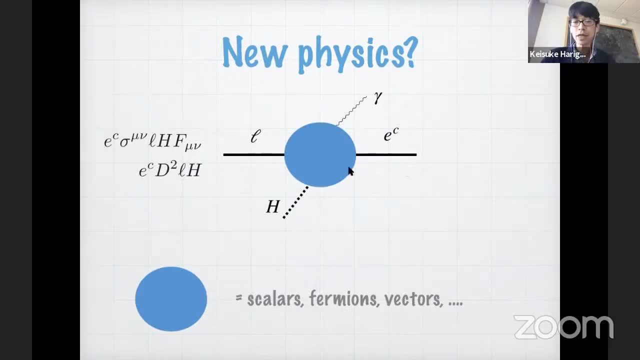 to the new particles or new interaction generate, generate this the quantum correction that can be expressed by this diagram. So left-handed particle, muon, right-handed muon, photon and Higgs. So the anything could be inside this blob. 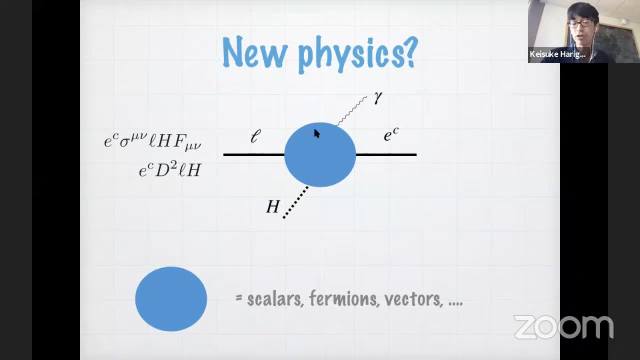 It could be scalars, it could be fermions or it could be vectors. So this, the computational model, is of course module-dependent, but we can. we can extract the naive expectation for the mass scale of the new Higgs. 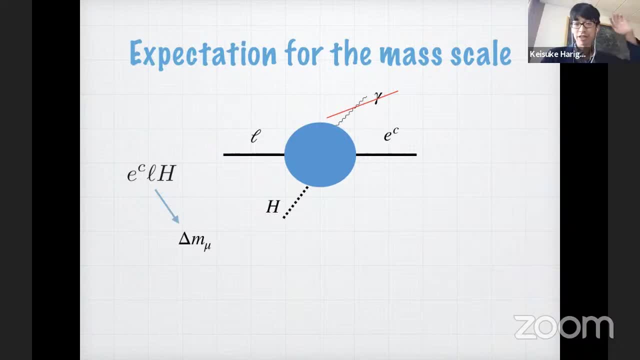 in the following way. So from this diagram let's just remove photon. So then this is nothing but the quantum correction to the Yukon coupling between Higgs and muons. So that gives quantum correction to the muon mass. So this is dimension four. 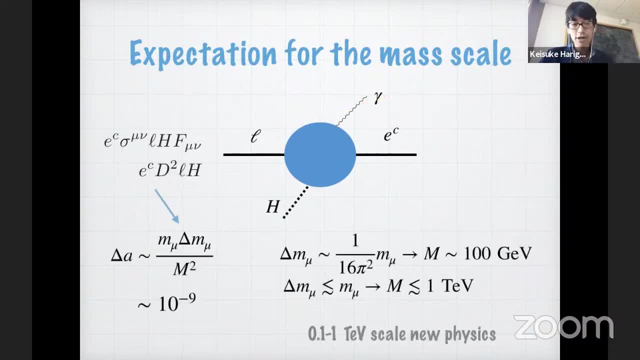 correction to dimension four operators. So now putting back the photons, a photon, we obtain the dimension six operator. So then from the dimensional analysis. so we can just put the new Higgs mass scale in the downstairs and compensate it by the muon mass. 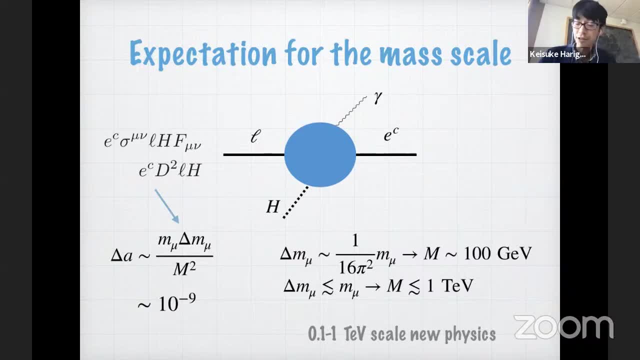 to obtain a naive expression, that naive relation between the correction to anomalous magnetic moment and the correction to the muon mass. So if let's require that, this is a slide that observe deviation 10 to minus nine. so if this correction to the muon mass 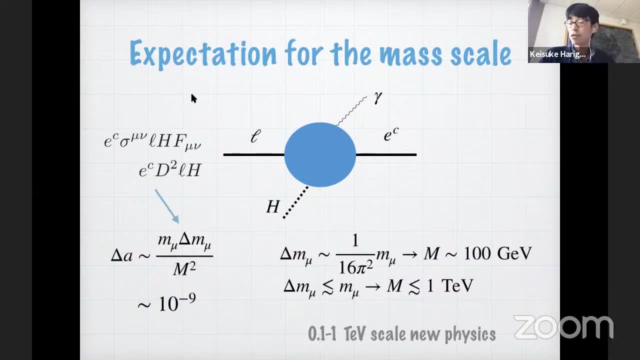 is one loop suppress in comparison with the muon mass, which is the case when this correction itself is that proportional to the muon-Yukon coupling. So then, to explain deviation, we need a new Higgs, mass scale around a hundred Gb. 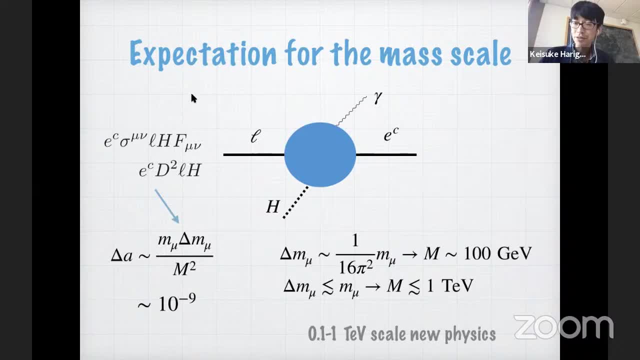 But on the other hand, if the quantum correction to the muon mass is as large as the observed muon mass itself, so this new Higgs mass scale could be as large as the one to 50 Gb scale. So from this, 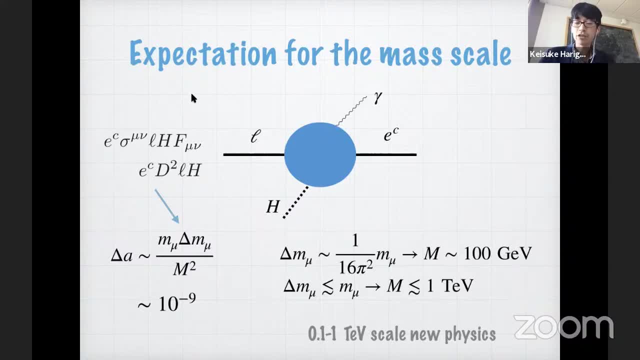 you can see that we will expect a new Higgs scale around the electric scale to the 10 times the electric scale. You're saying those two corrections have to be of the same. You're saying those two corrections have to be of the same order. 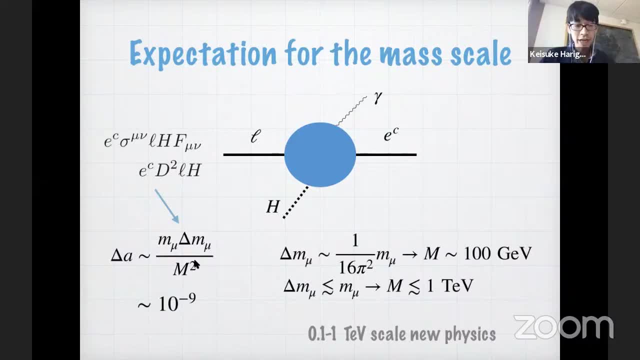 for the prefectures. I mean this naive relation after pre-factor. yeah, But look, it is just dimensional analysis, because look what scale you have. You have mu and this new mass, large capital. M right, The statement is that the answer is proportional. 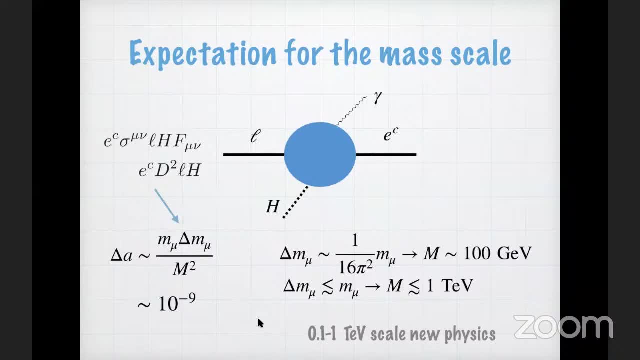 to square of the ratio. Okay, And the proportionality to mu square follows from chirality right, essentially So. in this sense, then, it's just about numerical coefficient, But the appearance of There is no any other low energy scale besides the mu. 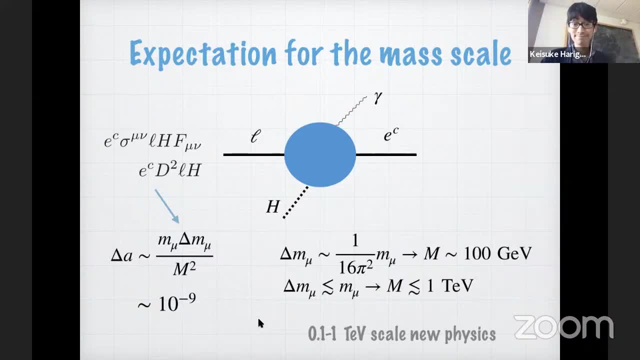 if we are talking about this, Mm-hmm, Mm-hmm. Okay, Thank you. Well, this numerical factor could be six or one six. So, yeah, no more than my expectation, but we should actually compute diagram, Yeah. 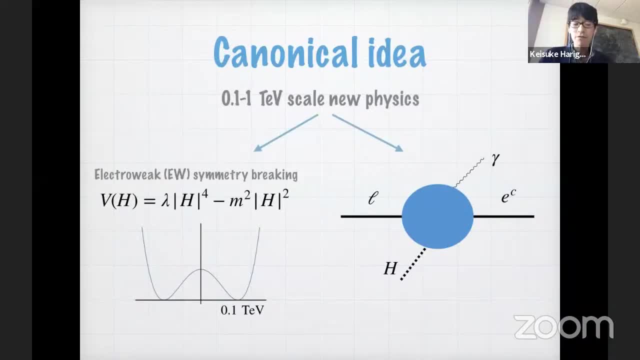 Okay, So then, based on this, approximately the origin of the electrocuite scale, and I new physics to explain the g minus, give us a G mass to the people- has considered the following, what we we could call canonical idea. So this new physics scale around the 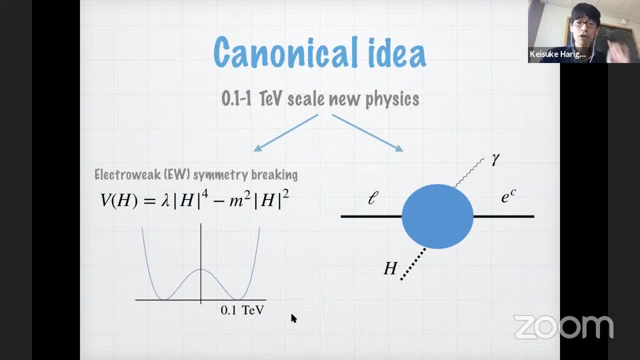 electrocute scale or bit above that electric scale explains both the origin of the electric symmetry breaking by the stamina fix and the deviation of the G minus two famous example is supersymmetry, where the mass of the Higgs is basically given by the 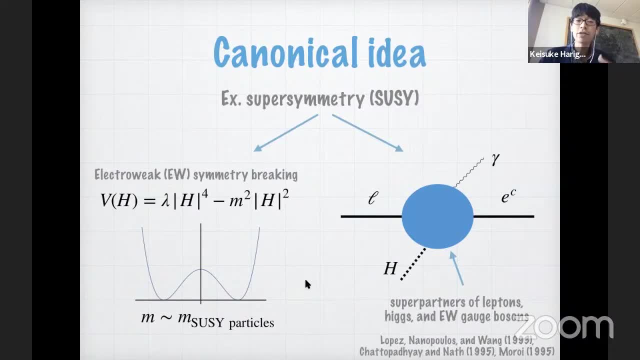 masses of super particles. So in other words, Susie breaking, induced electric symmetry breaking And the masses of the superpartners of wepton, Higgs and electric gauge boson give a quantum correction to the muon-magnetic moment as was first considered by these authors. 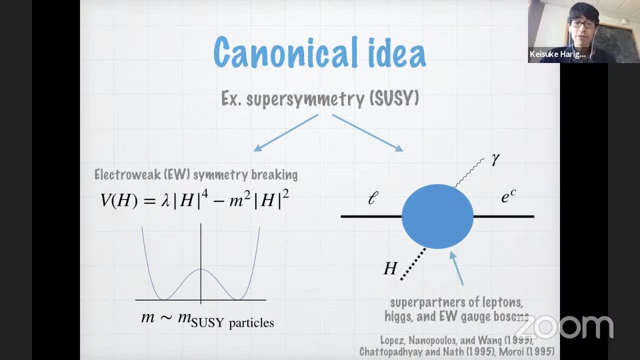 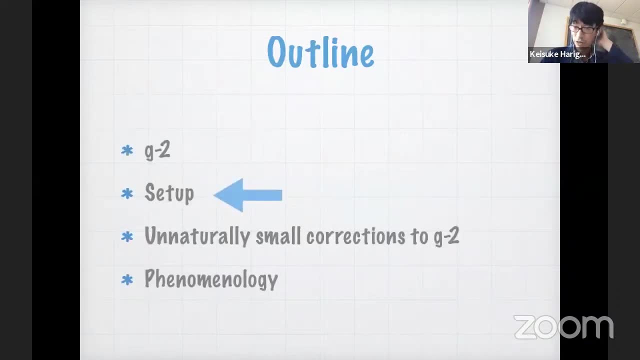 So this was a canonical idea which dominated for maybe the last 20 years or so. So that is the end of the overview of the G-minus and the past box. So let me move on to what we want to do: the setup. 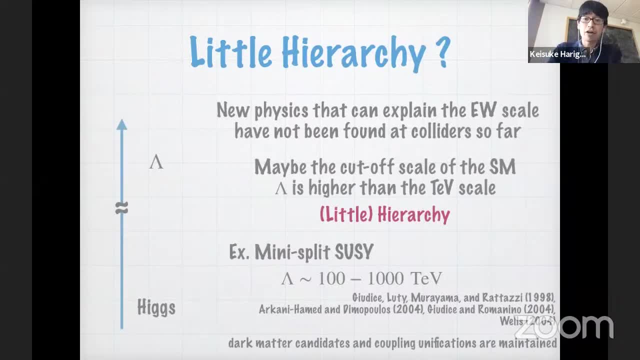 So let me move on to what we want to do: the setup. So let me move on to what we want to do. the setup. So the canonical idea was, as I explained, connecting this muon G-minus 2 with the electroweak symmetry breaking. 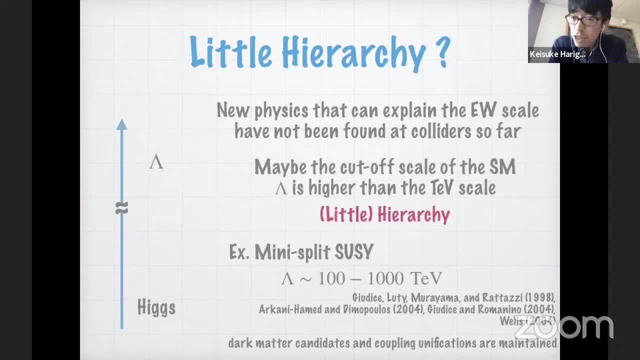 But today we'd like to consider the different possibility where we have so-called little hierarchy between the electric scale and the new physics. Yeah, so explaining the electric symmetry scale by new physics is a great idea, But unfortunately so-called So far no new physics that could explain that electric scale, the magnitude of the. 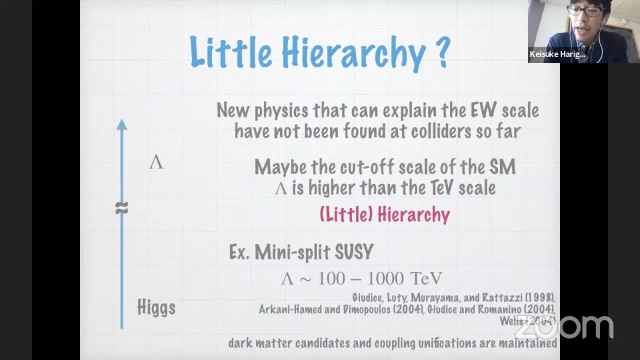 electric scale have not yet been found at colliders so far. So, based on the situation, we should seriously consider a possibility that the cutoff scale of the star model, which we can call lambda, is higher than the TV scale. It could be much higher, but it could be just a bit higher than TV scales. 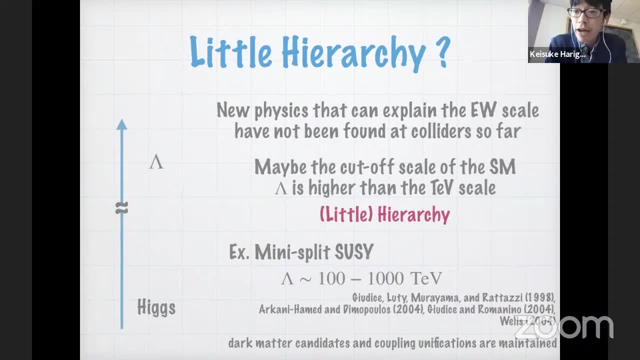 So we are. We often consider this situation the little hierarchy between the electric scale and the new physics scales. So one example, known example- is so-called mini-split supersymmetry, where the cutoff scale, the masses of superpartners, are around 100 to 1,000 TV. 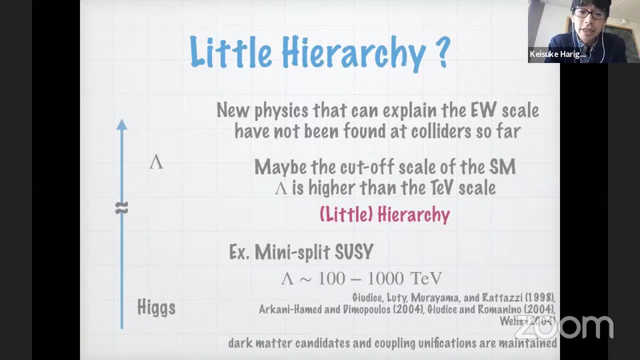 So in this scenario the electric scale is highly fine-tuned, but still it has some good motivation, like having dark mass, Yeah. So it could be 0.2,, 0.6, or something like that. that could be high enough to take a. 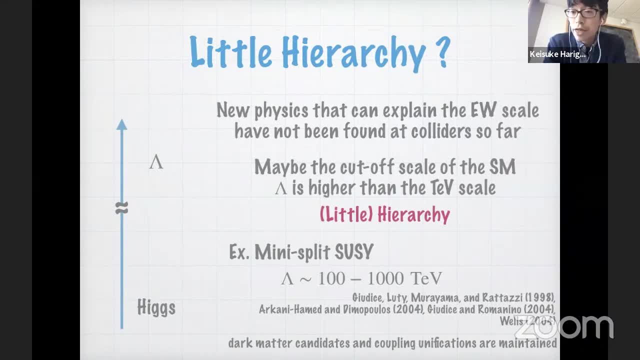 lot of mass. So this can be found at the mu and W. So it says that it's actually a little bit different. So one example. so on the right-hand side you can see the mass of the metal and the other on the left side. 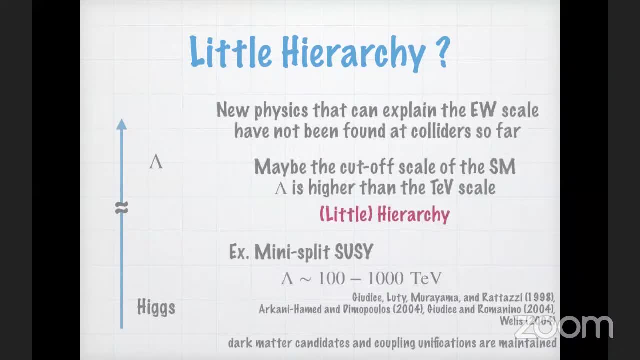 So the mass of the metal that I just showed you. but it's not possible to have a strong mass. You can actually take mass of the metal directly from the material, and that's what. Maybe it's just a little bit of weight, So I will try to explain it a little bit slower for you, but that's the way I can do it. 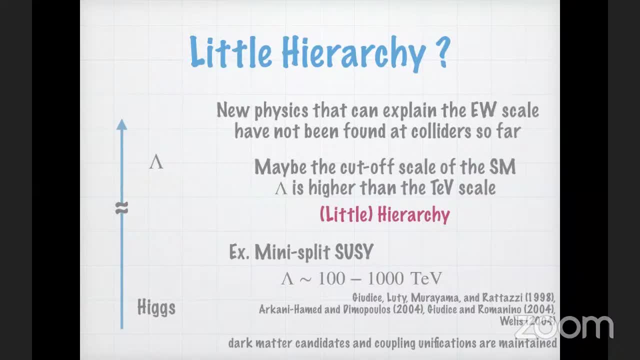 OK, OK. So let's see The wave shirker. you can see it here. Oh, so it could be at the top particles of mass around that scale. What amounts? what does it mean to explain the scale, Explain the scale. it's like the obtaining that scale. 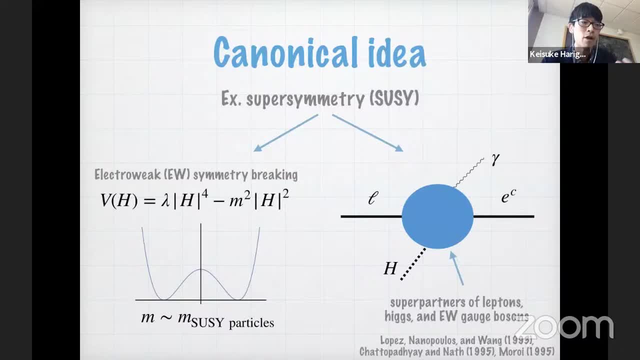 from other dynamics, like obtaining the Rommelson mass or Pion mass from the QCD scale, I see. so you will always shunt it to some other scale that you already have. Yeah, yeah, Okay. So the idea is that one wants to have that scale, naturally. 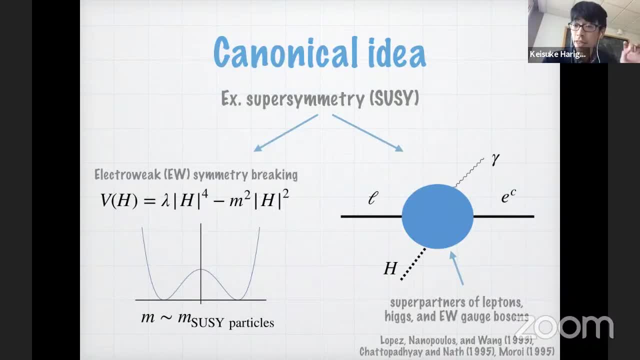 So, for example, we usually do not complain that QCD scale is much, much smaller than the Planck scale. That's just given by the so-called dimensional transmutation. So when we say we obtained some scale from some dynamics, That's a very basic idea. 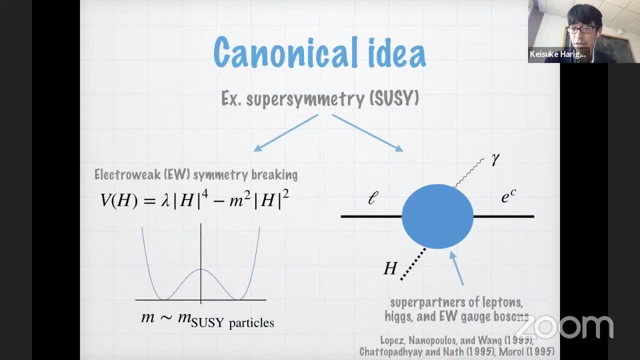 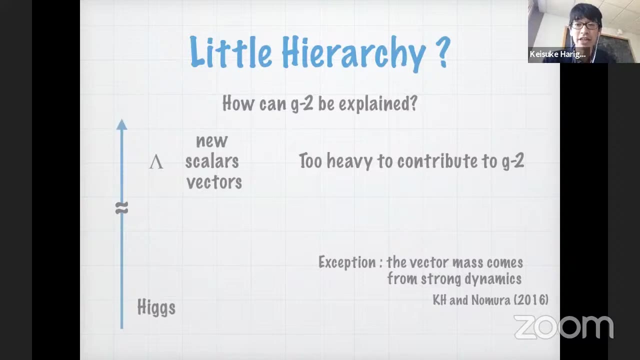 We want to explain the electric symmetry from some other dynamics so that we can easily explain why the electric scale is smaller than, for example, gravitational energy scale. I see, thank you, Thank you, yeah, So let's see. So then, if this is a, if the hierarchy is the case, 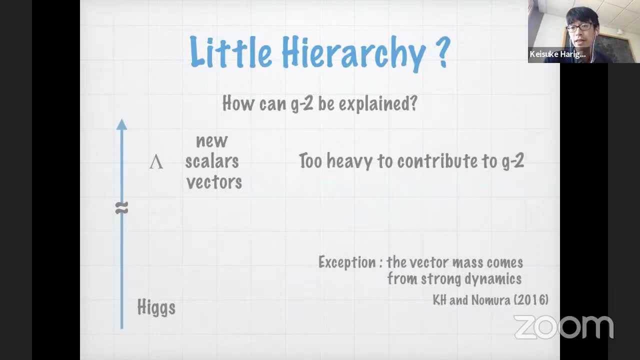 if the scale, a cutoff scale, is behind the Higgs, much, much larger than the electric scale. So how should we explain that G minus two? So we would explain, we would expect that new scalars would also have- would have a mass scale as large as a cutoff scale. 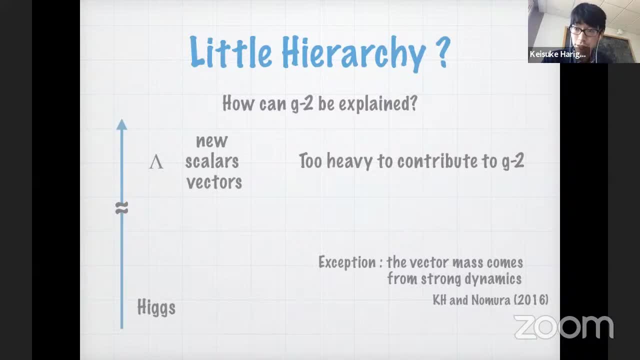 So they are too heavy to contribute to the mu G minus two, And we could also consider a vector. but to have a vector, so since we haven't formed them, we must give a mass to them. So we need some Higgs that give mass to vectors. 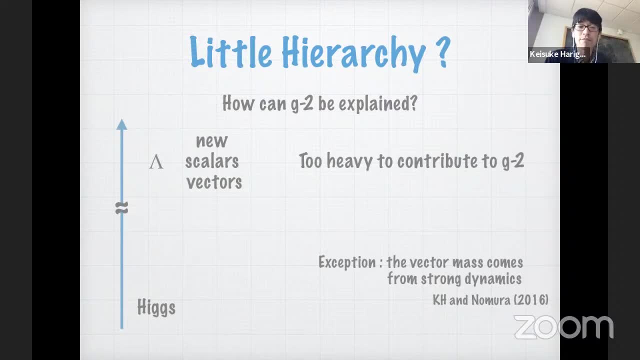 So because that extra Higgs which would be, you know, would be also heavy, we expect new vectors, if it exists, will also be heavy. So it is unlikely that new scalars and vector will explain that this deviation of G minus two. 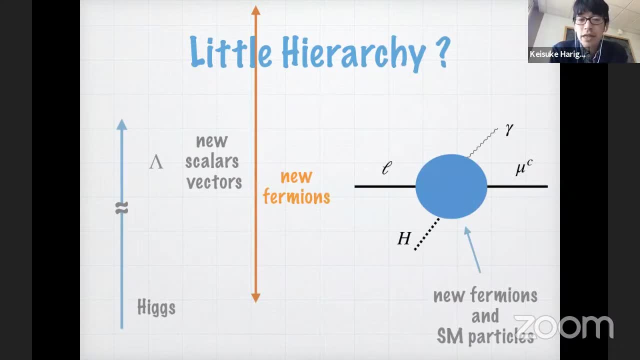 So we can, we will consider a possibility that new fermions explain the deviation of the G minus two. This is because new fermion, the masses of new fermions, are rotated by the, by the chiral symmetry, So there must do not have to be as large as a cutoff scale. 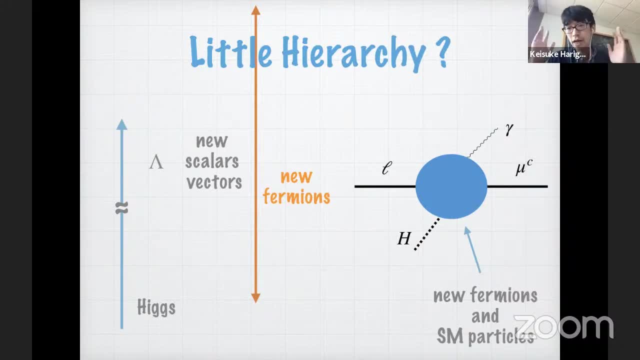 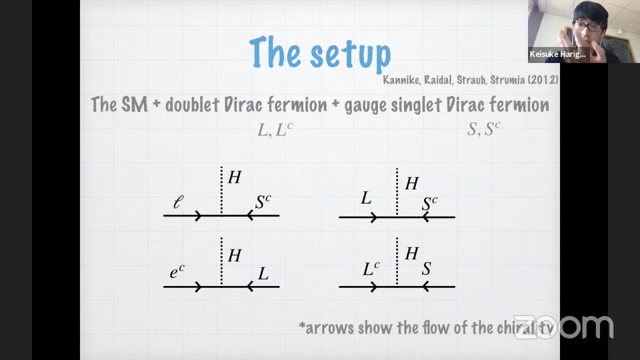 of that theory. So we restrict that the possibility to the case where this blob includes only new fermions and standard model particles, And such a possibility has been already considered in the literature. So for example, people consider that standard model plus SU, left-double-right Dirac fermions. 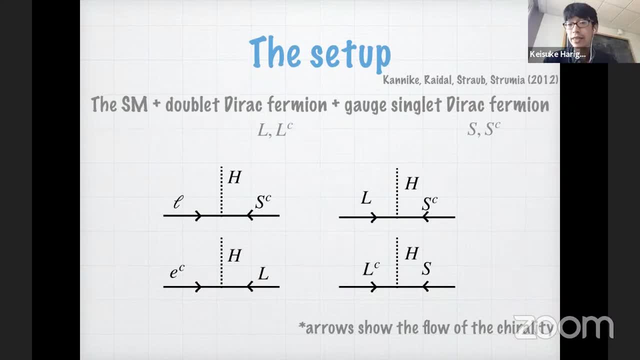 plus SU left-double-right Dirac fermions plus gauge-singlet Dirac fermions, And these also consider this possibility And the generic interaction between those new particles and the standard model particles are in addition to the gauge interaction. these four you cover interaction. 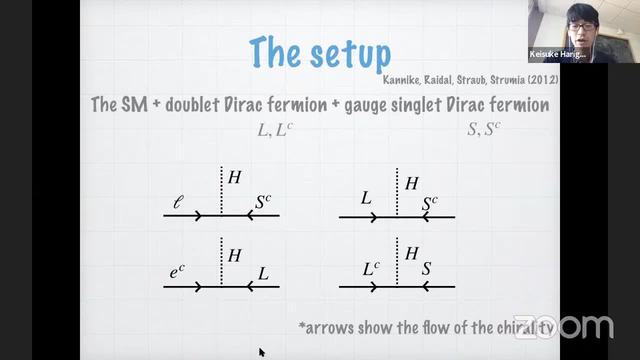 So here these arrows show the flow of the chirality. But but Higgs is the same Higgs, The standard model Higgs, or it's a new Higgs? These are all standard model Higgs. We never introduced new scalar because we haven't observed that it's a new particles. 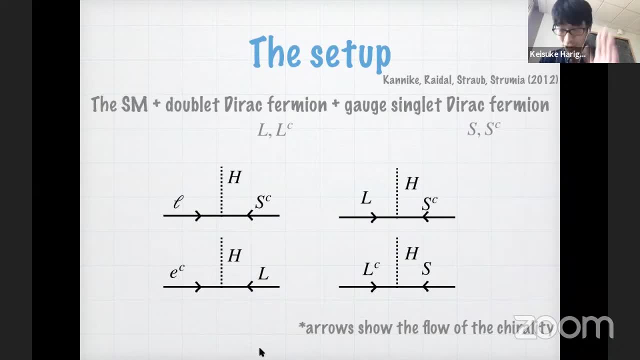 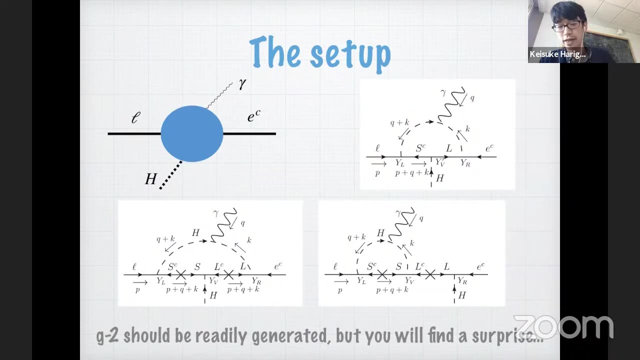 Yeah, New dynamics. yeah So, let's only use Higgs. yeah, So, so then with this interaction, and we can actually write down some Feynman diagram that seems to generate the muon G-minus two or or dimension six operators. 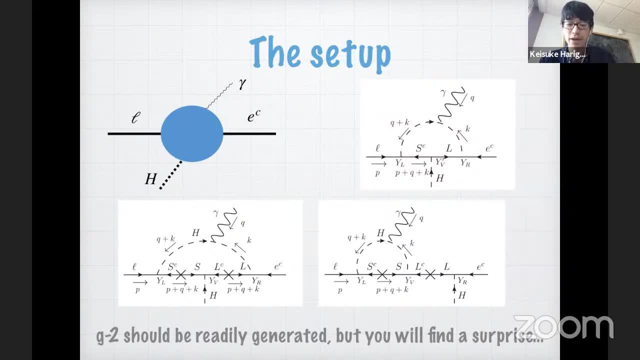 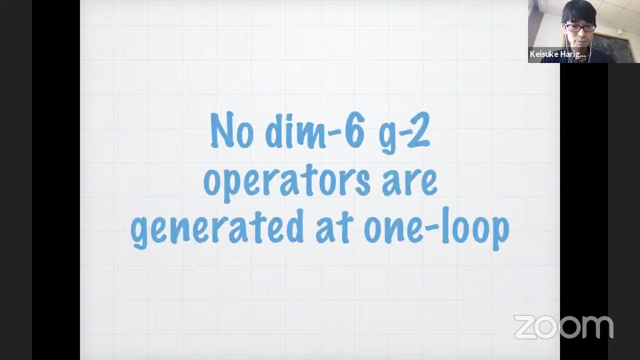 So if we compute these, we will then the non-zero G-minus two. but let's compute that, but we will find a little bit of surprise. Okay, let's compute the muon G-minus two in this setup. So it turns out that no dimension, six G-minus operators. 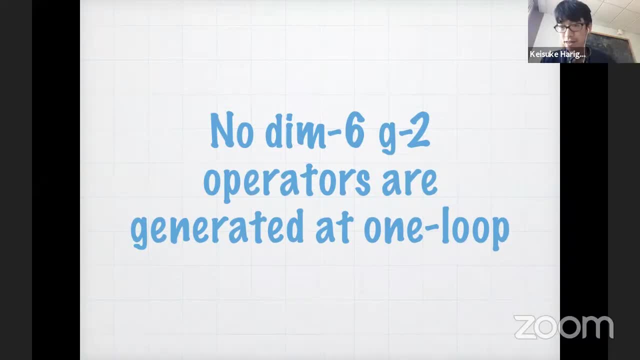 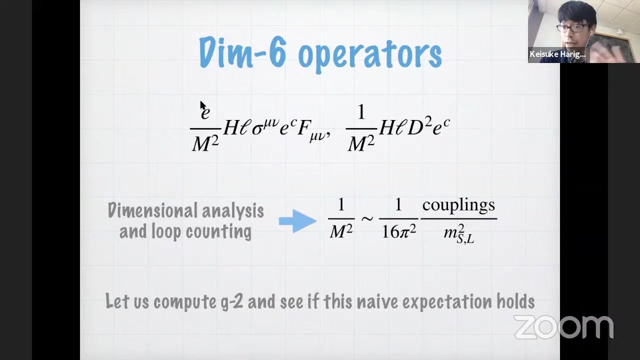 are generated at one loop level. So let me explain why that is the case in detail using a Feynman diagram. So, as we discussed this, muon G-minus two could be in the electric symmetric notation explained by this dimension. six operators So from the dimension analysis and the loop counting. 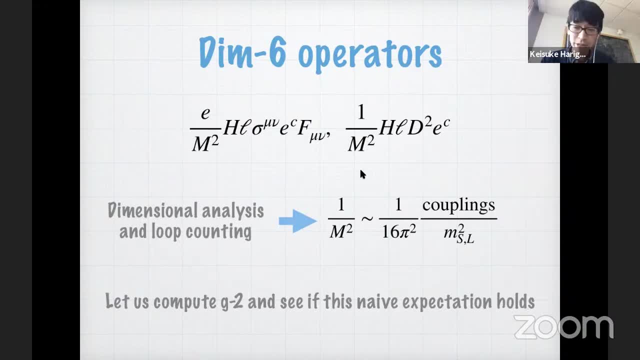 so here this one over m squared, m being the mass scale, would be as far as one over m squared. Okay, So if we compute the muon G-minus two over 16 pi squared, that loop factors and the correction of calc frames divided by the masses of new particles. 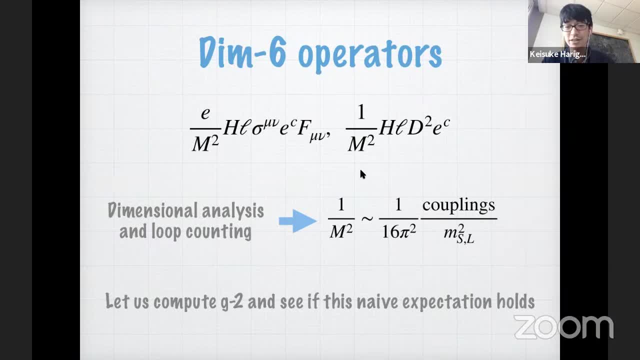 this would be our naive expectation, And if someone asked me to estimate the G-minus two in 10 seconds, this is the answer I would give. But let us compute the G-minus two and see if this naive expectation is really true or not. 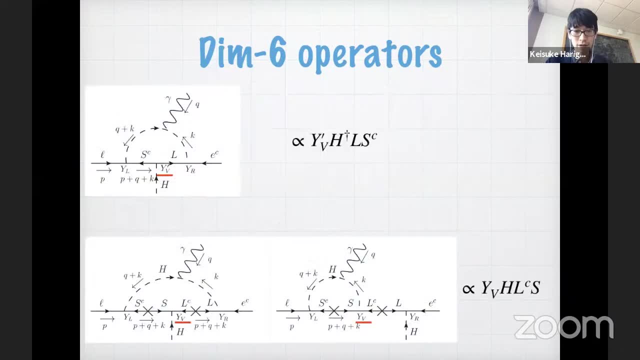 The answer is no, as you might expect. So the quantum correction can be divided into two classes of the diagrams. One is the proportion of this-Yukawa interaction, So another is proportion to this-Yukawa interaction, And the first one has only one diagram. 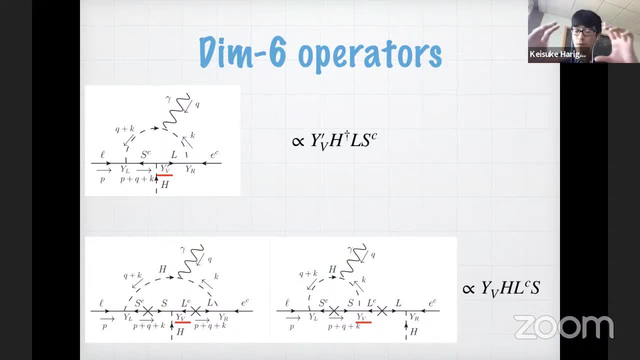 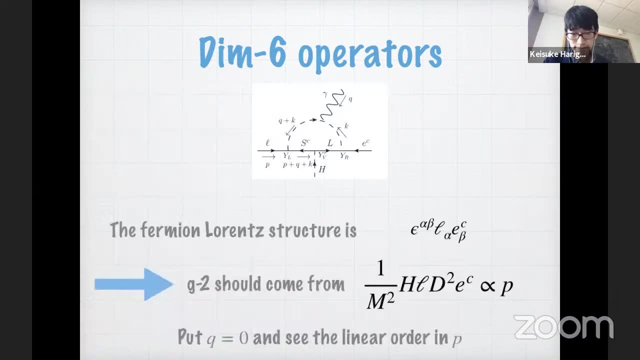 The second one has two diagrams, And for the second one we must sum over two diagrams, of course, to maintain J-G invariance. So let's start from the first one. So here you can see that fermion-Lowrance structure. 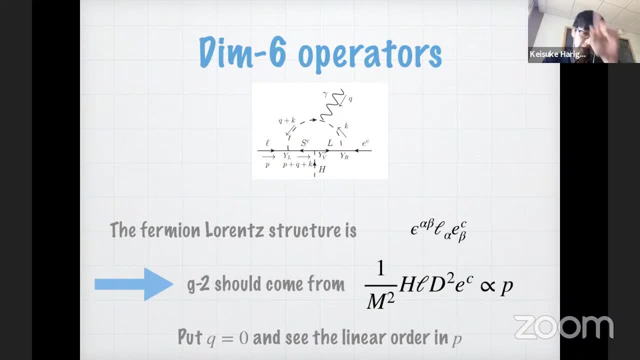 is trivial. There's no Pauli matrix inside because there's no gauge bond attached to the fermions, So the fermion-Lowrance structure is trivial. So then the G-minus two at amplitude level should come from this second dimensional sixth operators. 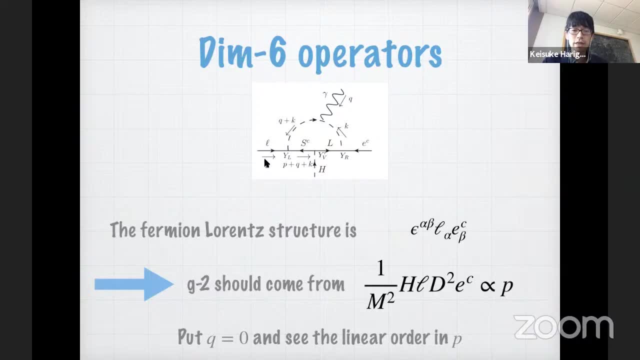 So Fitch is proportional to the linear power in the momentum of the x-axis. This is the external fermion. So to compute the distance G-minus two, we could put Q, the momentum photon, to be zero and look at the amplitude to the linear order in P. 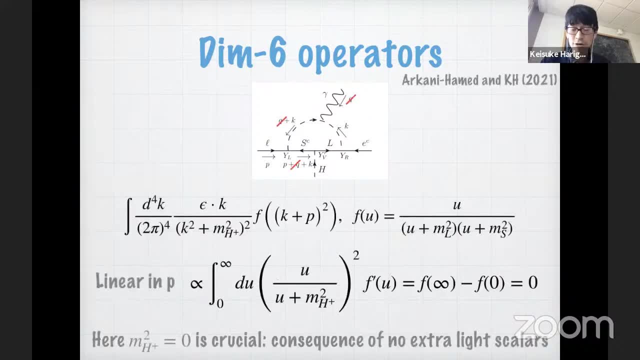 So let's do that. So then, this is the intermediate step. So let me explain how each factor comes. This epsilon times K just comes from this part, photon, the charge-Higgs interaction, And this blue part comes from just the propagators. 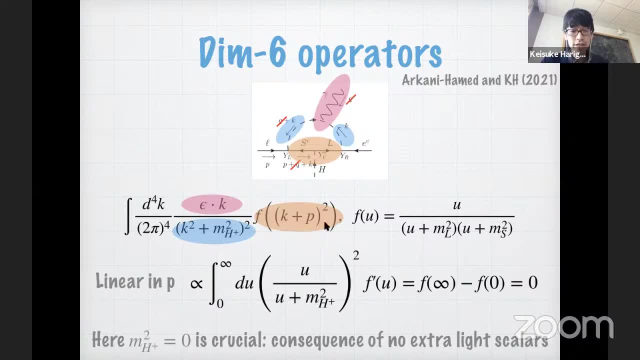 of the charge-Higgs, okay, the momentum weight And this function F comes from these propagators of the fermion and its express form is given here. So here charge-Higgs, which is in the standard model, is massless. 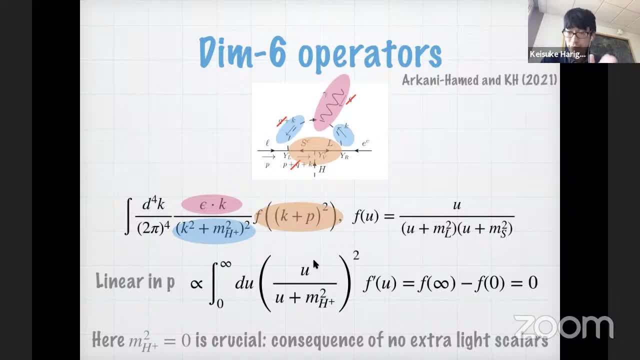 but to clarify what is massless. What is massless? What is happening is I keep that mass as a free parameter for 10 seconds. So if we expand the amplitude to a linear order in P, so here this is what we have. 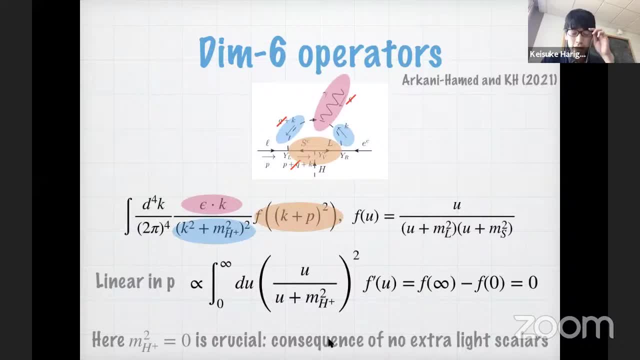 So here U is just K squared with the Euclidean signature. So then, and since we expand to the linear order in P, we have the derivative on F, the function F. So if we put the Higgs mass to be there, 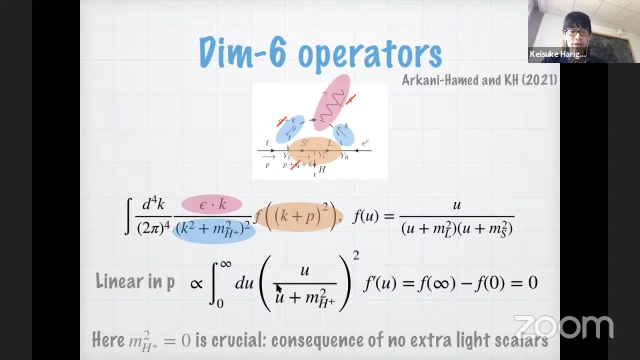 as is the case for the standard model, this is integration of the total derivative. so Fitch pick up the UV boundary value and the IR boundary value and Fitch vanishes. So here you can see that it is crucial that the mass of this scalar is zero. 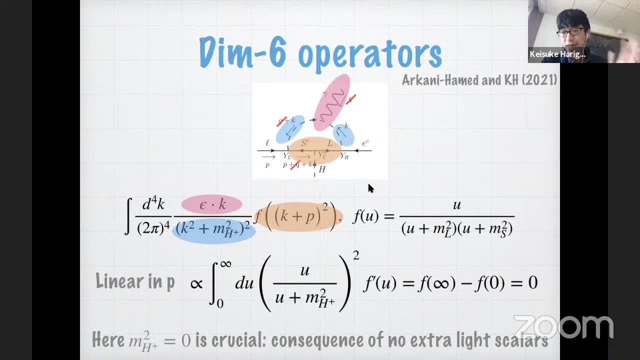 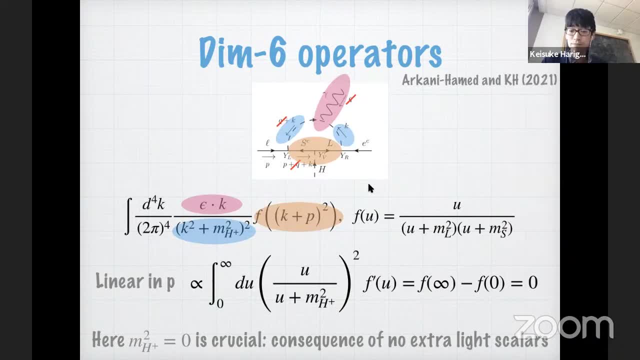 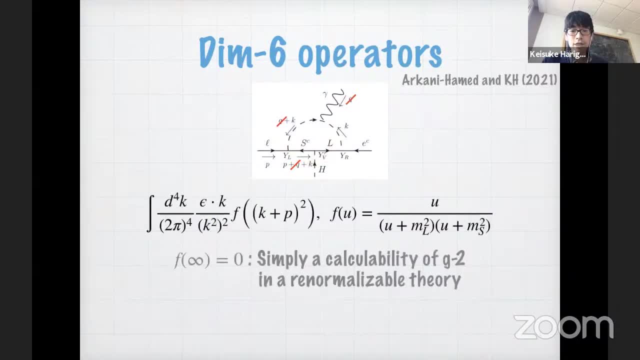 because of the scorohampoo is not going to contradict the those viruses because the sting goes out. So this function still have neither the R one nor the F three, but this function in circled模 passage not going to confuse them. So since this Over- Top, 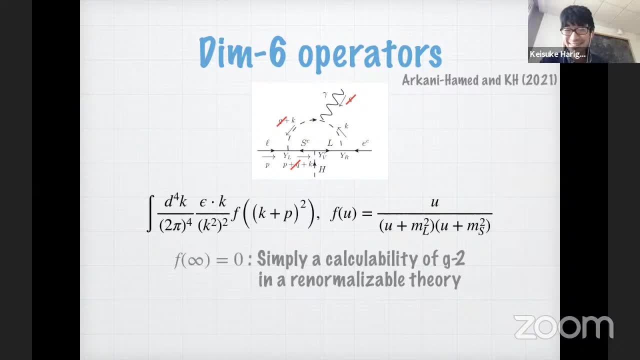 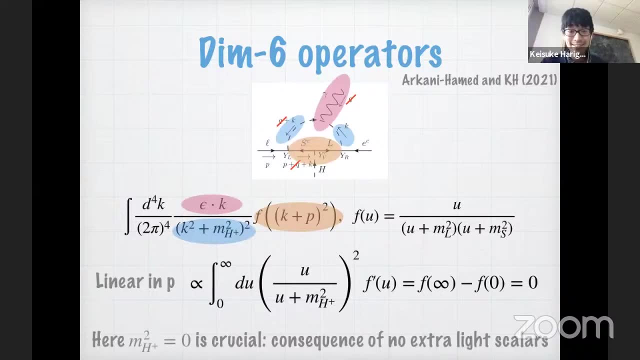 we are just going against the gravitational chain, Table R. Thank you, Can we go back to the previous slide? This one, Yeah, this one, Because I'm trying to say that it is much simpler than you are describing. Because, first of all, you are implying that this implies that 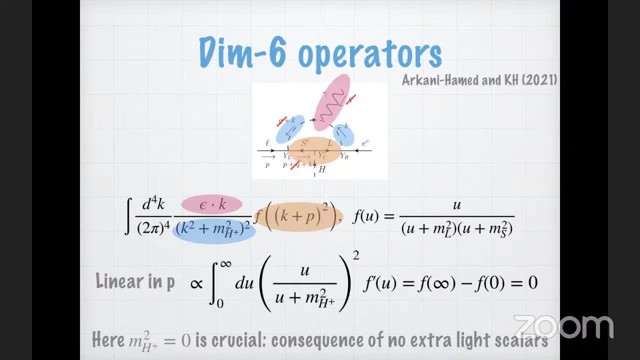 OK, forget about gauge coupling, right, Because it's just H, Because in principle there is a kind of this relation between. you know, for example, in unitary gauge, for example, the diagram would not exist even, You see, because H would be having only, I mean, zero charge component. 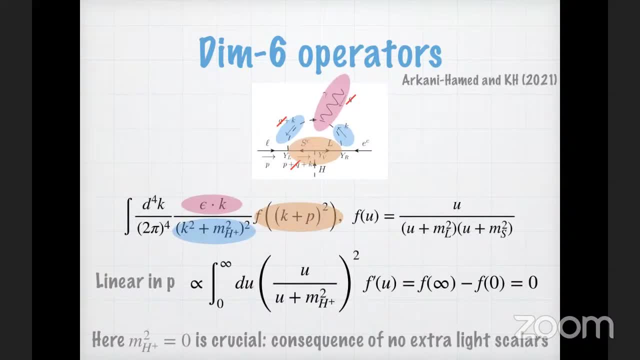 OK, let's take it as it is, as you're describing. OK, now let's cut the loop. Let's consider the diagram without photon and it would be initial lepton, final lepton and three Higgs right. 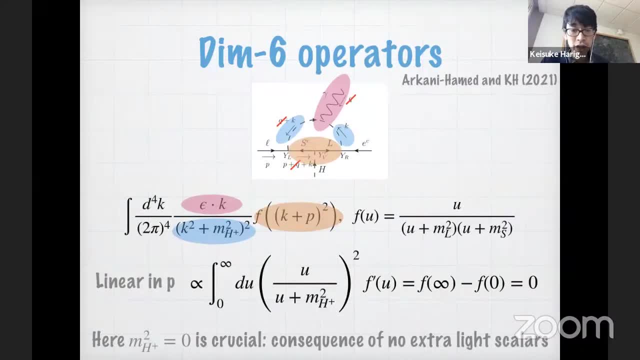 Three: one Higgs- Sorry, One Higgs, which is you have going down, and two other Higgs which then form the loop. OK, OK, OK, yeah, So you have a diagram where you have three external Higgs. 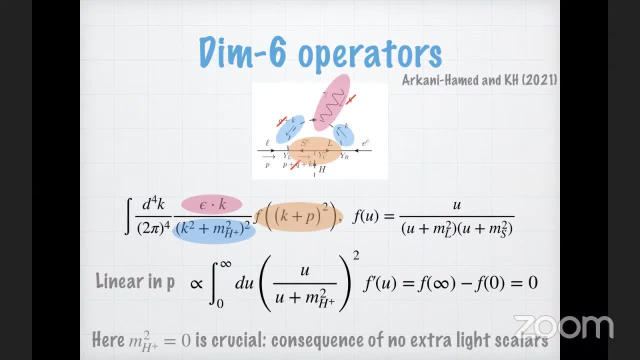 And two leptons right And, as you mentioned already yourself, the structure of the diagram says that spin indices of these leptons are convoluted, So it means that leptons form spin zero. OK, and it is just a three-level effective operator which contains three Higgs. 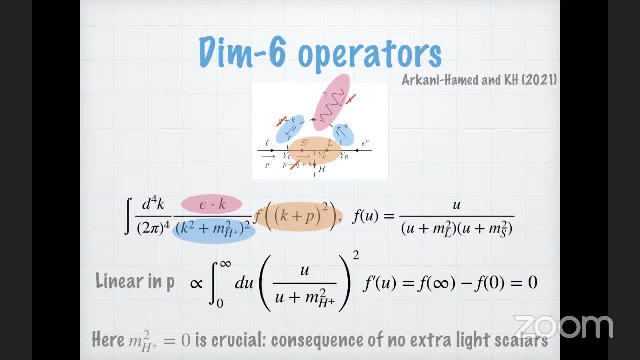 And leptons in spin zero state. It is before loops. OK, now and it is. I am trying to say that it is a three-level of Wilson operator product expansion which gives you this operator cube of Higgs field and leptons. 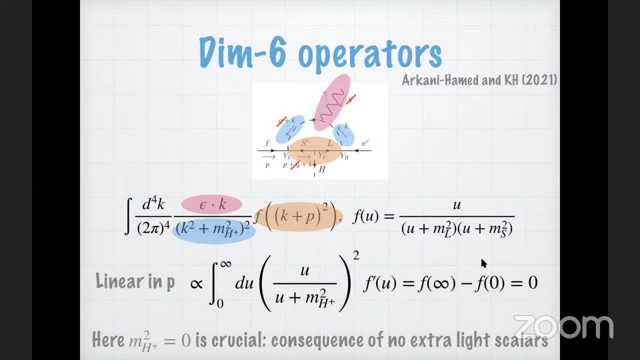 OK, and then of course you can say: aha, let's consider magnetic segment of this operator With full photon or whatever, But however, once my leptons are in spin zero state, then it will never generate magnetic moment operator. whatever you do, 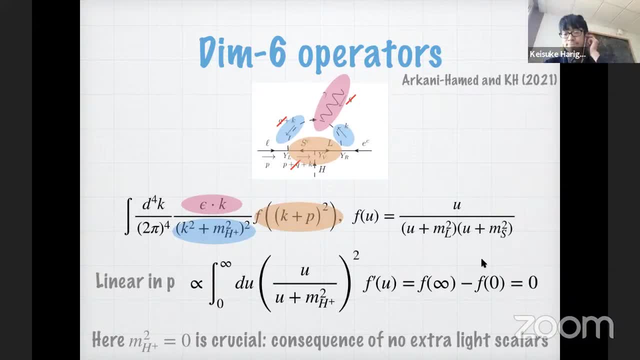 So this constellation is predictable, But still so we can just then consider the next high-dimension operator. No, no, no, But at this level I am trying to say that This explains why you are getting this total derivative, because the matrix element of this operator could not produce magnetic moment. 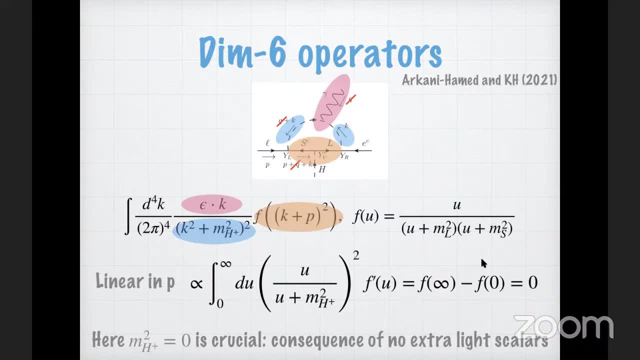 Because my operator, this original operator I am talking about, is contained in spin zero state and you may not spin zero state in leptons to have this magnetic dipole moment. So in this way you are No when you are calculating. 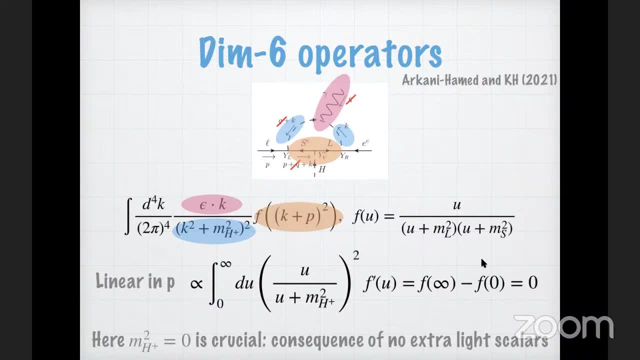 it is including your loop calculation, But I am trying to factor out this three-level path from loop path. But still, I mean you are talking about dimension six operator here, But I mean we could consider some higher-dimension operator. No, no, no. 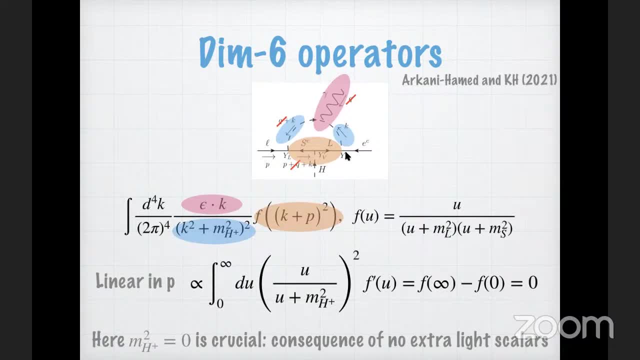 No, but just a moment. It would be Because, at the level I consider, I did not introduce derivative external momenta, So I did not need them. At the higher loops you probably would consider external momenta. then it would be a different story. 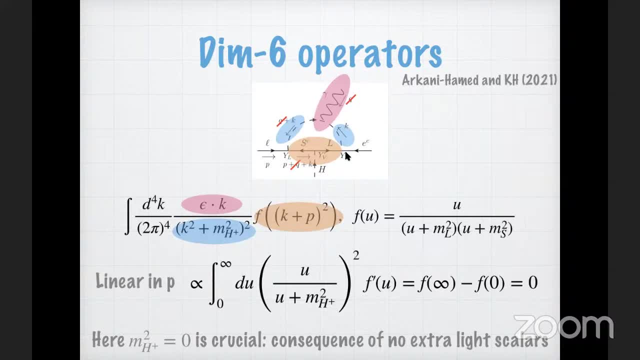 But at the level of discussion we have now of this dimension, Okay, for me what I described is the dimension five operator, right 3H. No, no, dimension six operator. Dimension six operator. But the fact that leptons are entering a spin, zero state. 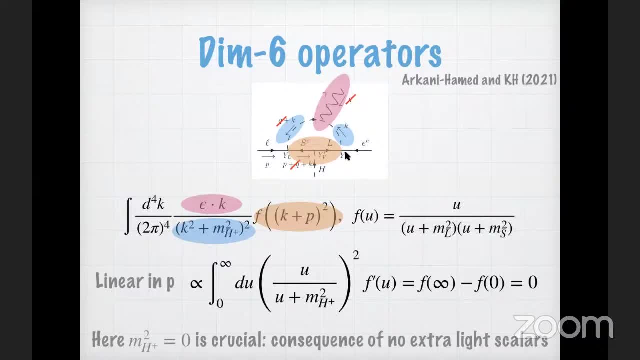 it's enough to explain this vanishing. That explains why there would be no logarithmic correction from dimension six to dimension seven. We still have, from the effective theory point of view. we have dimension eight, operator that can generate dimension six through quadratic divergence. 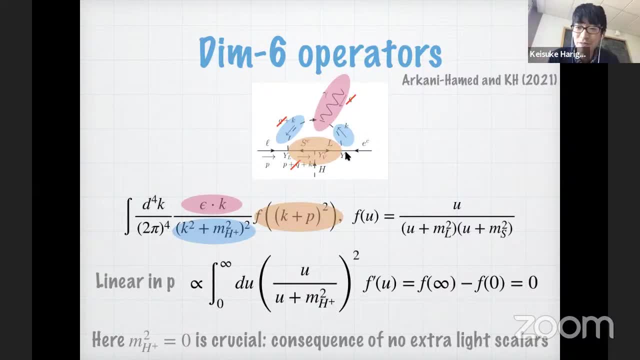 Actually, I will get to that later point. Maybe we can discuss that again. No, no, but look, I'm trying to make He only focused on this particular part. I'm trying to say there is no surprise. No, no, no. 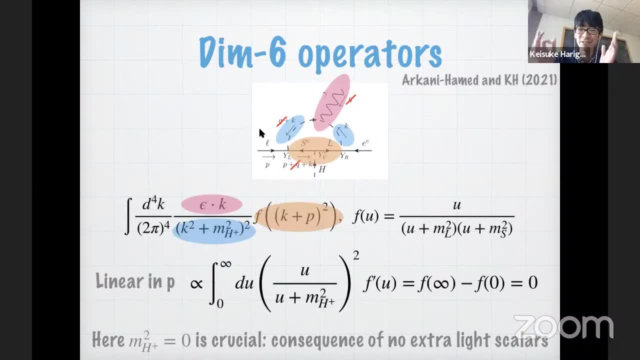 Even for this particular part that is not enough. You can just simply look at a dimension six operator, at the logarithmic theory. I'm not sure that I follow. What they are doing is just look at this effect operator after integration S and L. 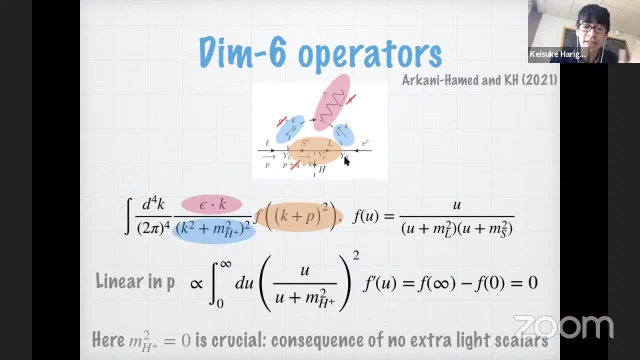 That is dimension six, And argue that that dimension six operator will not generate this dimension six G mass operator, That's what I agree with you. But to argue that G mass should vanish, if you want to use the logarithmic theory, we must also look into the dimension eight operator. 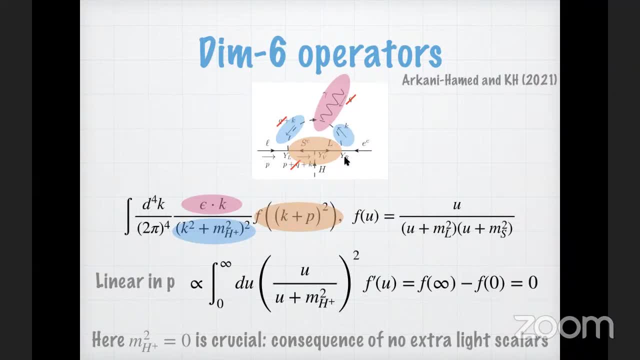 that can generate dimension six operator by quadratic divergence. Okay, just a moment, We are talking about different stuff, Because here we are talking about an effect which is mu square divided by a heavy mass square, right. Okay, However, from the dimension eight operator, 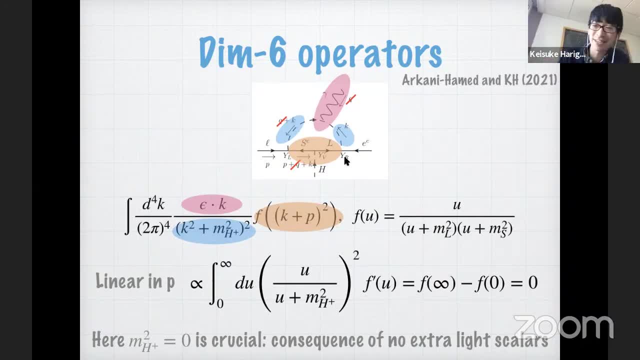 if you have a quadratic divergence, you can generate dimension six operator. No, no, no, Wait, wait, wait. M square over M fourth, So you can't simply look at dimension six operator in the logarithmic theory. No, no, no. 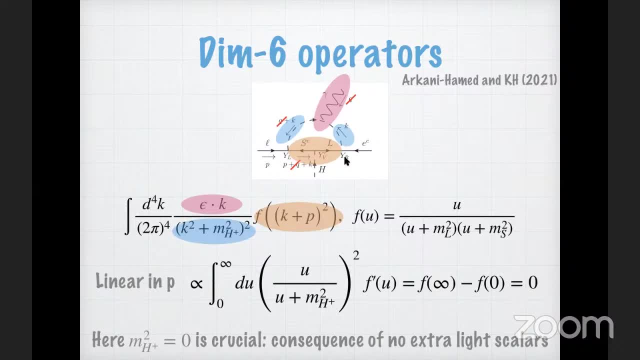 Wait, wait, wait, wait. It is a point which should be clarified Normally, as we discussed the correction of the order of mu square, divided by heavy mass square. right, Okay, When you are talking about higher dimension, you are talking about correction of mu to the fourth. 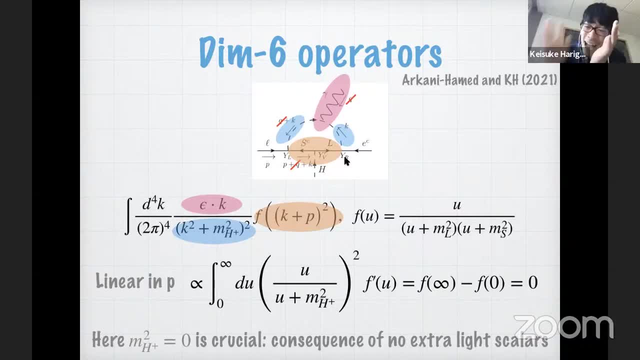 divided by mass. to the fourth: Yes, but however, if you look at the dimension eight operator in the logarithmic effective theory, the quadratic divergence could generate dimension six operator and compensate one over M. fourth: I do. I do not follow, Because once we started, 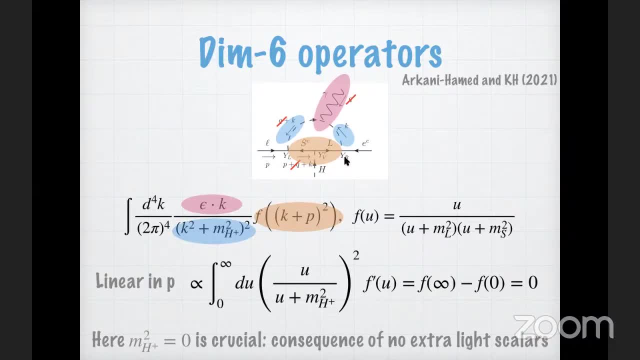 we found dimension six operator in the three level. In the three level, And I'm saying that the dimension six operator in the three level doesn't exist, Not, doesn't exist, It doesn't contribute later on to a magnetic moment, It does exist. 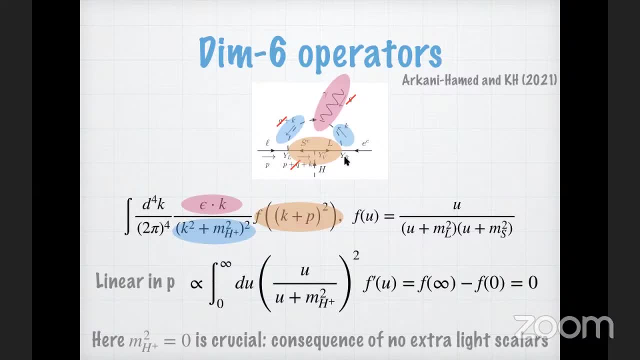 but it contains spin zero structure out of lepton And that's why, whatever you, if you are talking about this particular dimension six operator, it never would generate. Okay, You still don't discuss operator of higher dimension as also a three level. 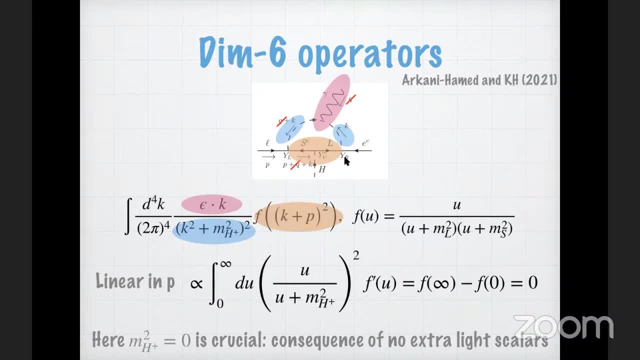 Mm-hmm, Mm-hmm, Mm-hmm, Mm-hmm. Then discuss what's there, but it would be no mixing between these two states. No, no, no, no, no, no, But but yeah. 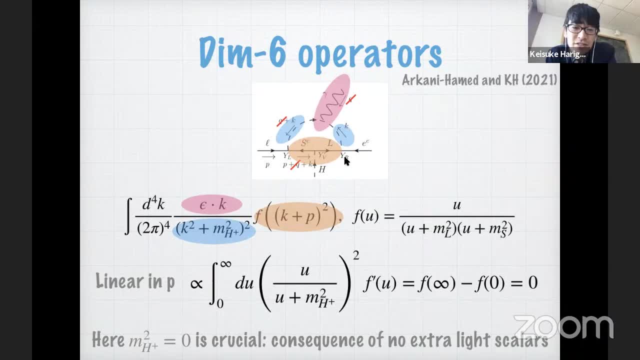 at the RG? no, But if you wanted to use that logarithmic effective theory to show that G minus vanish, you must think about the quadratic divergence, which is of course absent in the low energy RG, but generally it exists. Forget about divergences. 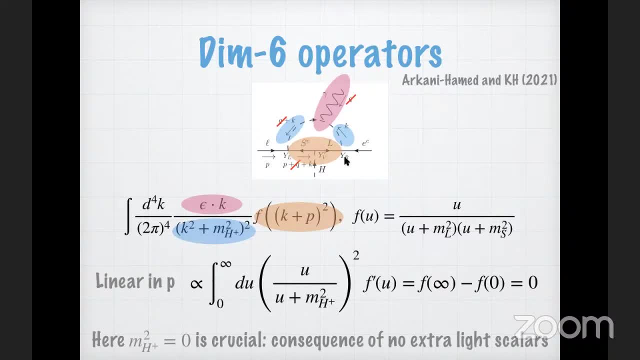 You do not need to think about divergences, because everything in this case is finite. Okay, Because, Yeah, yeah, but that divergence is actually that. just, I mean that, yeah, in the full theory, But my point is this: quadratic divergence. 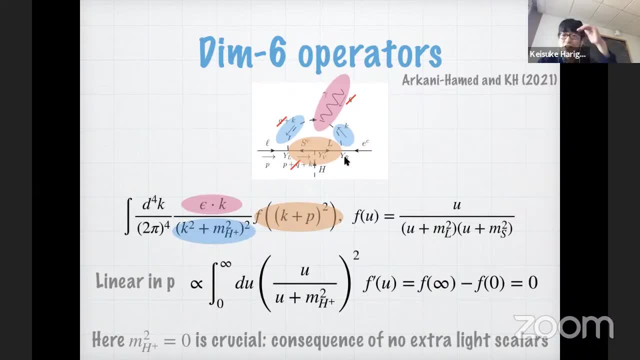 in the low energy, in the low energy effective theory suggests that there could be UV contribution. But but what means UV contribution? Well, here everything is completely fixed, because we know what is UV Mm-hmm Once we. I just said before. 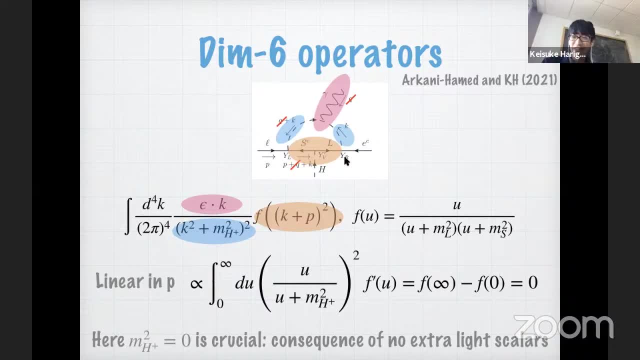 we know what is UV, So we are looking In the in the net. you use effective theory: Yeah, So you can't say that this is finite. Just use dimension six operator. Yeah, There could be the dimension six operator generated from. 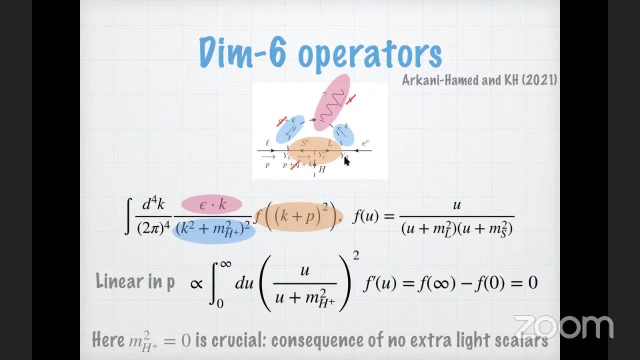 the quadratic divergence and dimension eight operator: Mm-hmm. But I think it's. it's still not important because once, once you are doing this kind of Wilson operator product expression, it is a way to account for UV right- Mm-hmm. 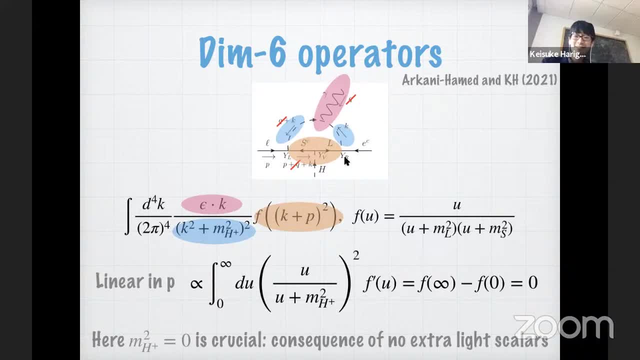 Because you are saying the UV is provided by heavy quarks, right, Mm-hmm, And we are looking for the effect of this heavy, heavy quark. So this could be as mu squared, divided by capital, M squared or mu to the fourth. 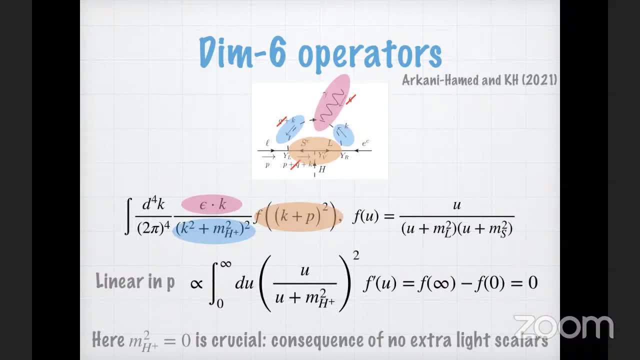 divided by heavy mass of positive force, Mm-hmm. So to discuss this kind of heavy- heavy I mean different type of divergence or whatever. eventually the results should be formulated in terms of coefficient of quadratic mu over M or quartic. 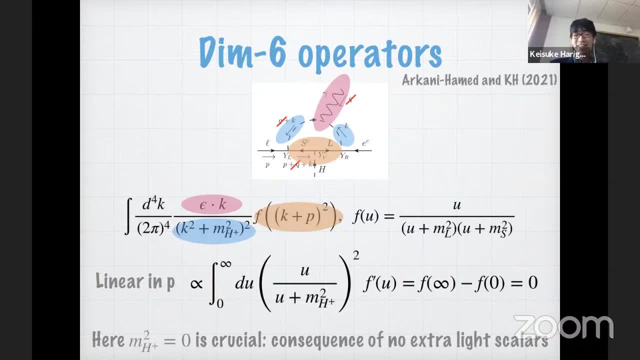 mu over M. That's it. It's the answer. In that formulation there could be UV boundary condition of dimension six, operator. that contributed me on G minus two And you- I mean you- you can still prove that there is no. 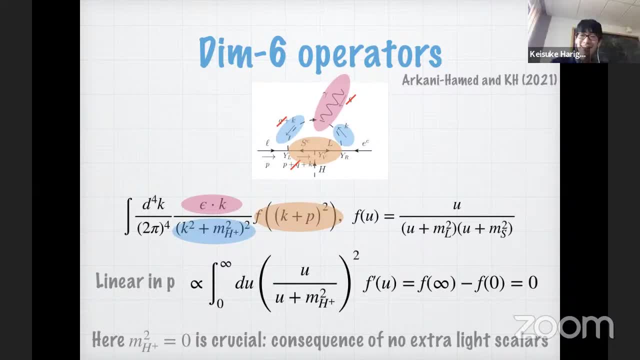 mu squared, divided by M, squared right. It is your proof, Okay, Okay, And I am. I am trying to give you an argument that this is indeed true, But I am trying to say that my argument is simpler than yours. No, 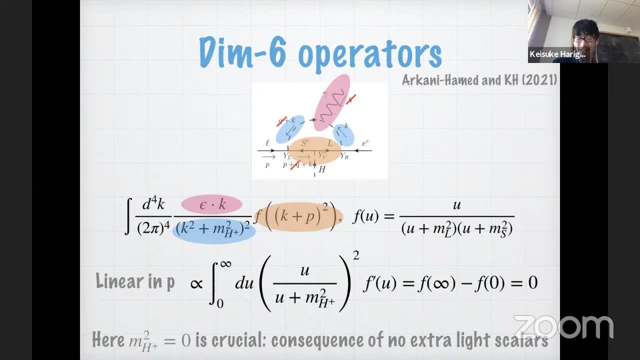 no, okay, my argument is, your argument is wrong. No, it's not enough. It's not enough to prove that mu to the fourth divided by M to the fourth, But for, for the purpose of this particular consideration of one loop, you did. 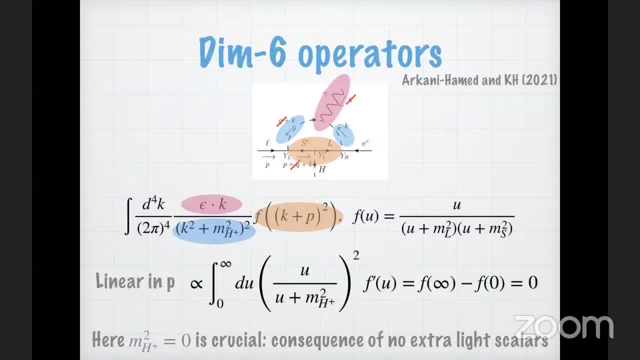 for this purpose, it's enough. No, no, no, I disagree. No, I disagree. Okay, but but it is. but you, you can disagree, but your result do agree with what I am saying? Okay, okay. 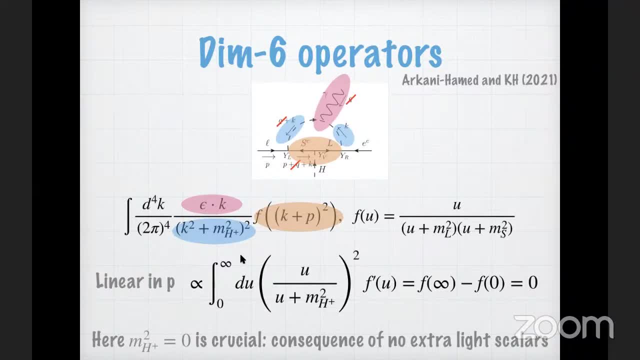 Okay, so I liked the way you agreed, that you agreed that this is totally finished with Te movie, Because So I, so I would like to, I would like by thank everybody for, for, for, for the in here, end here, and beauty is interaction, and you know that you can go to the gauge where H plus is zero. 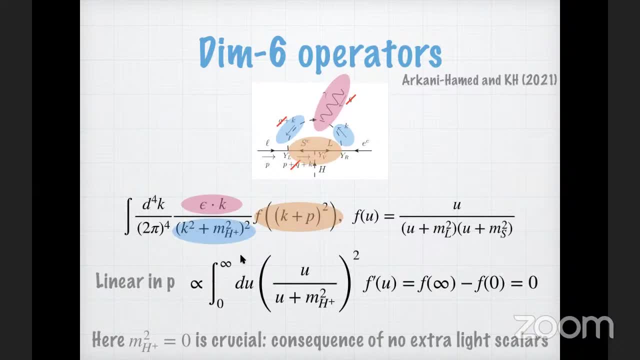 So why do you refer to H plus, which doesn't exist in the standard model? Then even for the unitarity gauge we have a corresponding diagram. Yeah, You should correct that. That equivalents to this computation As long as the rebound momentum is above the electric scale. 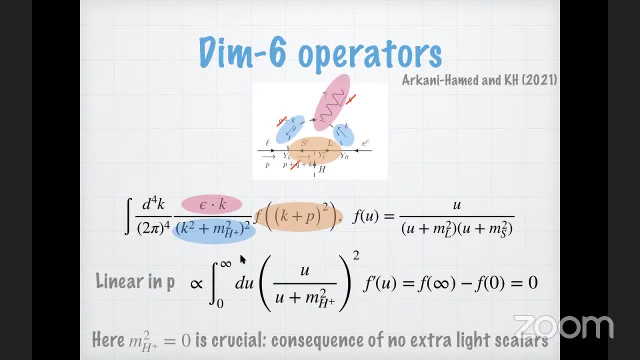 Right, But then we are talking about the effect of Mw. So in this way, when we are talking about normal Higgs and you neglected Mw. So in this way, you are considering the case where the gauge coupling is zero. 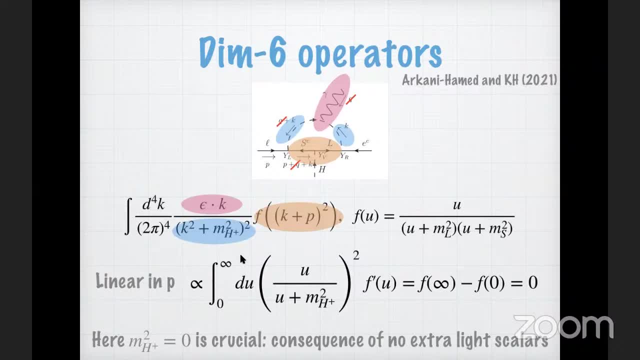 Okay, then, when the gauge coupling is zero, then all masses in this particular theory, you should say yourself whether it's a theory with unstable Higgs, whether it's a theory with very unstable Higgs, Whether it's a vacuum average or it's a theory without vacuum average. 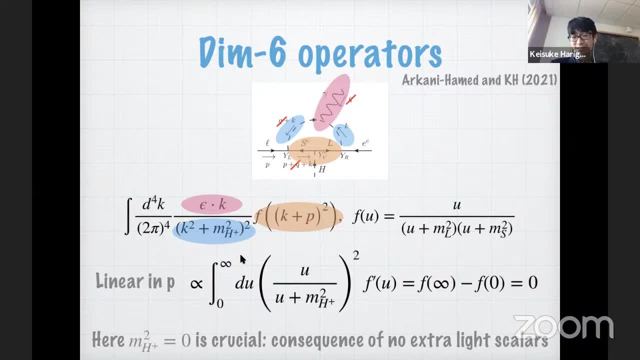 So you did not formulate this. So your Higgs theory, if you are to an unbroken case, right then. I mean, as long as the rebound momentum is above the electric scale, this computation is also fine. But we are talking, at the end of the day, about low energy theory. 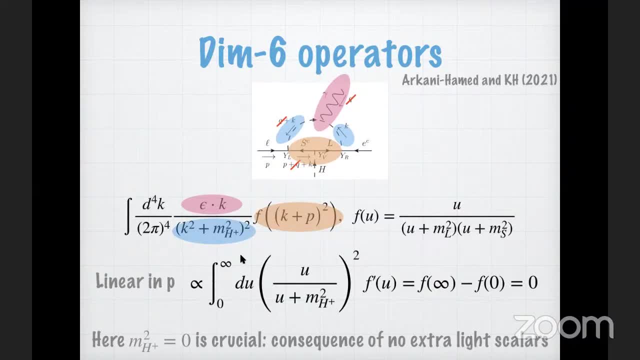 It's important what is the physical Higgs mass, As long as the new Higgs mass is above the electric scale. so this diagram can be well approximated by this golden boson picture, So we don't have to use W boson to see the dimension of these operators. 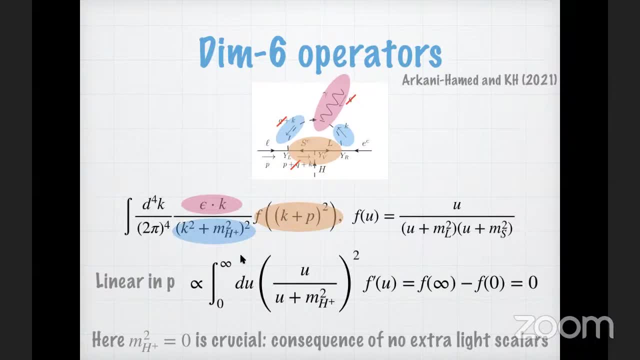 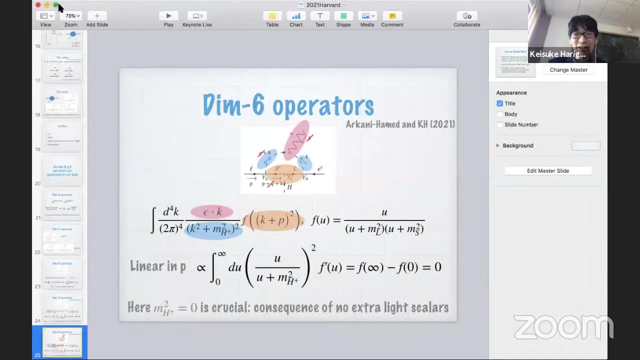 Okay, Either you're considering a standard model or you're not considering a standard model. In standard models, there is no way to pass. That's it. I totally disagree, but let me proceed. We are talking about a physical particle. 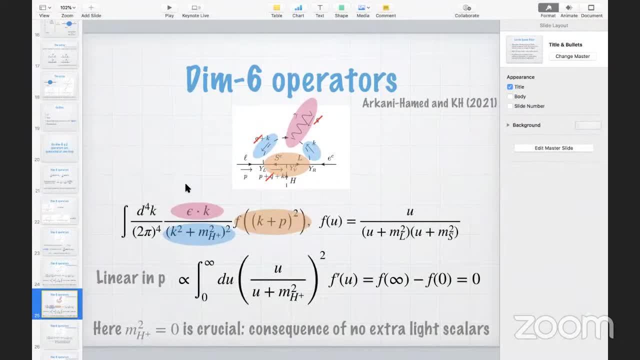 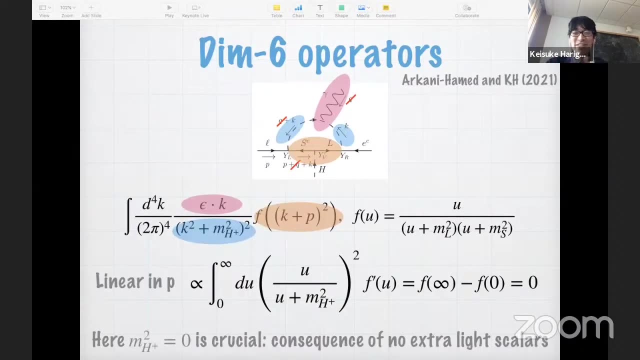 A physical particle. you can count In unitary gauge, it doesn't matter. You can count what are physical particles in your theory. Here this is a computation above the electric scale. So the Higgs picture is also good. I'm not saying that it's not good. 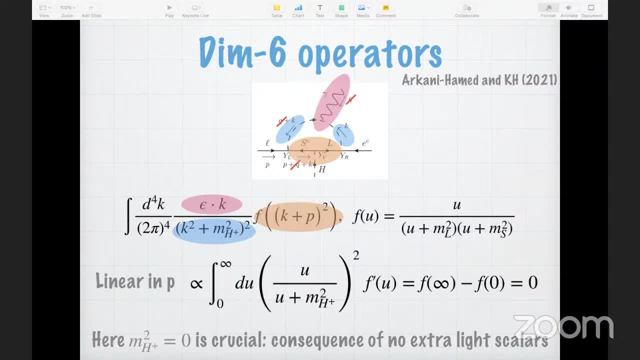 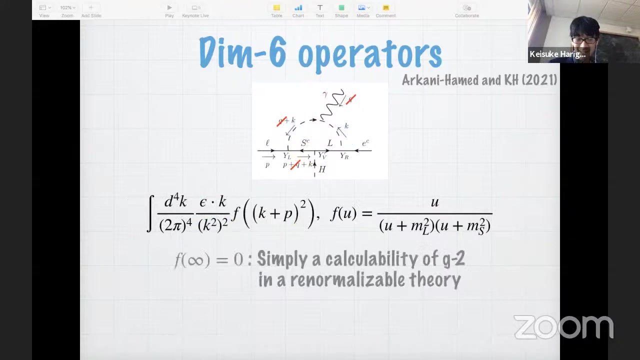 It doesn't make you free from obligation to say what a physical spectrum. Okay, I think maybe you can continue this discussion offline and we can continue with the talk. We already tried it offline a little bit before Mm-hmm, So let's see. 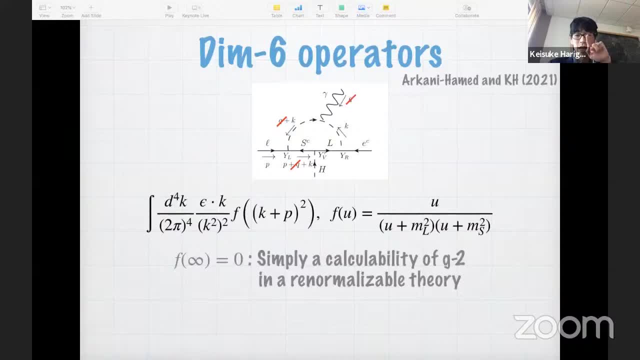 So since here it is important that this function vanishes both at UV and IR. So let me a little bit elaborate on why they vanish at both UV and IR. UV is trivial. This simply comes from the curriculability of the muon g-2 in a renormalizable theory. 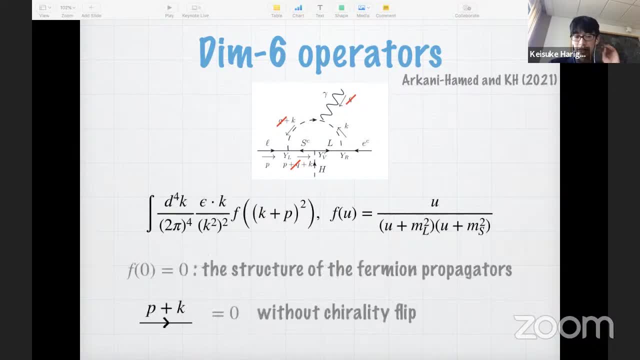 This is rather trivial. What is not so trivial is this function vanishes at the IR, So in this computation. so this comes technically. this comes from the structure of the fermion propagators. So here, in this fermion propagator, it does involve a chirality flip. 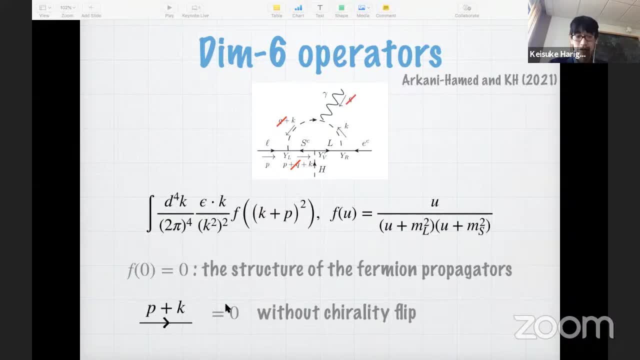 So when the momentum vanishes, K plus P equals 0, this trivially gives 0. So that's why this F0 equals 0.. But there's a more interesting way to see why F0 equals 0 from the symmetry point of view. 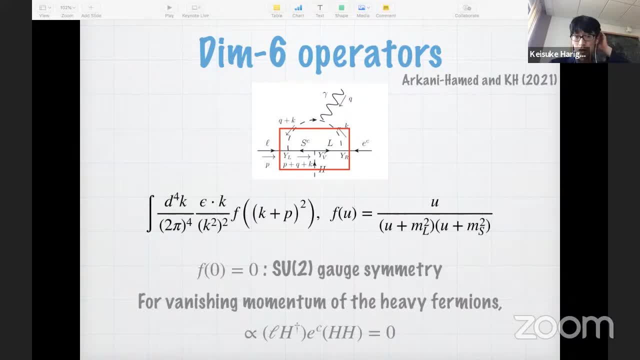 So in the limit where the fermion momentum goes to 0, the amplitude of the contribution from this red box should be expressed by an. It's proportional to an effective operator, without derivative on the fermion. But you can, But let's try to just construct that. 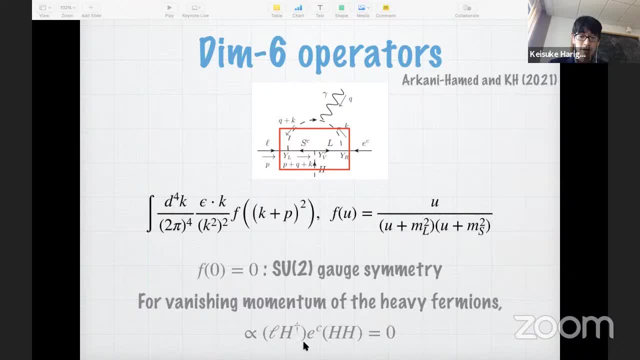 But however so, here the only operator that we can write down is this one. But here, since we use- We only use the standard model Higgs, this HH, which is contracted with the SU index, trivially vanishes. This is why this F0 goes to 0.. 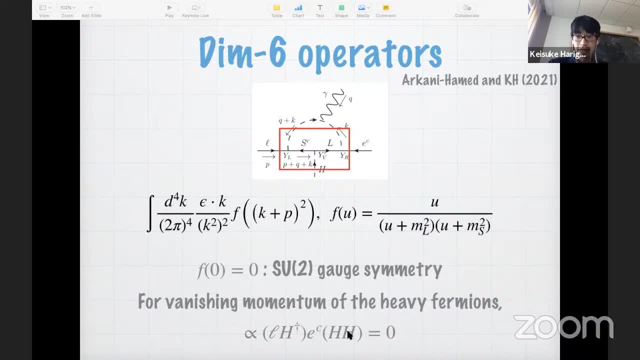 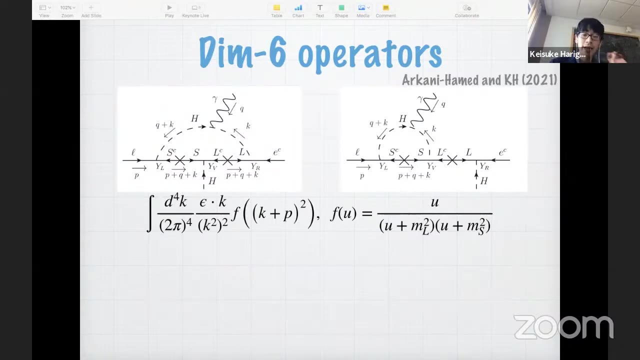 And you can again see that importance. So it's not just an absence of new scalar. If this 1 over 8 is a new scalar, this identity doesn't hold. So now let's check another diagram, proportional to another set of Euclid coupling. 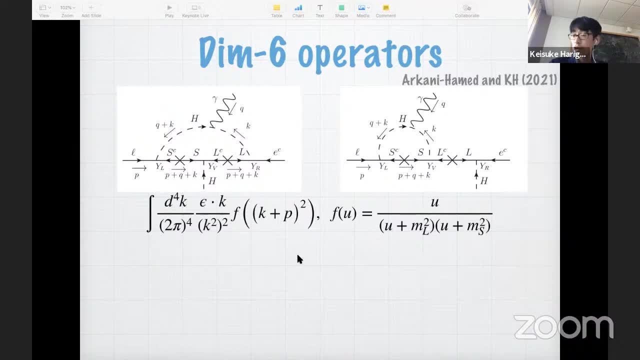 But it turns out that X gives the same form of the quantum correction and with the same function, F. So here the real function of this function is this: The reason why F0 equals 0 cannot be attributed to the structure of the fermion proprietor. 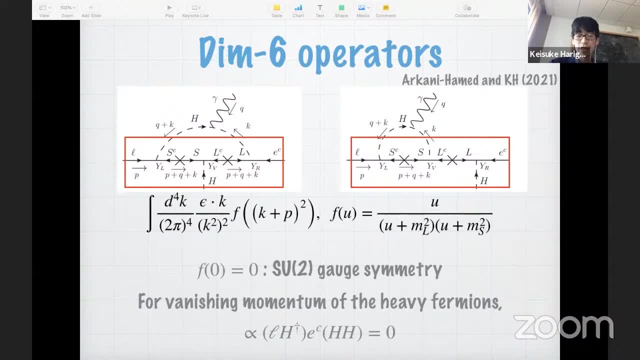 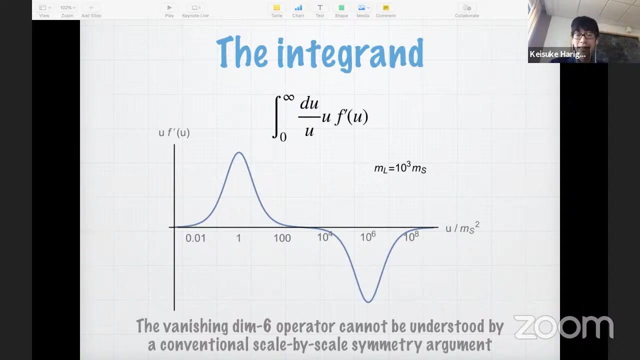 Instead, that should be attributed with the fact that the operator with the derivative trivially vanishes because of this SU structure. Okay, So let's just look closely into this quantum correction And just look at the integrand. So the integrand is of this form: 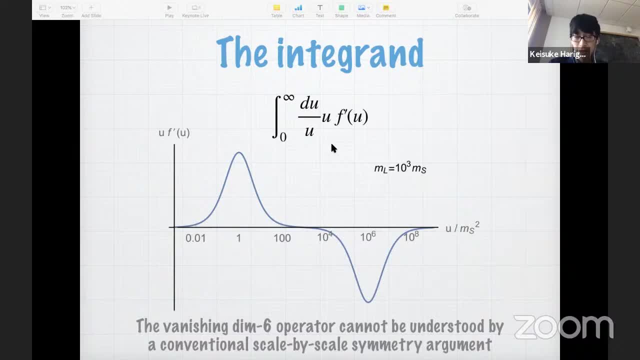 So here I just express this in the log space. So X-axis is the momentum square in the log axis And Y-axis is the integrand. So you can see that the integrand is non-zero at each energy scale. But the integrand 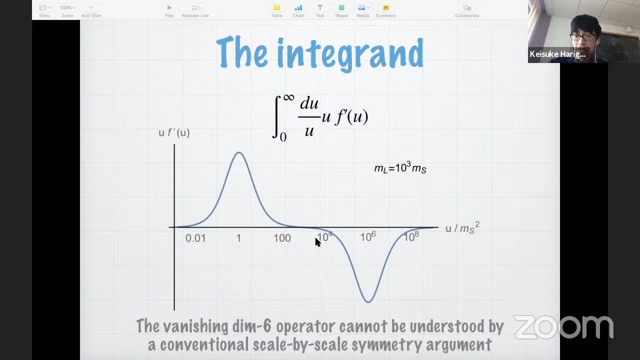 The integration over. it can't stay between these two pieces. So here, to clarify the structure, I took the unrealistic mass hierarchy between the ML, the mass of the doublet, and S, the mass of the singlet. From this you can see that this vanishing dimension 6 operator cannot be understood by the convention. scale-by-scale symmetry argument. 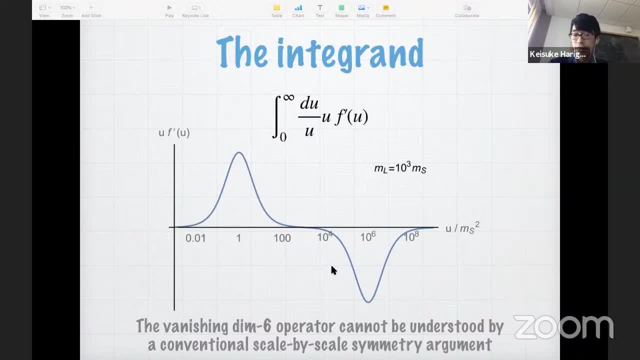 which requires that the integrand vanishes at all energy scales. But look, it is exactly what I said. Once you see that it is dimension 6, operator in T-level contains this spin 0, then this automatically follows: No, no, no. 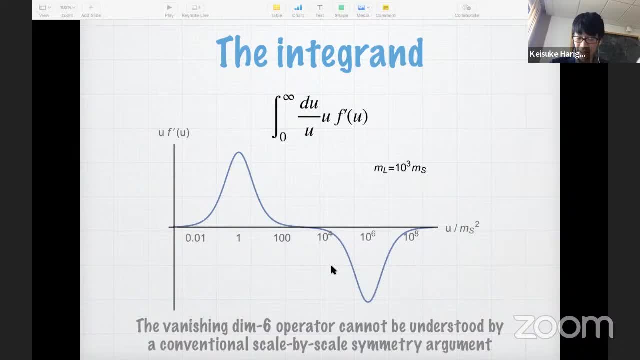 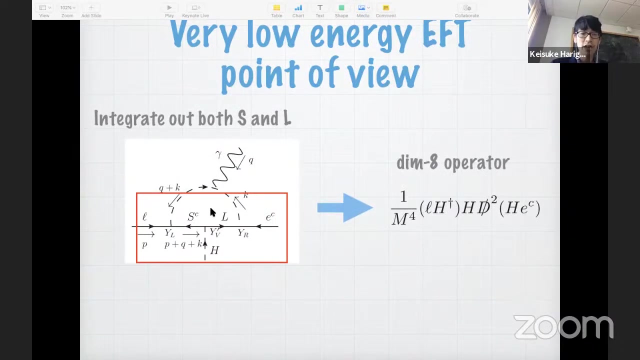 Let me say more about that in a few slides. So let's see Now. let us see this integrand, What's happening in this integrand From the effective field theory point of view, So at the very low energy, so we can integrate both S and the singlet. 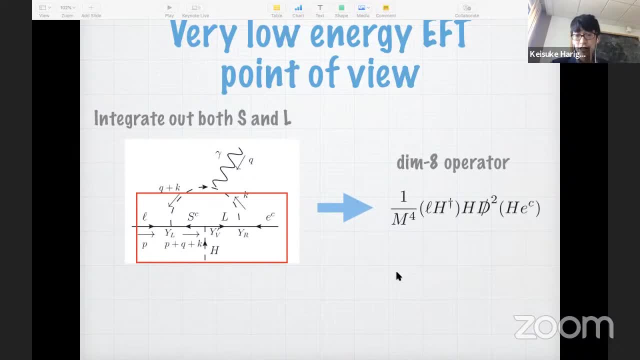 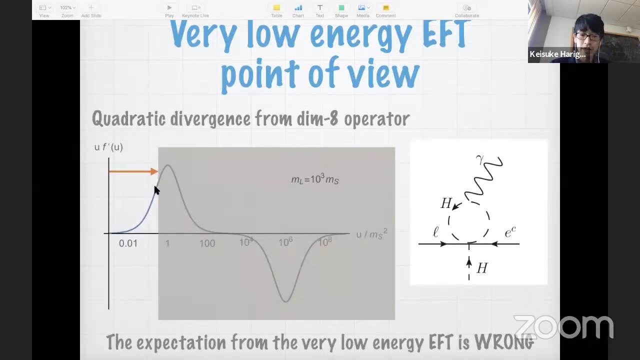 And since the dimension 6 operator vanishes trivially, so we have dimension 8 operators. So then this first peak in the IR could be understood by the quadratic divergence from dimension 8 operator. So we make this. So we may think that from by observing this quadratic divergence, we may think that, oh then we end up with a nonzero muon g mass. 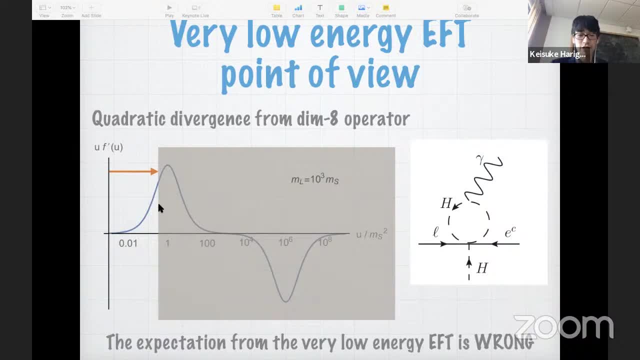 But what happened is, in the full UV theory there is a cancellation between IR and UV And we, the expectation, the naive expectation from the very low energy effective field theory is wrong. So I have this this, could this partial answer to the Al-Qadi's comments? 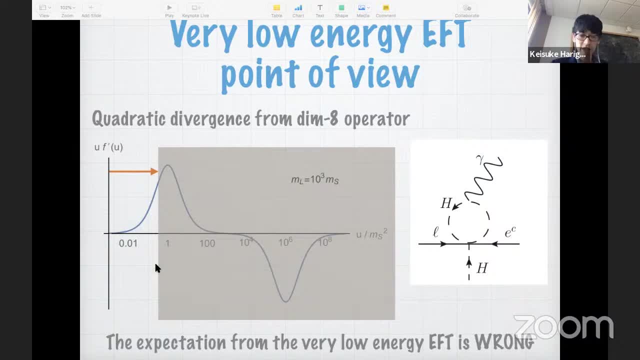 So this is what I said. So from the low energy effective field theory point of view, there is this continuation from dimension 8 operator. It's not enough to see that trivially vanishing dimension 6 operator contains three peaks. Do you agree or? 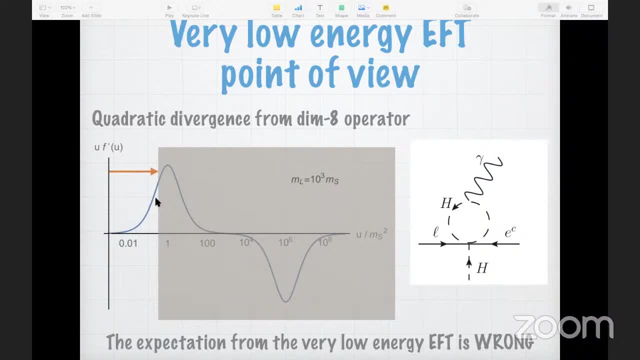 But dimension 8 operator. this contains one over m to the fourth, or what? One over m, fourth? but could be compensated by the quadratic divergence in the integrand. No, no, Just a moment. I am not talking about three level expansion. 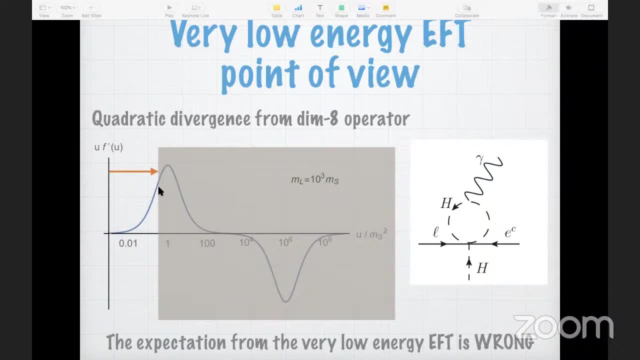 I am talking about three level expansion, That's right. Dimension 6 vanishes, But just a moment. Then you have one over m to the eighth, Four, One over m to the fourth And you have x, derivative from leptons, right. 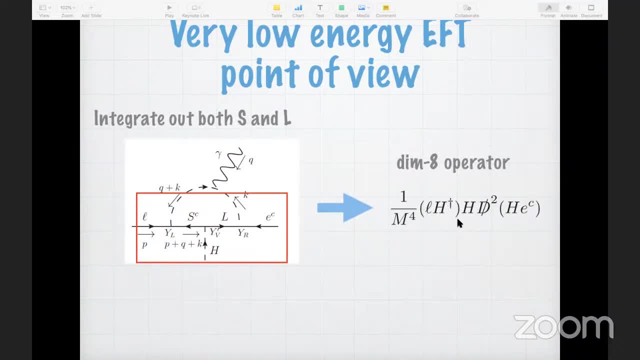 This one, Yeah, Okay. So then, when you have x derivatives of leptons, This x derivative would be like this square: This square acting on leptons, Okay, But this square acting on leptons once we account for photon, then this square would be equivalent to f mu. 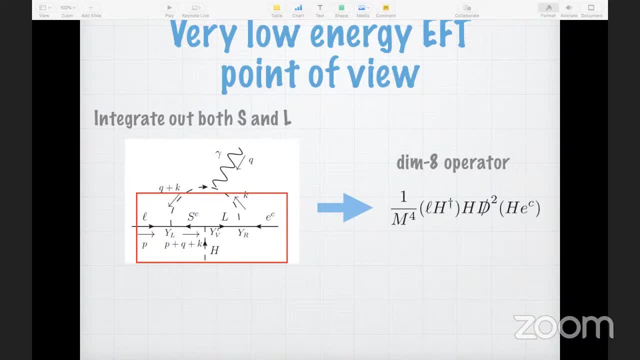 And then I would agree with you, Because then you would have operator f mu. But then the answer would be, I believe would be like, when you're taking this matrix M, it would be like m mu to the fourth, divided by heavy mass to the fourth. 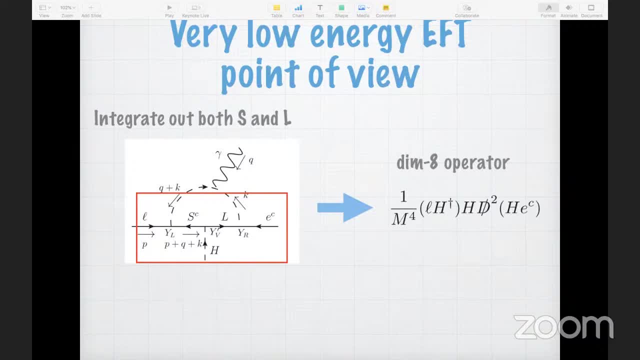 And it would be contribution to magnetic moment. So I don't. But this would be real higher dimension operator contributing to this. So I does not disagree with this. But I'm trying to say that you can still start from three level. Three level accounting for x derivative. 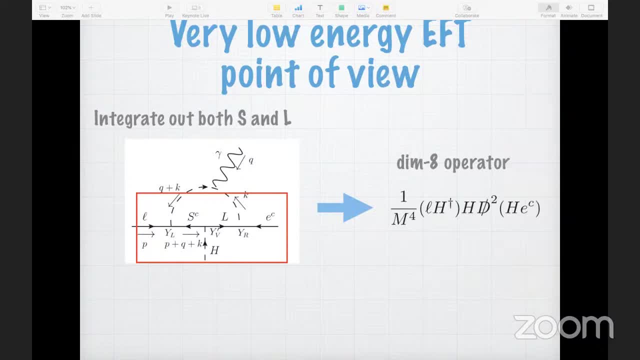 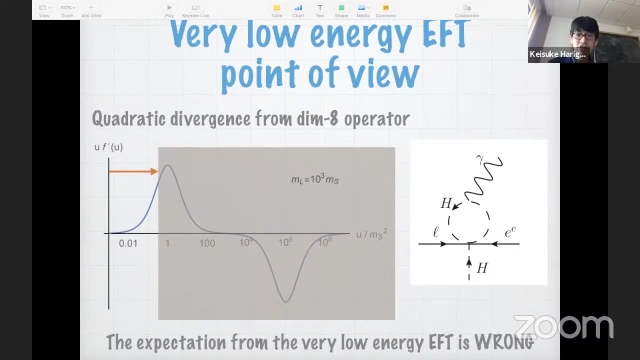 Right. So instead of saying that it is quadratic, you are just calculating how much this contributes Mm-hmm, Mm-hmm. I mean for you we say we can actually compute that. Yeah, All right. But then what you're saying about zero? here it is about dimension six. 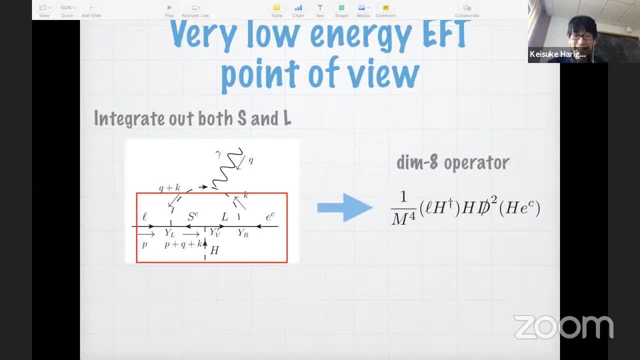 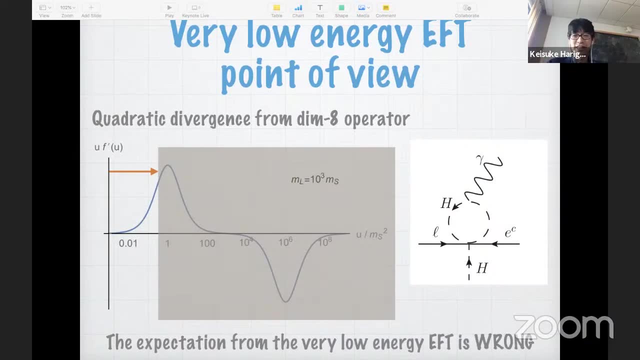 It's not about dimension eight, I don't know. But my argument here is we can't simply look at dimension six operator, at the low energy effective field theory, to argue that the human actually shoots trivial advantages, Because in the low energy effective field theory point of view there is dimension eight operator. 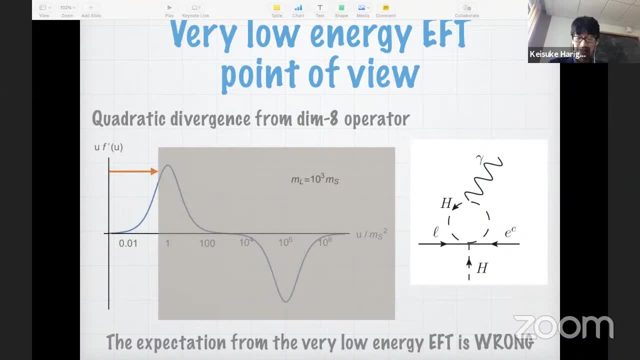 And quadratically divergent quantum correction to g minus two, Which is actually manifest in this integral. You can see that this dimension eight operator You cannot argue right Right. But once you are calculating coefficient for this operator, you can argue. 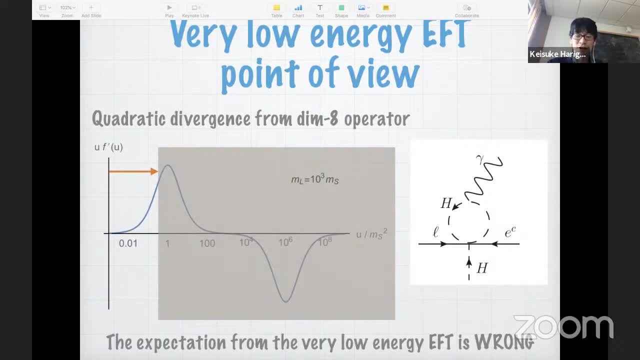 In low energy effective field theory, we can't really compute. No, We have finite, We can calculate. We have finite UV theory. There is no problem here to say what is a cutoff Mm-hmm. So to say that there is no way to calculate this coefficient is not in complete UV theory. 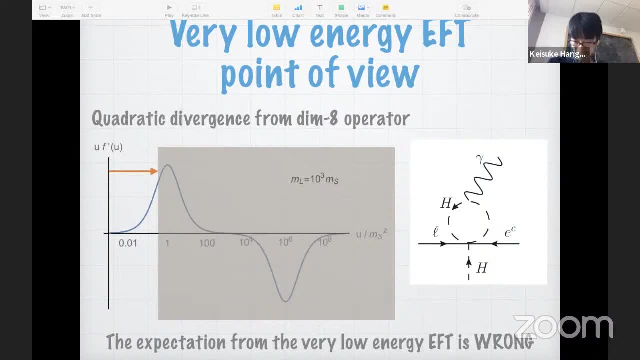 It's not. I disagree. Of course you can calculate it. Yeah, In complete we can compute that. But my argument is that you can't just look at the low energy effective field theory. We must look at the full theory. 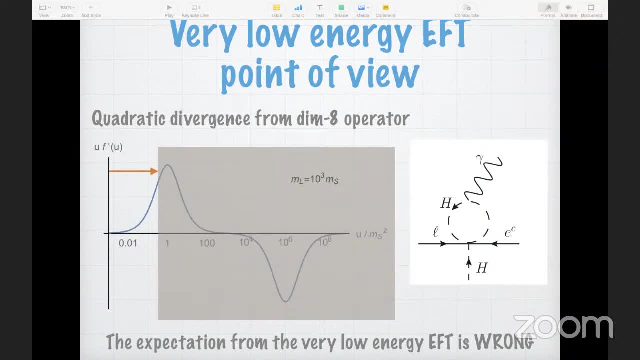 Sure, No, But it is always to calculate coefficient. you are looking to the full theory. Mm-hmm, That's true, Mm-hmm. We really should continue with the talk. Oh okay, I mean, we've mostly spent time arguing. 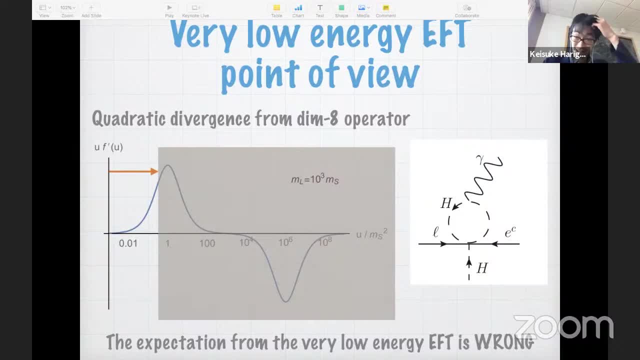 So no more. All right, I'll have to meet you, Okay, Okay, Okay, Okay, Yeah, No, No, But it is still an important issue. No, No, I'm serious. We have to continue with the talk. 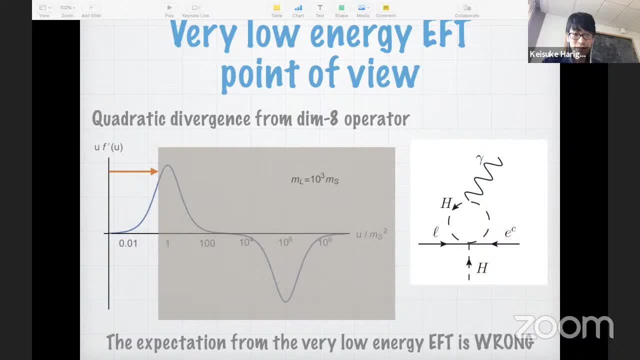 Sorry, Sorry, Yeah, Yeah, Let me continue. But most important point, we will finish very soon. Yeah, Let's see just some comments about it. That's also important. But yeah, Let me continue. We have 40 more minutes. 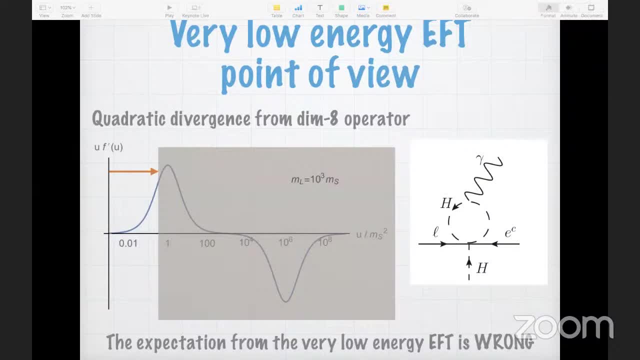 So don't worry about this. Yeah, Go ahead. Okay, Okay, Okay. So yeah, This is analogous to something like this: Suppose we compute the mass difference between charged biome and a neutral biome, Then our live expectation is the mass difference between the charged biome and the neutral biome. 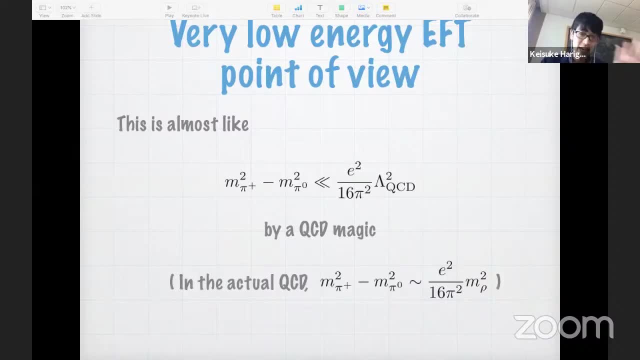 Yeah, Yeah, Yeah, Yeah, Yeah, Yeah, Yeah. So the expectation is: the mass difference is given by the one-loop factor times the cutoff scale of the QCD, which is the Lomason scale. That is correct in our QCD. 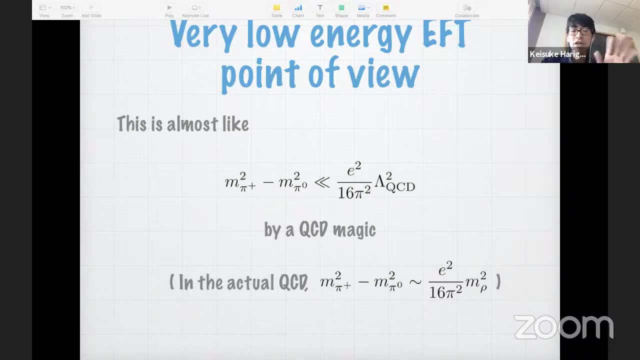 But this vanishing the G-2 is from the low-energy-effective theory point of view. it's something like we compute the mass difference and find the value much smaller than this naive expectation. This is a bit surprising to me, Okay, So. 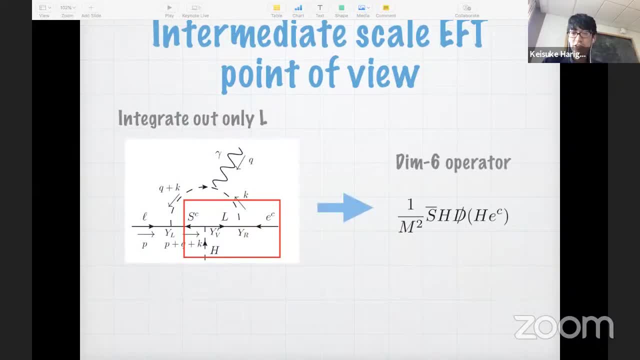 So now we have discussed a very low-energy-effective theory point of view where we integrate both singlet and the lepton doublet. So let us now consider the case where we have doublet singlet and consider the effective theory in between them, where we integrate out this doublet-lepton. 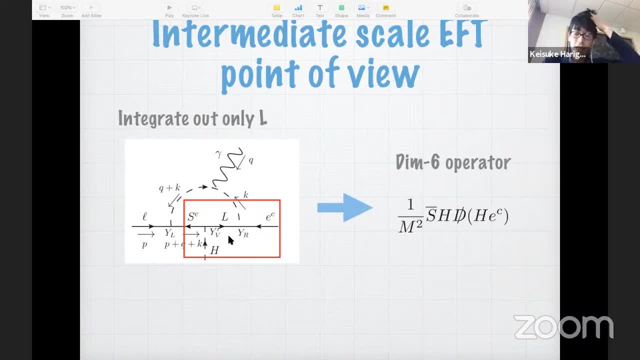 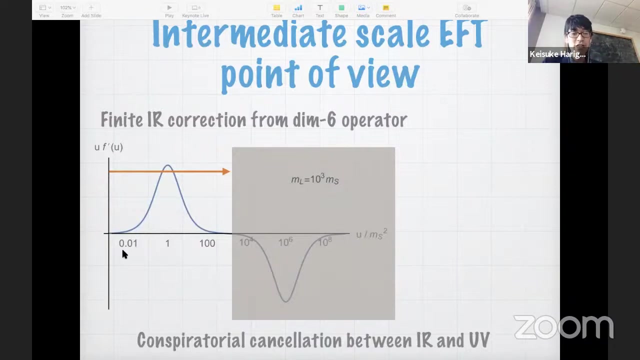 So then, from this part, integrating out the lepton doublet, we obtain a dimension six operator shown like this: Okay, So if we compute the G-2 from this, in the intermediate low-energy-effective theory, we have the correction corresponding to this first peak. 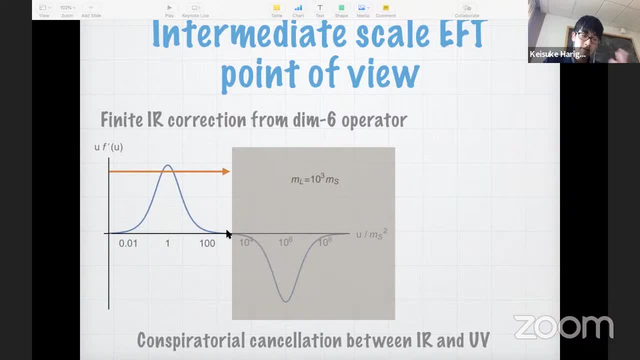 Based on this, one may think that the low-energy-effective theory- there will be non-zero G-2 even in the full UV theory. But what actually happens in the full UV theory is this: higher correction is canceled by the UV correction. So there is some conspiration or cancellation between IR and UV. 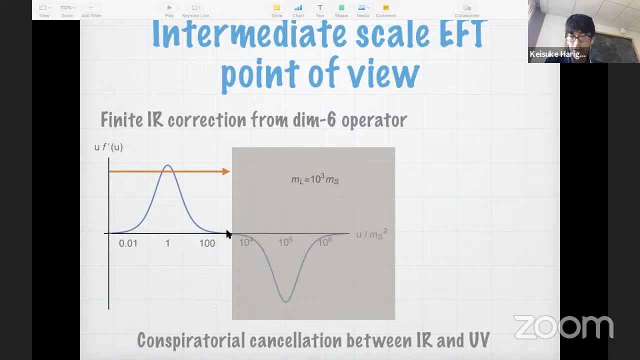 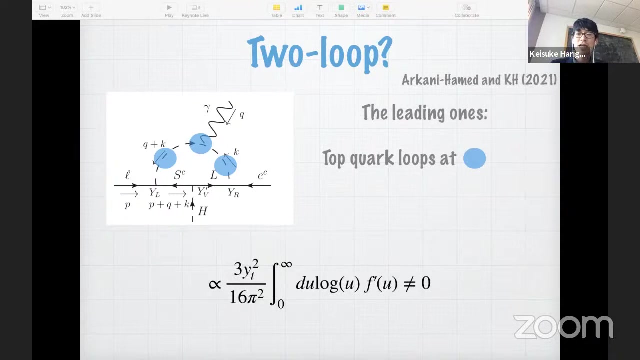 And this again live expectation from the IR-effective theory. that doesn't work here. So okay, well, at one look it vanishes. so maybe the next question: how about a two-look That does? do we have an electronic? does that still vanish? 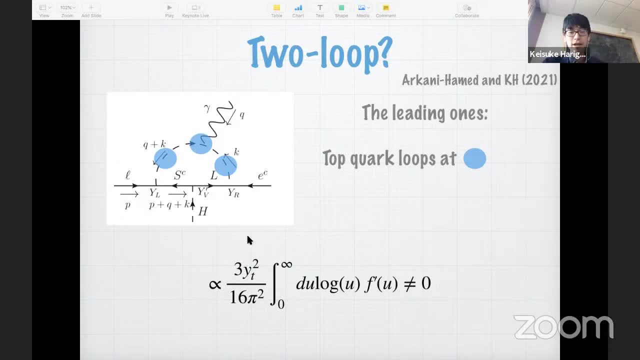 But the answer is no, it doesn't vanish The reading diagrams. The reading diagrams are the one where we add the top quark loop That is bigger, The top quark has an older one coupling with that peak and that gives a dominant correction. 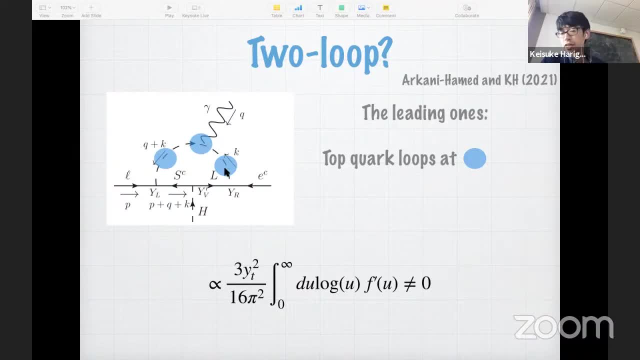 We can insert the loop here, here and here. That can be understood by this wave function renormalization. So the original, this du times f, prime, u integration involves an extra factor of a loss, Okay, Which no longer vanishes. 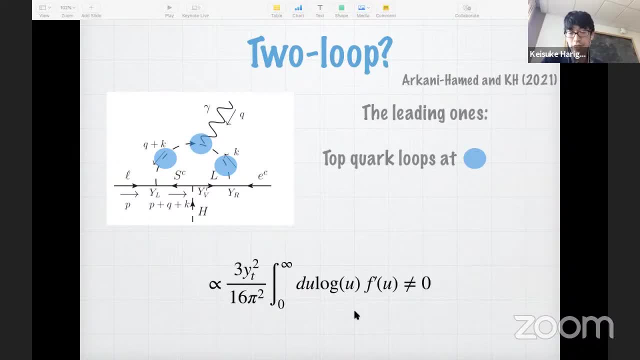 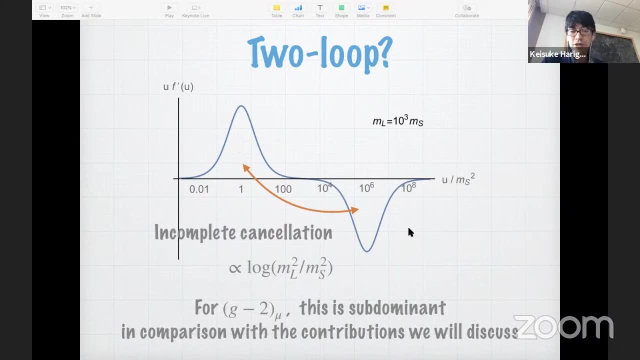 So at the two-loop level we have known the correction to g minus two, And what happened in the integrand is this IR peak and the UV peak has slightly different coefficient and the cancellation between them is incomplete. However, for the observed value of the g minus two, this two-loop correction is subdominant. 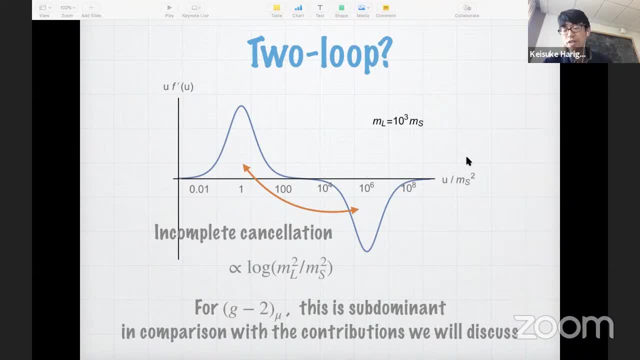 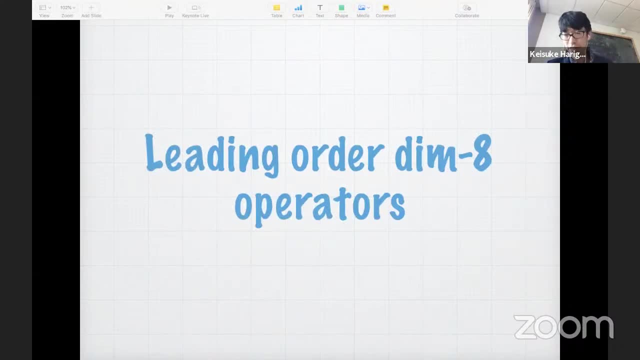 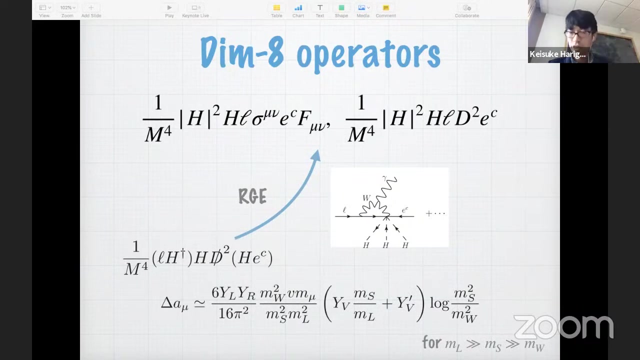 in combined with the integration. Okay, So this is what we discussed in a few minutes. So the reading one is given by dimension eight operators given by this. So in addition to the dimension six operator, we just add extra two Higgs's. 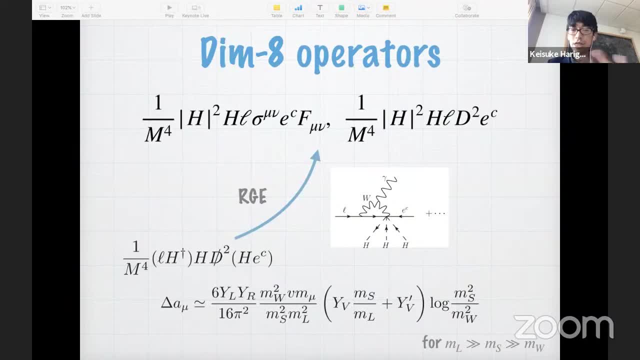 So this might be the appearance of this dimension eight operator from the viewpoint of the effective field theory may be understood as RG correction from this dimension eight operator. Okay, Okay, Okay, Okay, Okay, Okay Okay, Let's check this one just to see if those areas are grainy. 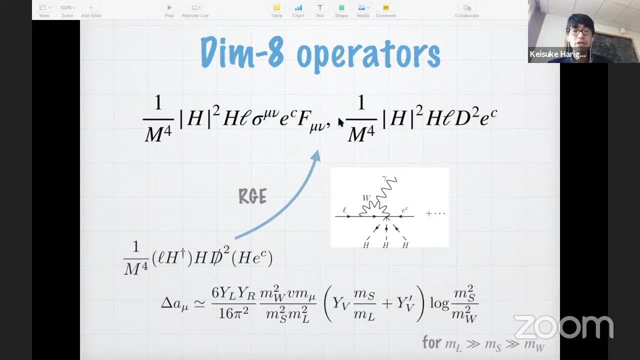 Let's just change one view of this region and just say one position to in your vision. So if you will only see this one, this is some of the 離線 you have discussed. Okay, Okay, Okay, Okay, Okay. 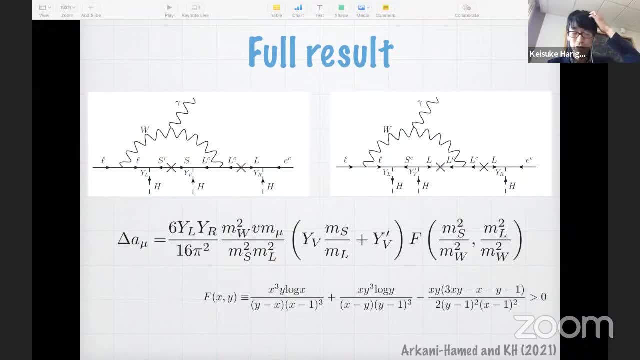 Okay, Okay, So this is the graduation coefficient, which is 0.. Okay, Okay, So in the Himmler's logic, a Julie, we just assumed that the increase in radiation, Sorry, result. and this is just the formula. So, as we expected, we have a one-loop factor. 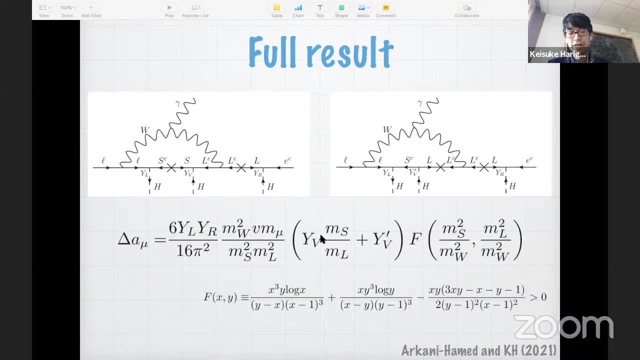 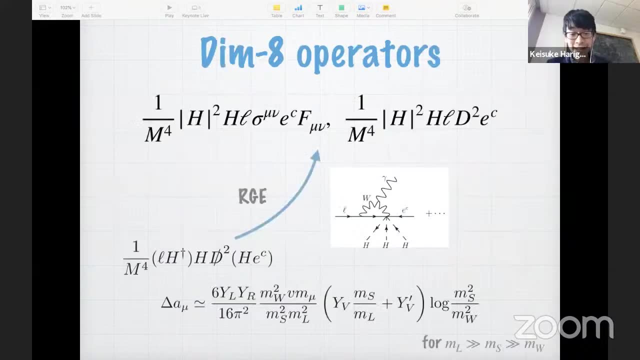 and the correction of the coupling here, here, here, but I'm sorry to interrupt, but mu is the first power. Sorry, mu is Is the first power, or it could not be A fifth? Ah, because you are saying that this V multiplied by mu, it should be mu squared. 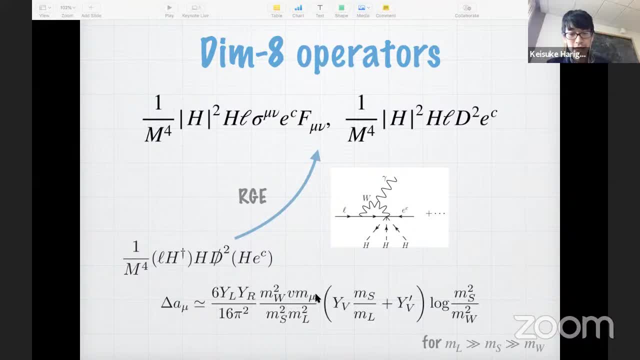 V times mu. So this mu just does not come from the coefficient of the operator, but just comes from the conversion of the dimension of six or five operators to mu. No, in no calculation you will get a mu in the odd power. This is just technically wrong. 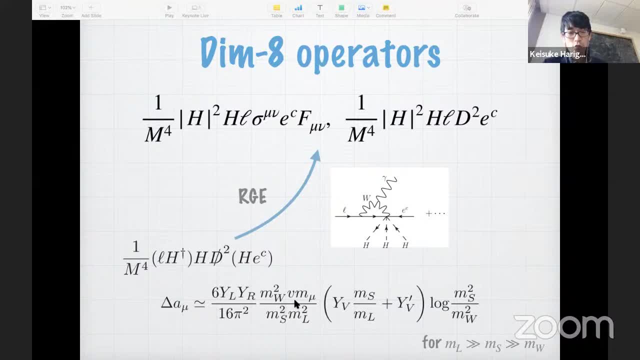 Sorry, mu fourth. Did you say mu fourth? It should be not V multiplied by mu, it should be mu squared, Actually, so that extra power of mu is hidden in here. Where This YL YR? Oh, no, not to. 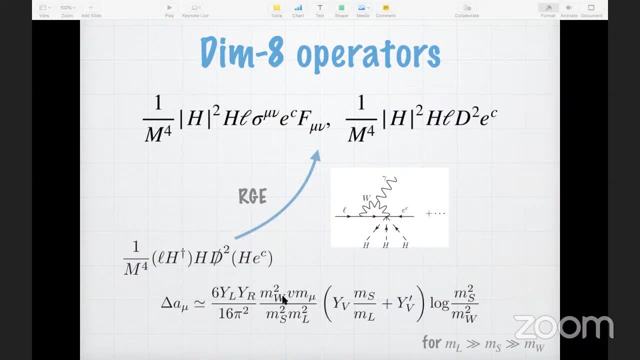 No, no, no, Why. Okay. So here, this mu just simply comes from that. Okay, so if we express this, this YL YR times YV, in terms of the quantum correction, it should be mu squared. 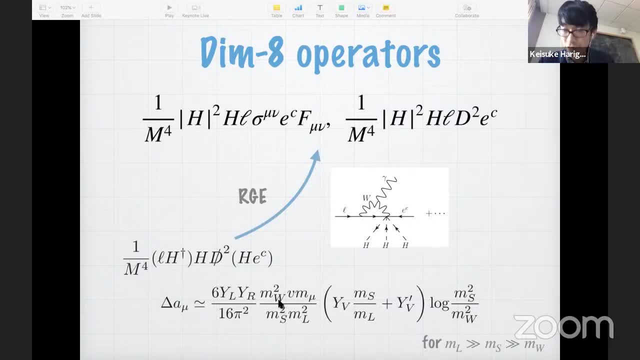 Okay, Okay. So this is a correction to the mu of mass. Yes, we have mu times, delta mu. Yeah, yeah, yeah, Right, but then you see, it's much better to write it explicitly as a mu squared right. 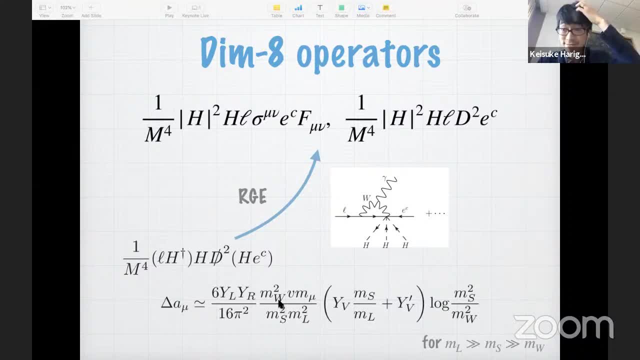 Mm-hmm. M mu times delta mu. yeah, yeah, yeah. Correction to the mu of mass: No, no. correction to mass is one story. Correction to delta mu is a mu squared because in definition it was one over a mu when you defined what is a mu, remember. 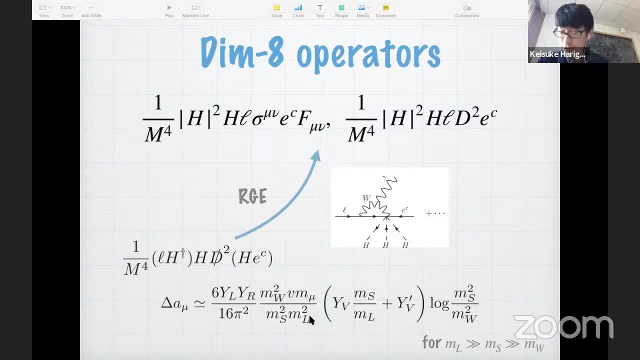 Oh yeah, that definition explains this: M mu, yeah, yeah. So then here I didn't express YR times YV in terms of delta mu. Yeah, This is actually. this can be expressed as M mu times delta M mu, and delta mu may be much smaller than actual M mu. Yeah, yeah, I agree. 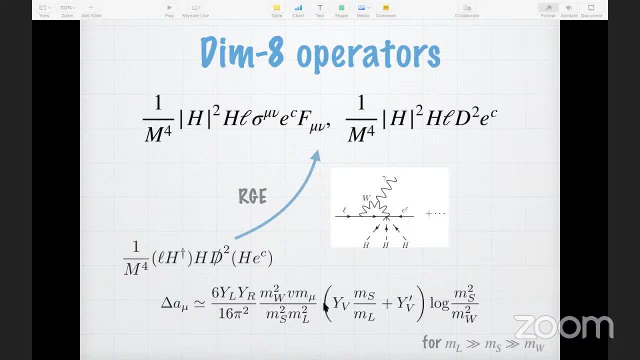 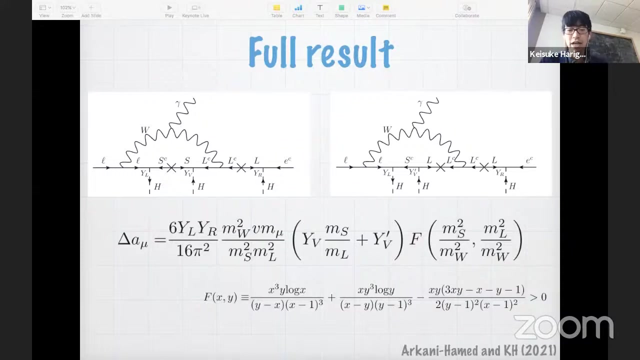 yeah, And also both operators are again the same operator. actually, Mm-hmm, mm-hmm, From B upon D minus 2, what physically happens? yeah, yeah, yeah, Mm-hmm, Mm-hmm, mm-hmm, Okay, And this is the result. And since this is dimension 8 operator, this: 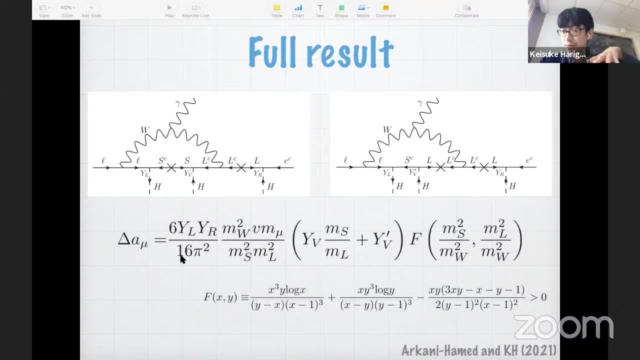 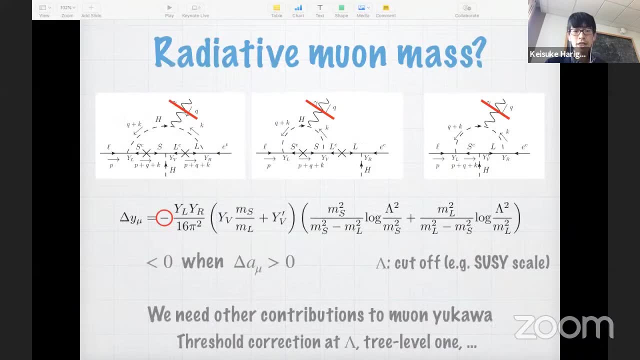 is fourth: power of new physics: mass scale. Okay, And this is the signal that appears in the in the downstairs. Okay, Ooh, So since now we, let me just pause few minutes to comment on the quantum correction to the mu of mass. 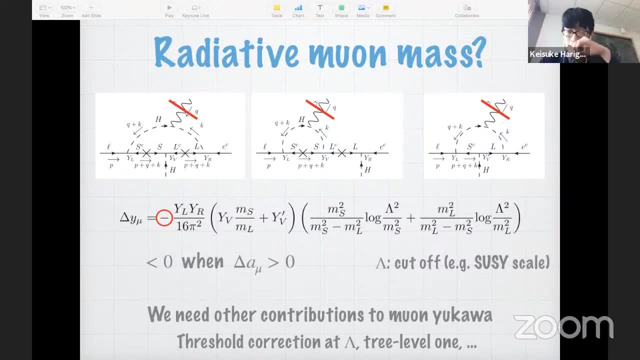 as we discussed, if just eliminate photon from these diagrams, so that the naive correction to the G mass, we obtain actually quantum correction to the, to the mu of mass. So then this is our formula. Okay, you can see this negative sign here. 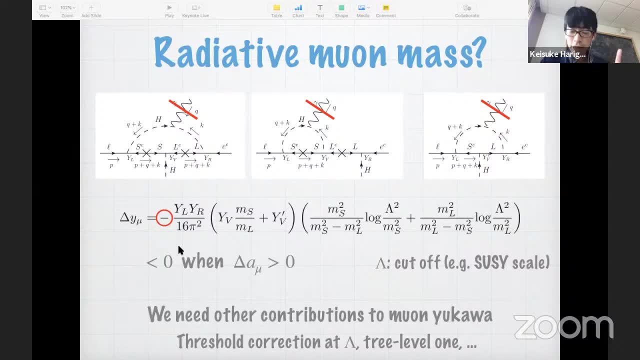 So if we explain the deviation of the G-mass from the standard model prediction, this correction to the G-mass must be positive. So if we choose the sign of the coupling so that the correction is positive, it turns out the quantum correction to the mu mass is negative. 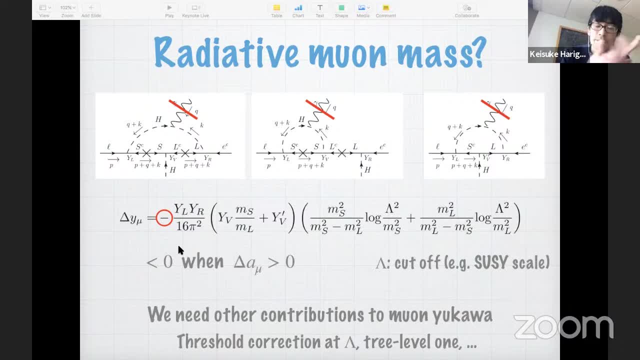 So this means that if we obtain the mu mass sorry from this quantum correction, so we obtain the wrong sign of the quantum correction to the mu on G-mass too. So we must have an extra contribution to the mu mass in addition to this quantum correction. unfortunately, 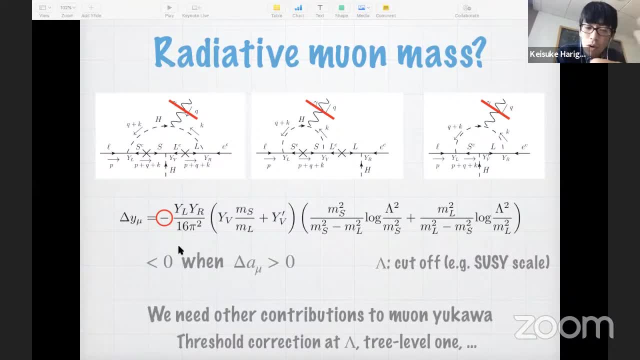 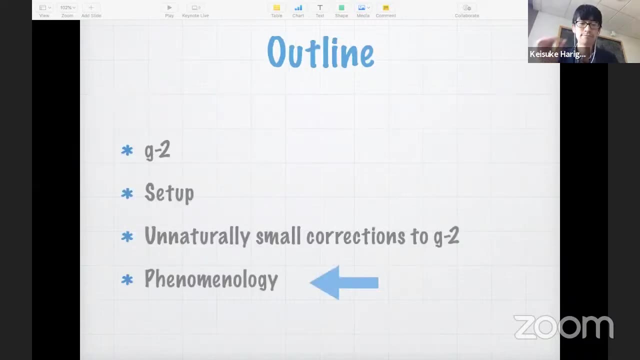 So this might come from just a three-level Euclid coupling or come from some threshold correction at that point. So this is a high-energy scale. Then we can obtain this fully radiatively at this low-energy theory. Okay, so now it's time to 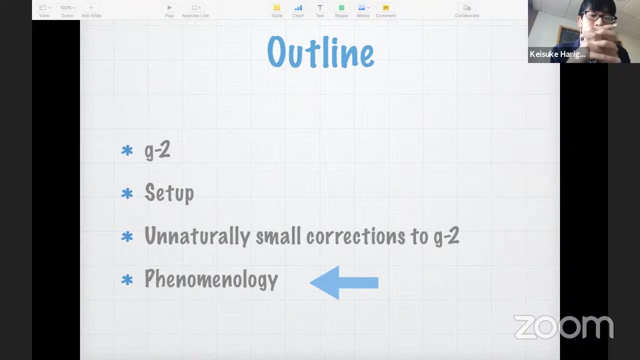 So now, what's the important point is, since the quantum correction of the G-mass is given by dimension eight rather than dimension six operator, the required mass scale of the new particle is smaller than the naive expectation Result. the experiment can more easily prove. 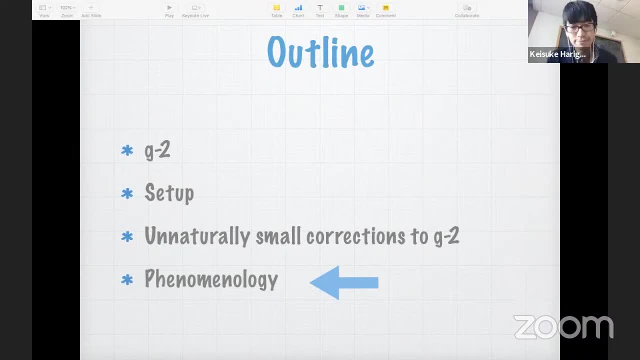 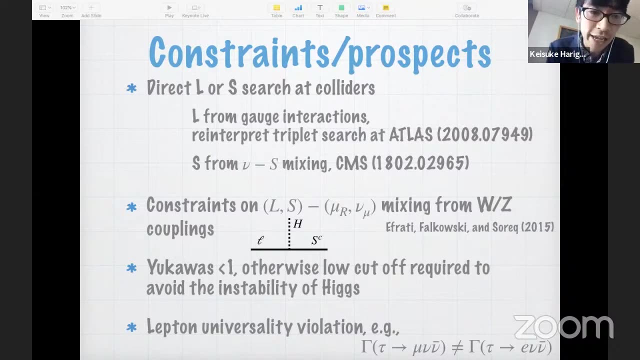 the viable parameters of that theory. So here is a list of the phenomena as you'll be consider. One is the very exciting one: direct production of the new particles at collider, What we call L, that which is the SU to the left. 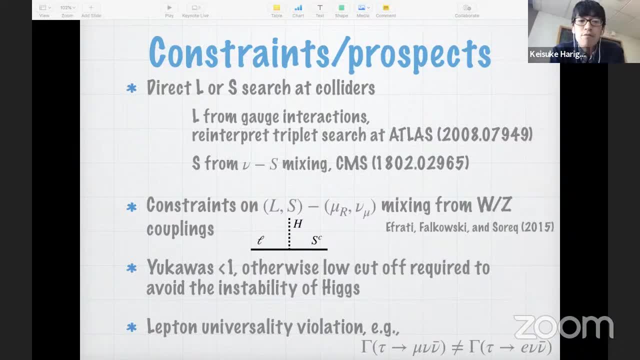 that red electromagnetic weak charge can be produced by gauge interaction. So this is the L-interaction And then the L-interaction. the L-interaction is a very direct interaction at the LSC. So then we use a constraint, We reinterpret the constraint. 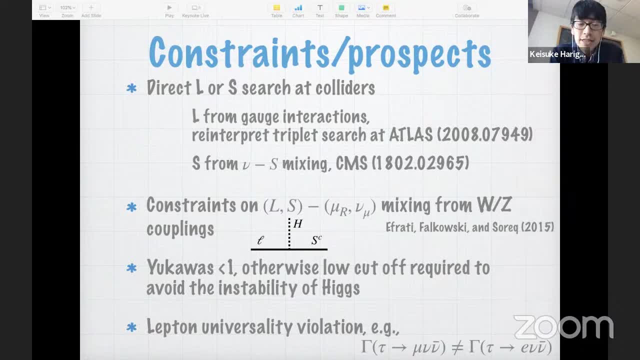 on slightly different model And this singlet does not have, of course, the gate interaction but still have a Euclid coupling with the standard particle, So it can be produced via that Euclid interaction. This is a very direct constraint or prospect. 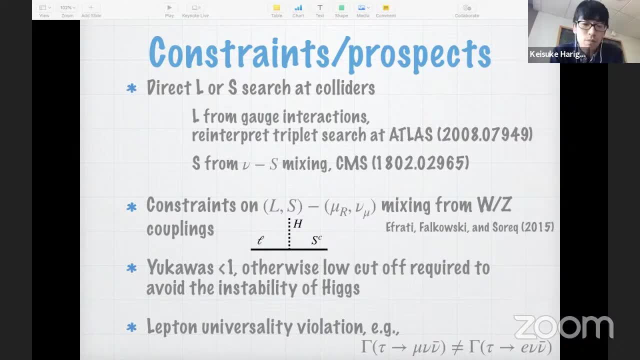 So then we also have some indirect constraint or prospects. So, because you know we have a very direct constraint, we can also give a picture of the initial Euclid interaction on the Euclid particle, And this is a very, very direct constraint on the Euclid particle. 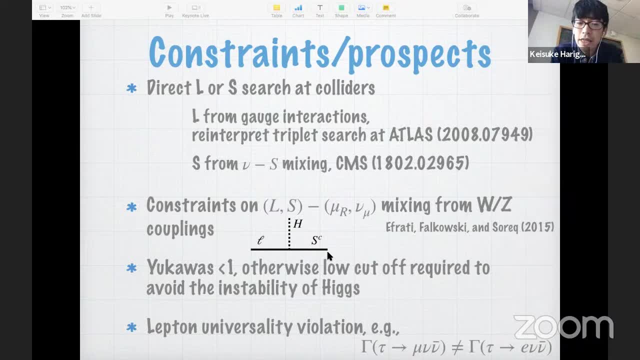 But this is a very direct constraint. So actually you can actually see that that is pretty direct constraint, So we don't have to move on. but this is what we can do here, So can I show something? So now we want to do the very, very direct constraint. 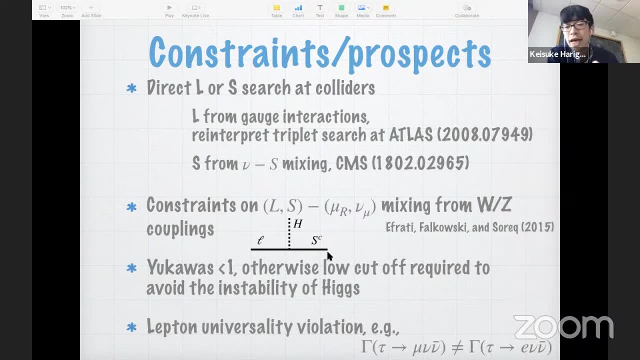 in the Euclid, as you can see here. So let's draw a graph, So let's do so that you can see here It is marked on the euclid. You can see that. you can see that because of that, the Euclid is very direct constraint. have slightly different property, such as the coupling with the W of Z boson. So this can be constrained or detected via precise measurement or the decay pattern of the electric gauge bosons. But at which range you are expecting the mass to be? It is below this 100 GeV before. 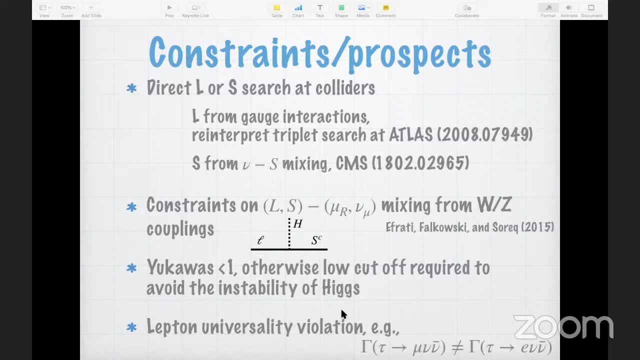 or it's larger than 100 GeV. I mean which direction you go. So heavier direction, heavier than 100 GeV typically. But heavier direction would be enough to give you observable difference for G-2? Because it would be suppressed, right. 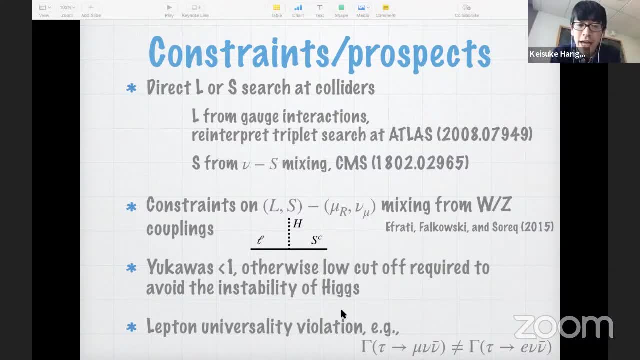 Yeah, but if it is too heavy now we can't explain the muon G-2, unless we take a realistic large UGAC gap-free. So we still have an upper one from the mass scale. So you are talking about 100 GeV or you are talking about 1 GeV. 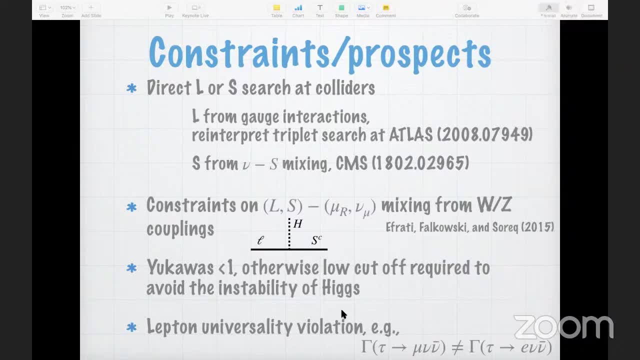 Even higher one. yeah, Higher one, okay, But your dimension 8 operator would be enough to give this for sigma deviation, for this heavier part is what I want. Actually, it is too heavy because of this dimension 8 operator It cannot. So mass is bounded from above to explain the muon G-2.. 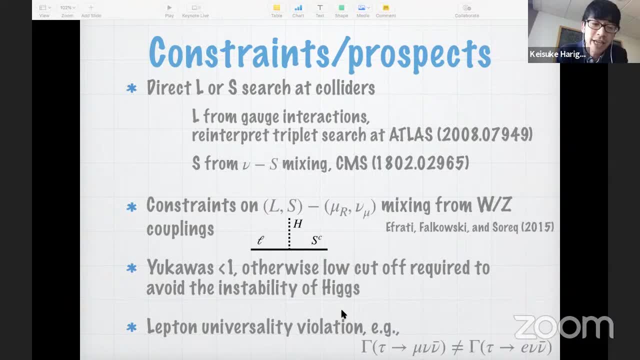 But then since we can't make the mass arbitrarily large, so we have non-trivial constraint, I will show the figure very soon, Okay, Thanks, thanks. And we also require that UGAC gap-free is part of it and is smaller than unity. 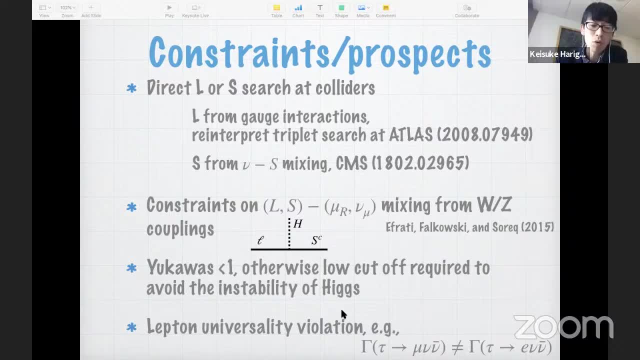 And another phenomenology we consider is so-called lepton universality. So in the standard model the interaction of electron and muon is basically dictated by the gauge interaction. It has universal, gap-free to W boson or Z boson. But once we have this mixing between the 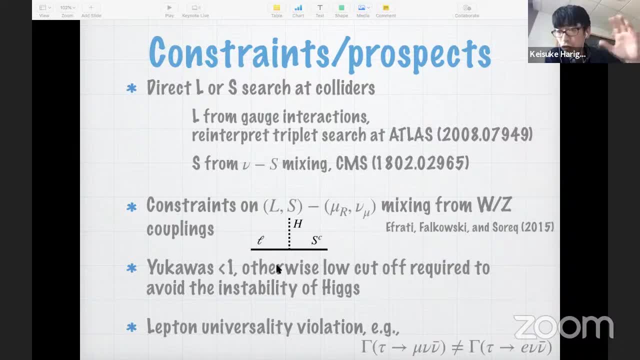 stammered particle and a new particle with different gauge quantum number, so their interaction with gauge boson could be deviated from the prediction of the standard model And in particular, since we only introduce new particle to the muon sector, the interaction of muon with gauge boson in general is different from the interaction of 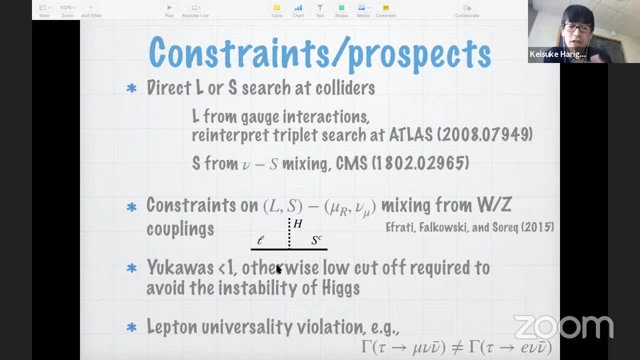 electron with gauge boson. So this is often called the violation of the lepton universality. So, for example, the decay branch of a tau lepton into muon lepton or electron lepton via double boson gate exchange provides important constraints. 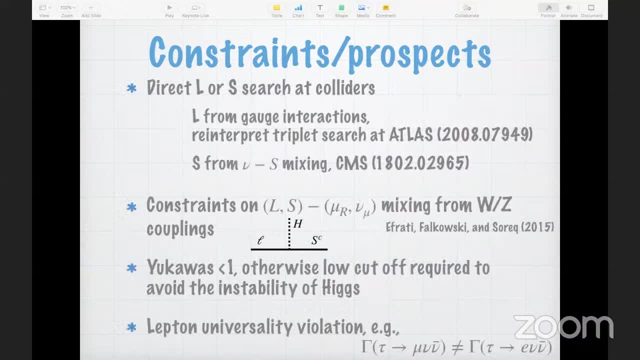 And May I add something Really nice? If you just make sure I really follow The capital, L and S are new fermions, right L and capital A and capital S are new fermions And L is the SU to the left doublet. 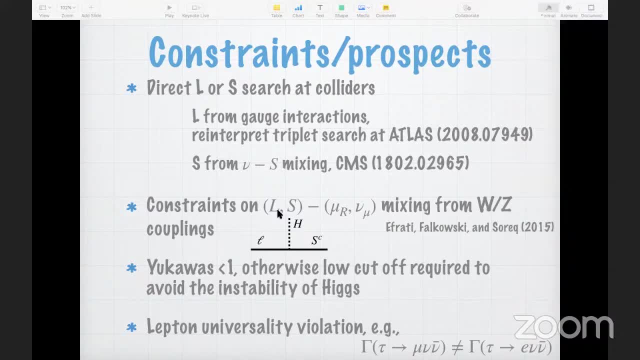 and S is a singlet S, yeah, And they are both new fermions. beyond, Both are new fermions, That's no problem, Just make sure whether they are. How do they satisfy, for example, like anomaly cancellation constraint? Ah, so 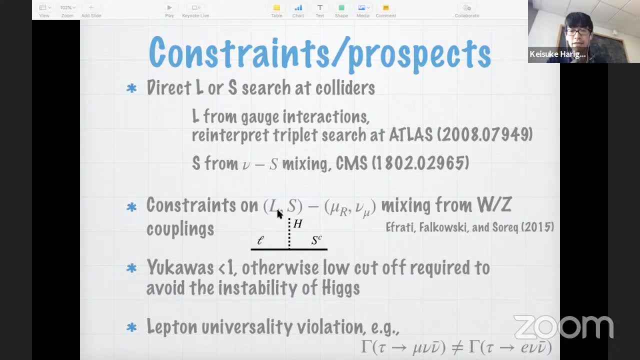 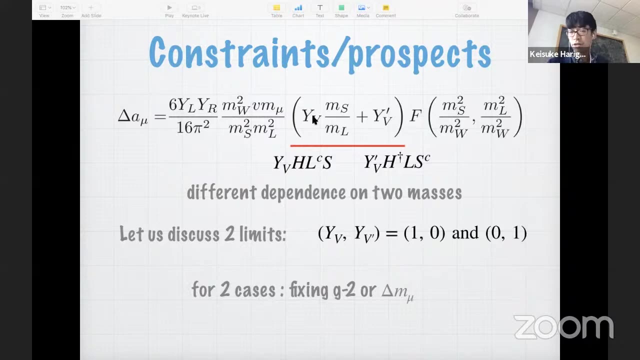 Since we just introduced Dirac particles anomaly cancellation is trivially satisfied. Okay, Yeah, No problem, Thank you, thank you, And the model has a few parameters. So especially the form of the quantum correction depends on if we use this Yukawa gap frame, which we provide with a different set of Yukawa gap frames. 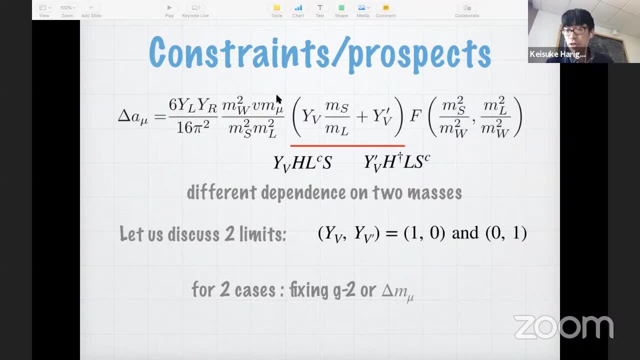 And they have different dependence. Then the quantum correction to the GMAS. it has a different dependence on two masses. So we will discuss two extreme case where one is one and another is zero, and one is zero and another is one. So we also consider the two fixing of the parameter. One. we fix the G minus two, Two. 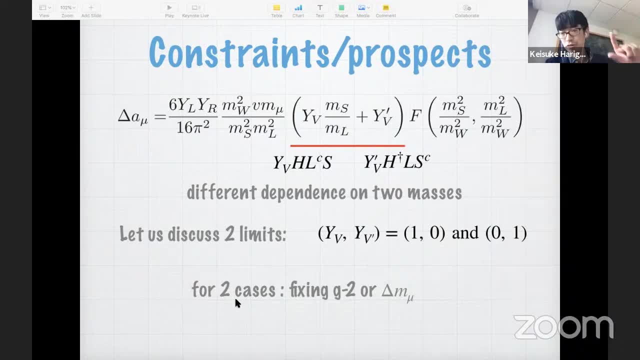 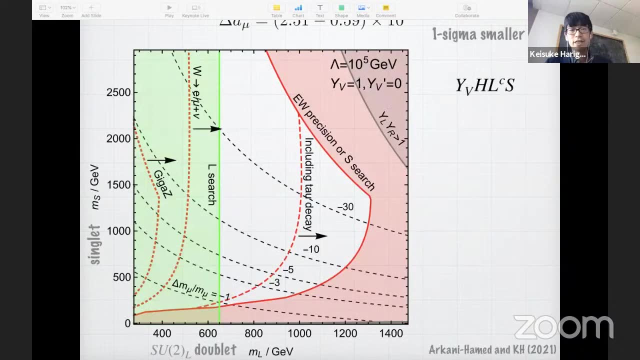 we fix the quantum parameter so that the quantum correction to the mu mass is fixed. So I in total show four parameters. So here is a pro a case where we put one of the Yukawa gap frame to be one, another to be zero. 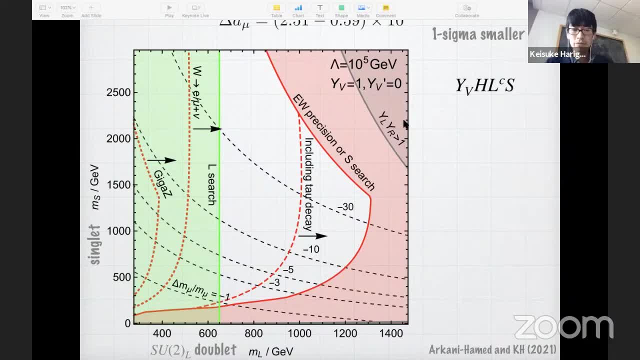 and require that the mu is explained within one sigma. So we fix on each point in this plane, we fix the coupling so that mu is explained. So then, after that requirement, this red shaded region is excluded by the precise measurements of the W and Z boson decays. 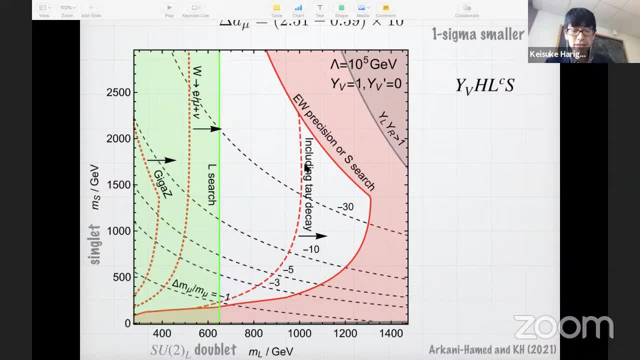 And to the right of this dashed line is excluded by the decay of the tau boson Lefton. universality constraint from the decay of the tau lefton. So you may naively think that since we consider new physics, low mass should be excluded. But here 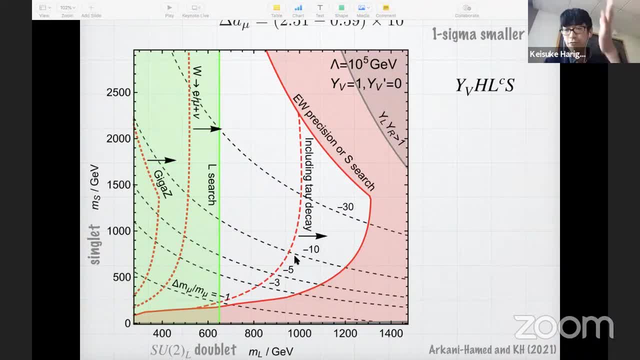 the reason why high mass should be excluded is because the low mass should be excluded from the decays. So the relation between the twoatzis is excluded here just because we fixed the parameter so that the mu G minus two is explained. So what happens is when we take the higher mass scale, 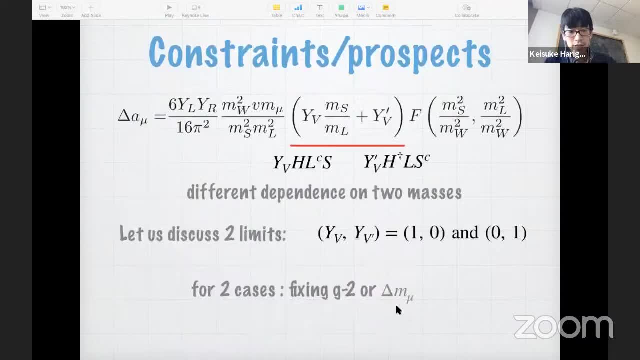 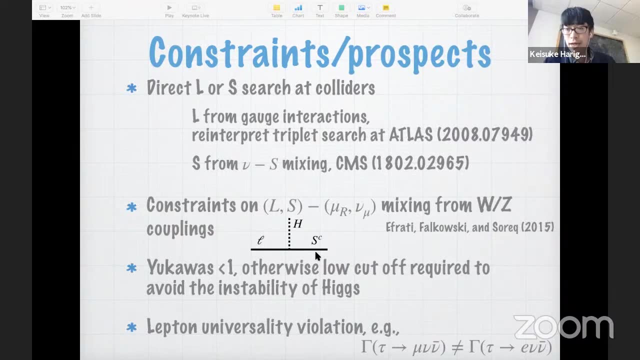 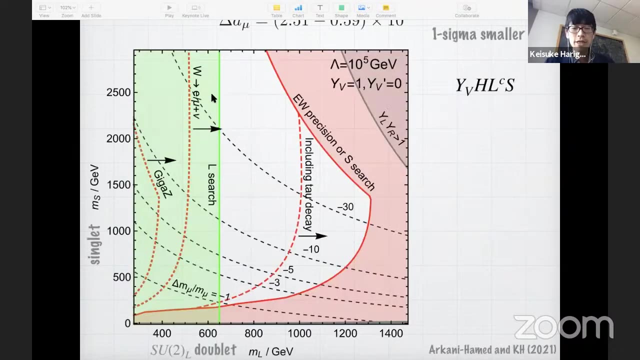 we need a larger coupling so that the mixing between the standard lefton and the new lefton becomes actually larger and the constraint from the W and Z integration becomes stronger. And this green shaded region is just excluded between the twoatzis and the new leftons. And so we 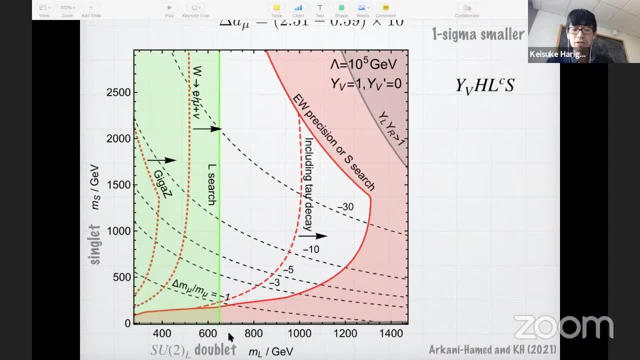 excluded by the direct search of the SU2 doublet L And if we have some future collider such as an international linear collider to the right of this vertical dotted line can be probed If we can produce 10 to nine of Z bosons in future collider. 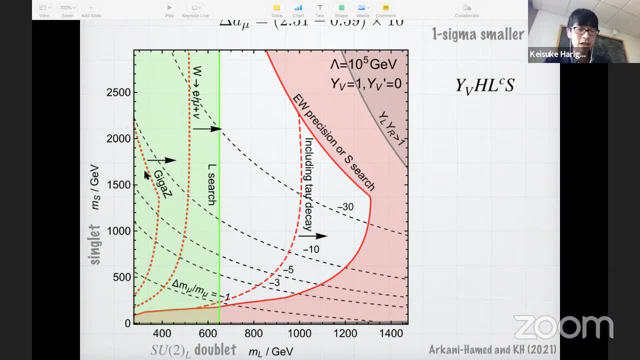 to the right of the second dashed line, which is labeled as giga Z, can be probed And this contour showed the contour of the quantum correction to the mu mass. So, for example, on the line minus 30, the quantum correction to the mu mass from this theory. 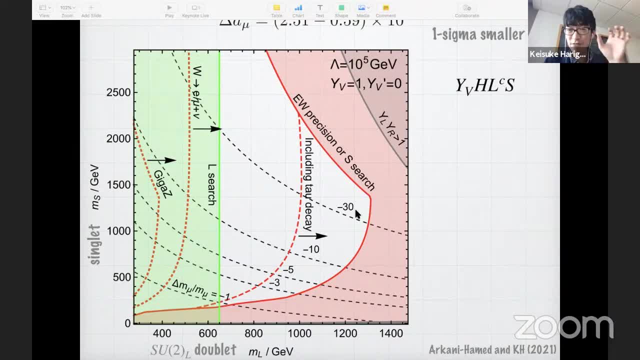 is minus 30 times the observed one. So we need a fine tuning like 31 minus 30 equal one. So this basically show the degree of the fine tuning In the model. So we should look at the region where this number is small. 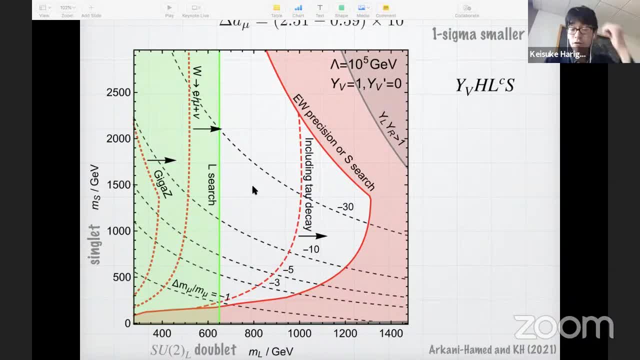 Now you can see that all variable parameter region can be probed by the future colliders. I'm not sure you are talking about correction to the mu and mass. Mu and mass, yeah, But mu and mass, I believe in your formula. 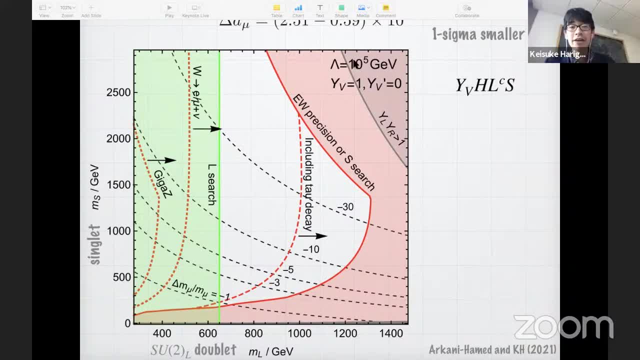 you are divergent, right Corrections? Ah yeah, So here I fixed the cut-off scale lambda to be some value. All right, but, but, but, but. but, look it's. it's a bit re-fixing, right. 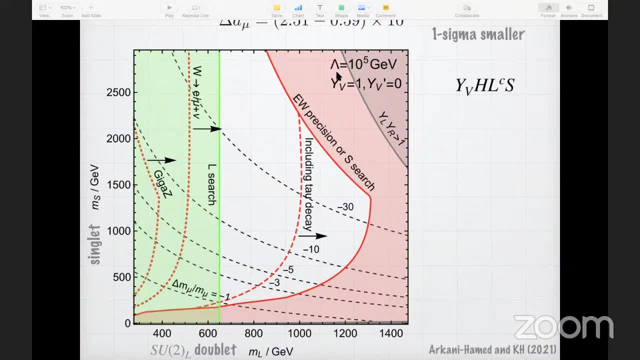 How do you know? Because you know that, strictly speaking, mu and mass it's a physical input, right? It's not comfortable, right? I mean, this is where put in some parameter. of course you can put some parameter. 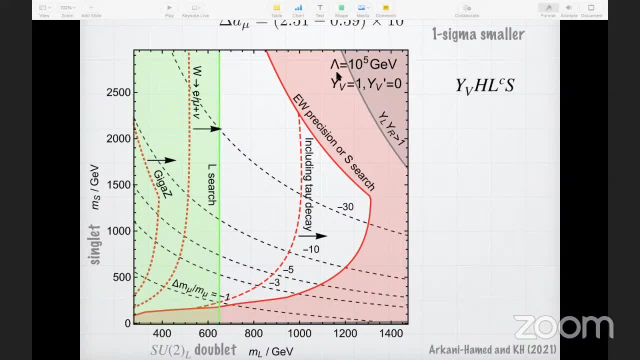 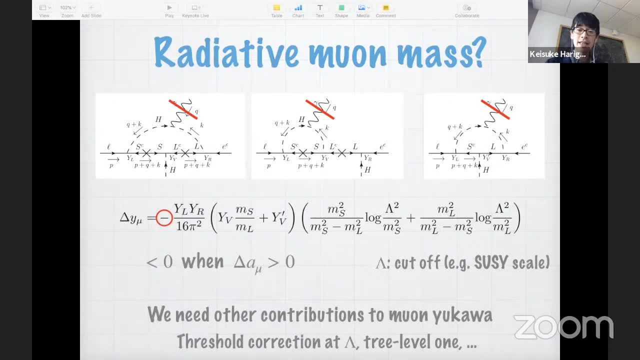 I mean, it's a radical division. It's not observable effect by itself. Yes, I imagine that we actually have some physics new. another new physics is, at this cut of scale, lambda. So this is a finite correction. Still, the dominant correction should come from this: 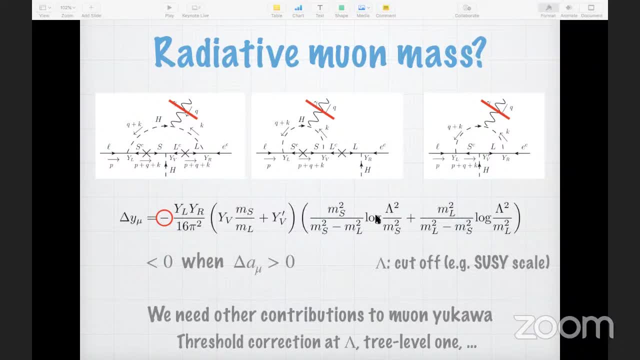 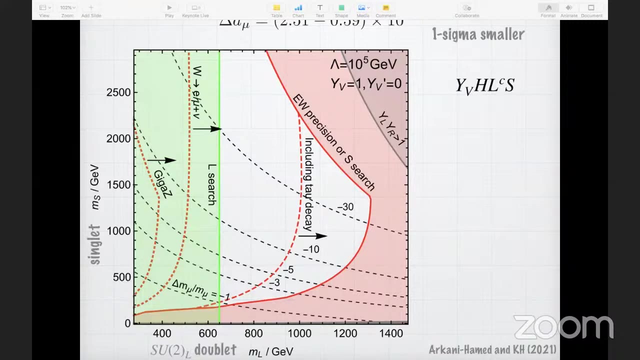 higher log running. I agree. but look your theory. even without introducing this additional physics, at 10 to the fifth JV, it is fully the theory. is UV complete right? You do not need to know. of course, it does contain necessity. 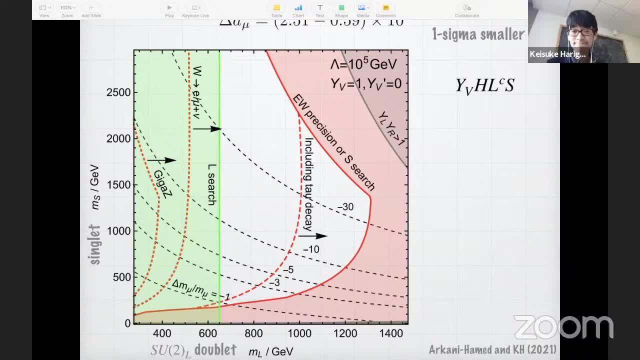 to introduce some physical input. right, But in this way you are defining your cutoff by measuring mass of neuron. Why it's no? I think that it is a little bit unphysical at the moment, Of course, if you would have real particles there. 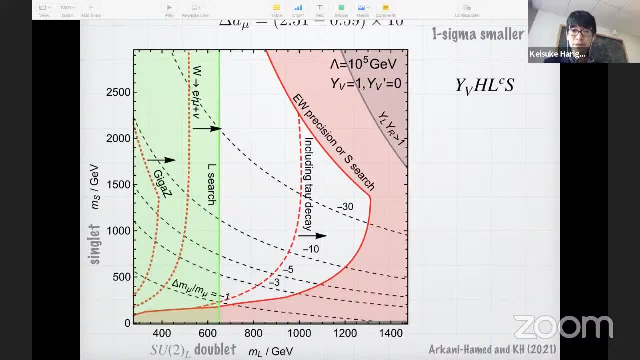 I would agree. right, I mean about there, because then you indeed can differentiate, but it is not in your theory, Not in our theory, but still we have this IR effect theory or our theory, we have this log divergence. 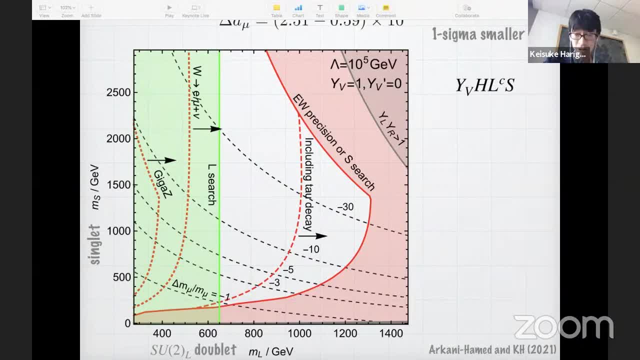 So, in other words, which could be understood by just log running. So I think it's fair to just show the compatibility with the possible UV theory, so that what could be the ultimate fine tuning in the model if we embed a theory into some. 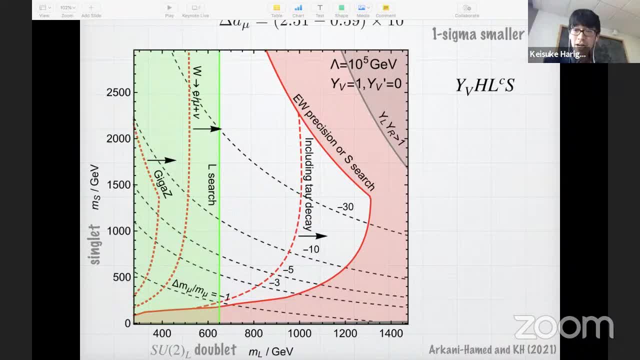 with a theory to a theory with cutoff scale, that cutoff then correct, And then we canVER to the mu mass, So anyway. so that's why I didn't show this Shade, that the region with high fine tuning, because, yeah, it is not clear. 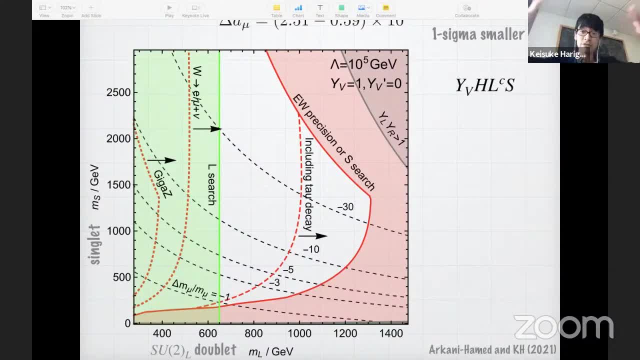 Is it really obscured or not? It is to only show that compatibility is a UV theory. yeah, So we should actually look at that. I agree, We should actually look at this red line and green line to to to definitely probe the theory. 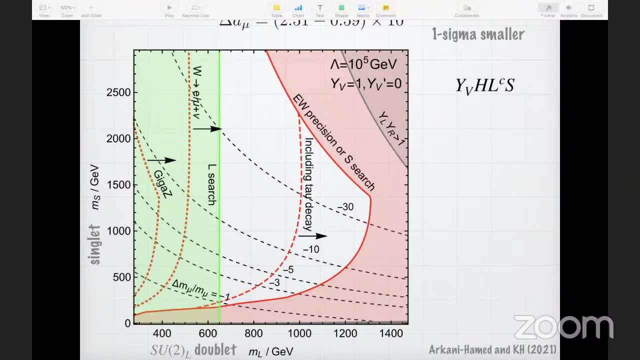 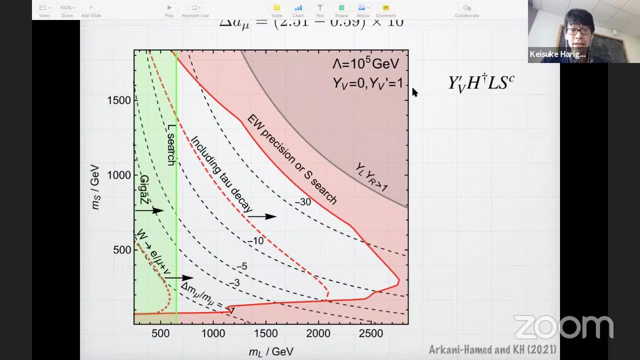 Yeah, Okay. so here is another set of cut-frames, so I just switch off the original cut-frame and just switch on this cut-frame. By the way, Keisuke, you can use full screen, because part of the slides are blocked on the top. 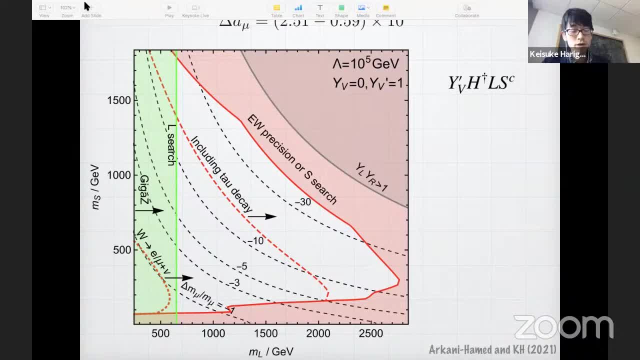 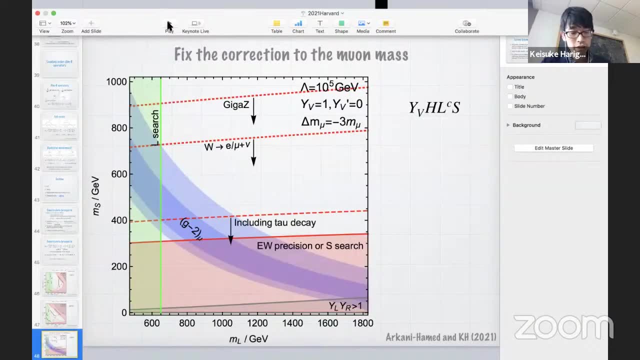 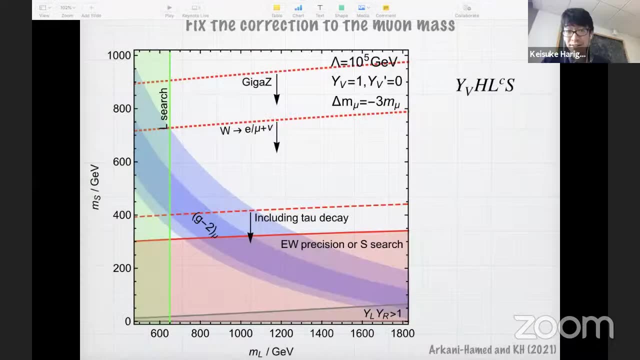 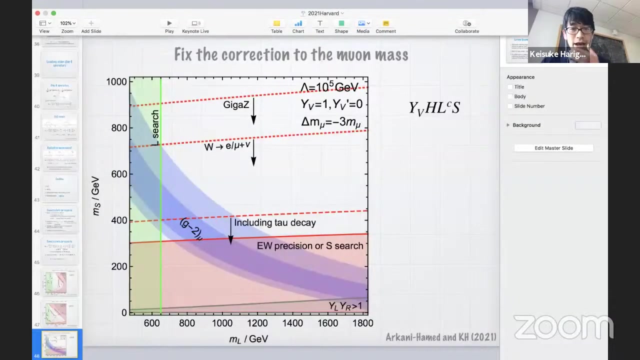 Oh, let's see what's Not a full screen. sharing Like this Full screen, Full screen, let's see. I should. How is it now? Is it still blocked? I used full screen on my side, I see. 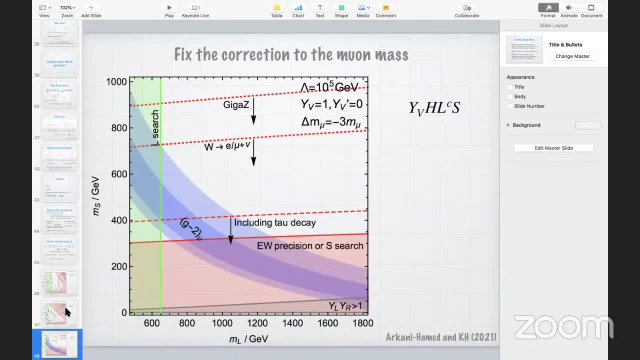 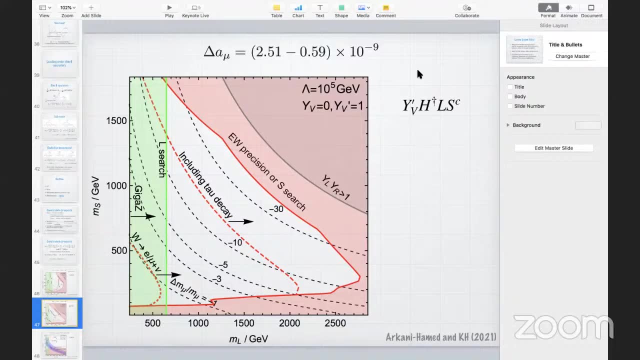 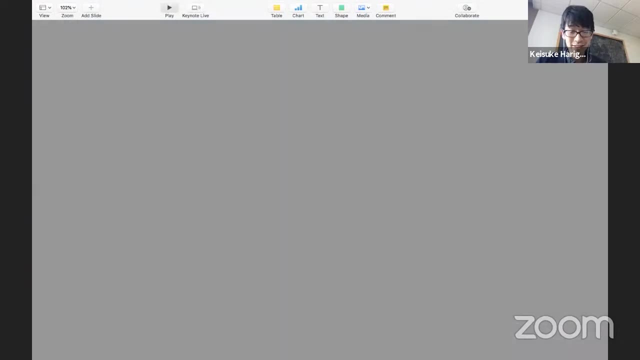 Maybe there should be this green right. There's a green button on the top the left side. Anyway, it doesn't really matter that much, Is that right? Let's see How does this work. now It's bad again. 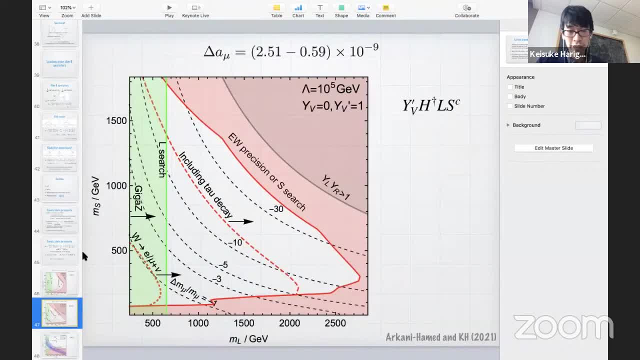 I can use this, then I think every part is now shown. right, Yeah, whatever, yeah, Okay, okay, okay. So here is basically the same figure, but for different cut-frames. You can again show that all parameter regions can be cropped. 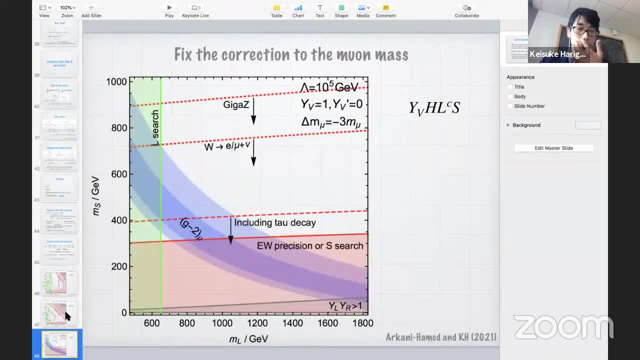 And So here, instead of fixing the muon g-2, so I fix the quantum correction to the muon g-2 while fixing the cut-off scale of the quantum correction to the muon mass. So then now this blue. 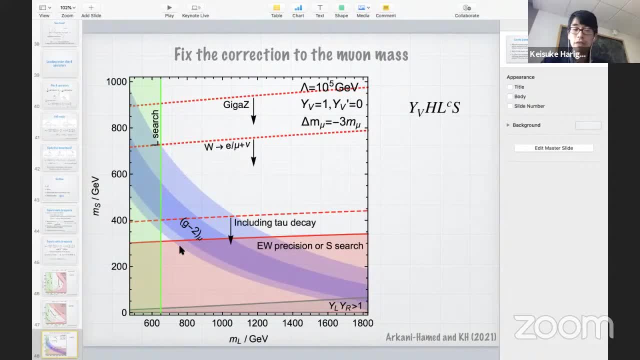 Inside a blue band we can explain the muon g-2.. Again now you can see the thick one shows 1-sigma range and thin one shows the 2-sigma range. Now again you can see that the future machine can probe the all viable parameter space. 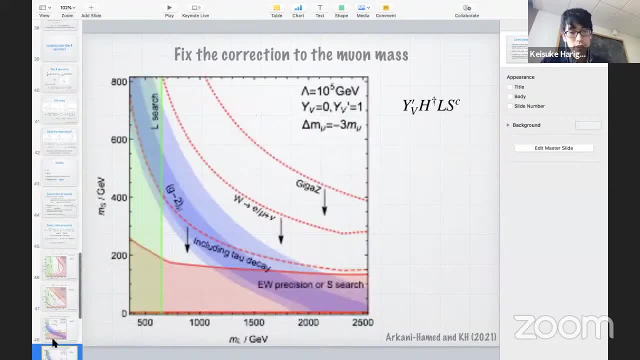 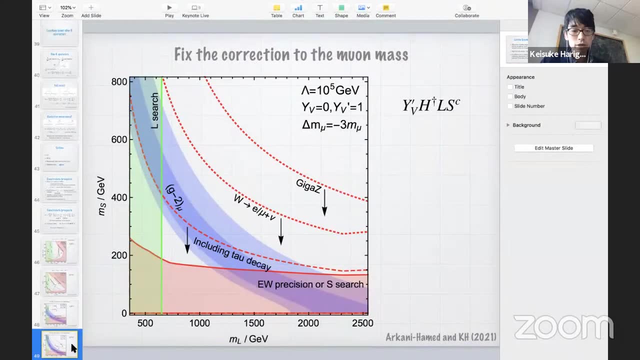 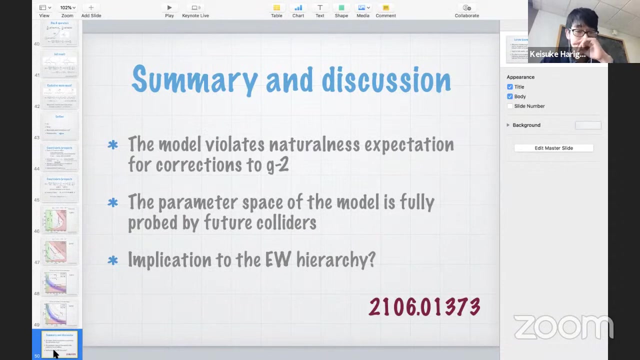 And Yeah, And just yet that's the same one for the different set of the cut-frame. Okay, So let me give summary and give some brief discussion. So this model violates the natural expectation for quantum correction, For quantum correction to the muon g-2.. 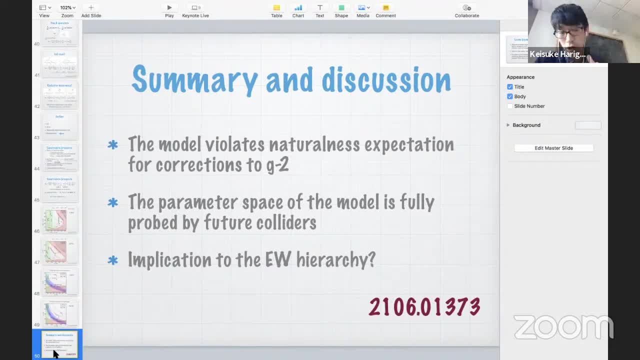 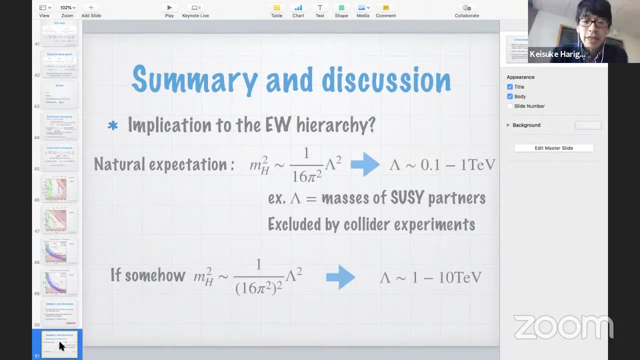 So as a result the required new physics mass scale becomes smaller and the parameter space of the model can be fully probed by future colliders. So this may have some implications to the electric hierarchy. So the natural expectation would be that if there is a new physics with a cut-off, 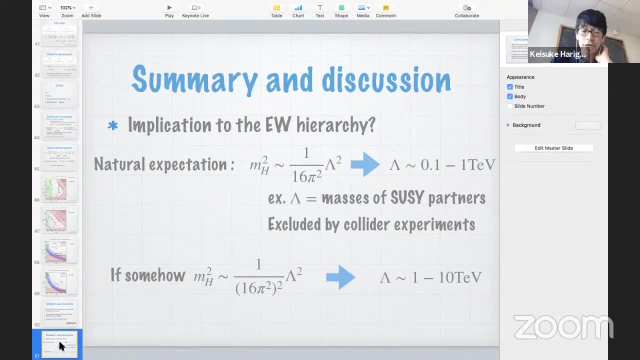 At the cut-off scale lambda, we will have a quantum correction to the Higgs mass as far as the one separation times the cut-off scale. So this cut-off scale is, for example, the masses of superpartners in supersimic theory. 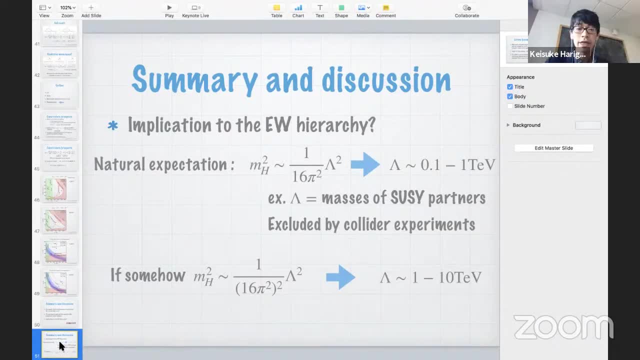 To obtain the observed Higgs mass squared, this cut-off scale must be around the L-cube scale. However, such possibility has been excluded by collider experiments. So if this natural expectation is again wrong and we have extra suppression like the to-do factor, 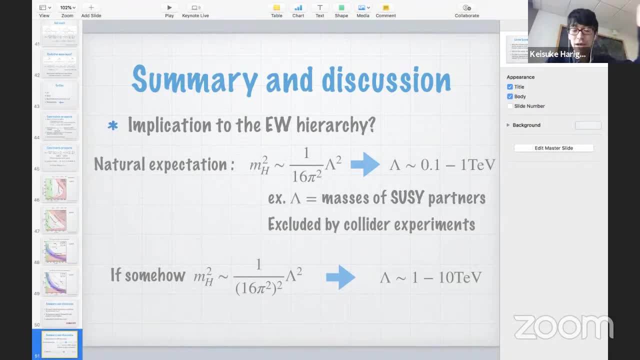 this The masses of new particles could be 10 times larger, say 1 to 10 dB, if it is completely compatible with the collider constraints. So it might be interesting to see if there can be some new physics if the quantum correction to the Higgs mass for the new physics is suppressed. 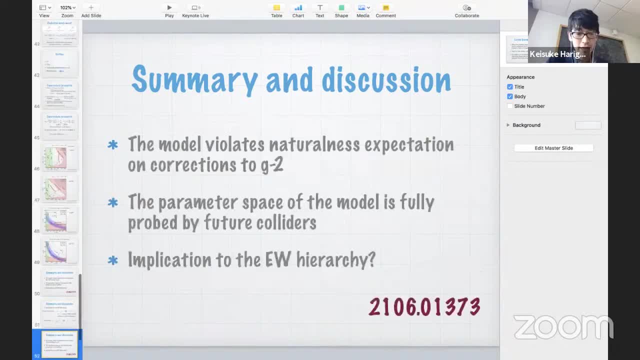 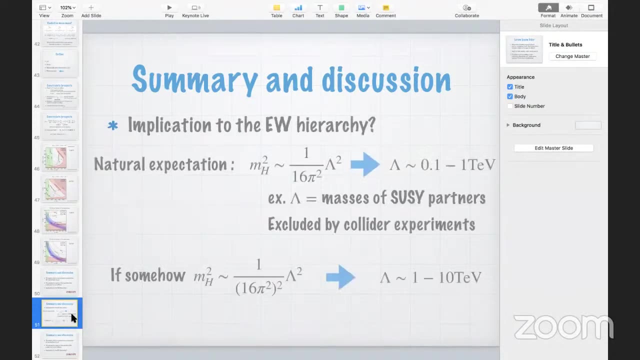 because of this total derivative phenomenon. Okay, that's all, Thank you Of numbers. I'm sorry, just to follow, Remember you estimate a normal correction request for 100 JV right. New particle right, I mean new fermions, say 100 JV. 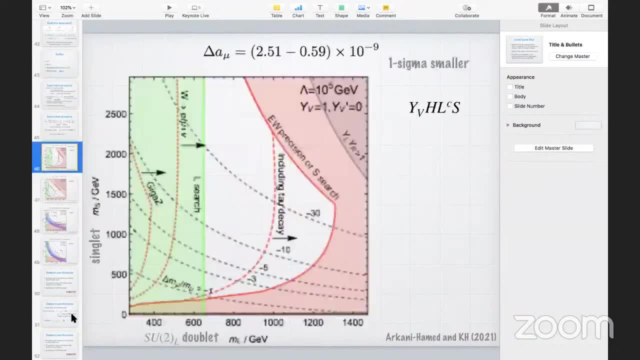 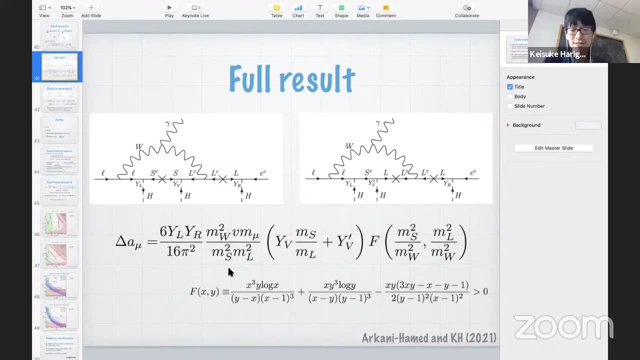 When you are talking about your correction, which has an additional Mw squared divided by Mu squared in addition to what it was right. It looks like you're suppressing correction, right? Okay, so when you're suppressing correction, then your new fermion should be even lighter than 100 JV. 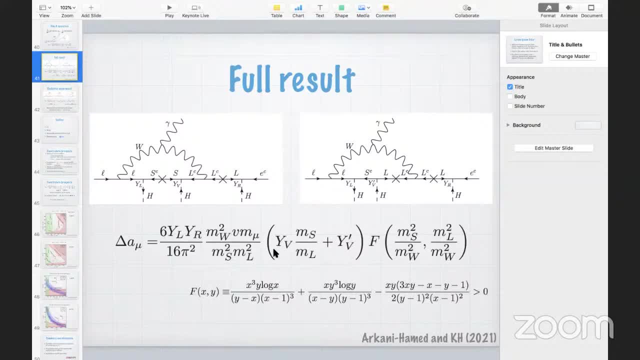 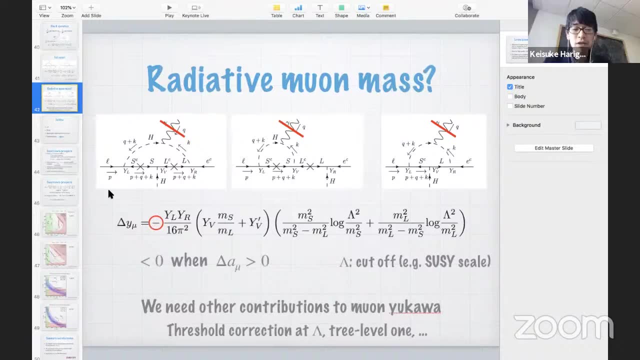 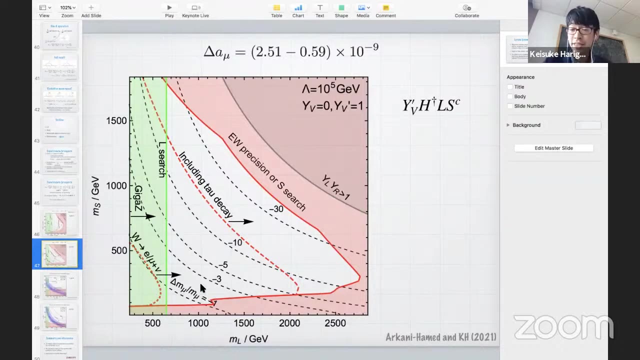 And I'm not sure I follow this particular path. What's happening here is the factor of 6 here, So I allow the quantum correction to the mu mass to be a bit larger than the delta 3.. So essentially, you're saying that numerical coefficient is large, right? 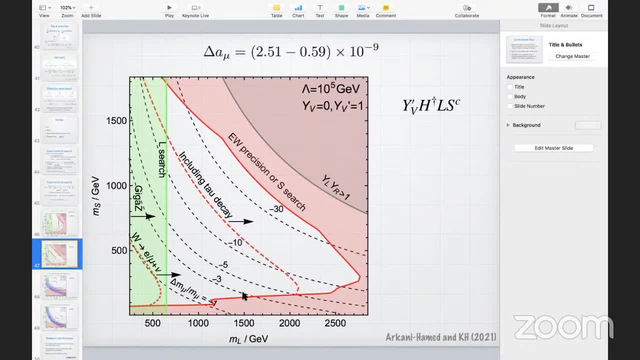 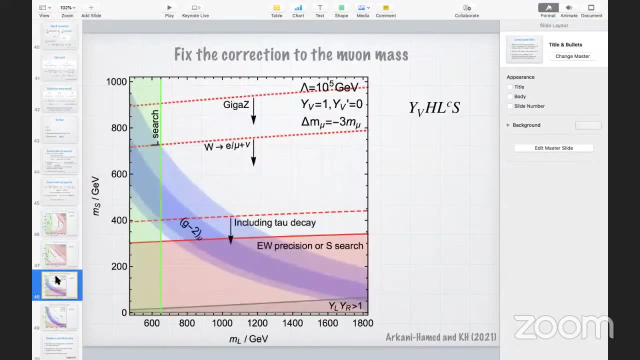 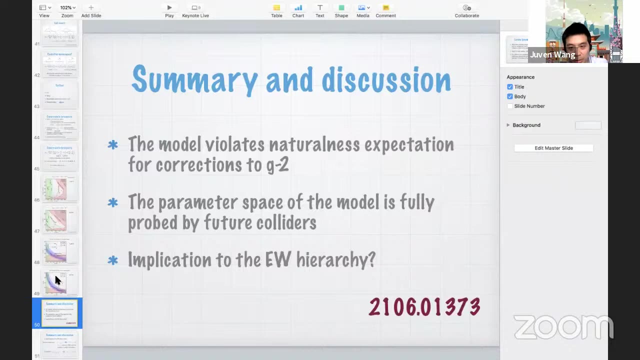 Numerical coefficient. yeah, Yeah, yeah, I see. Okay, okay, Thank you, Thank you. Yeah, yeah, yeah, Yeah. So thank you, Keisuke, for the wonderful lecture. Thank you very much for the wonderful lecture. 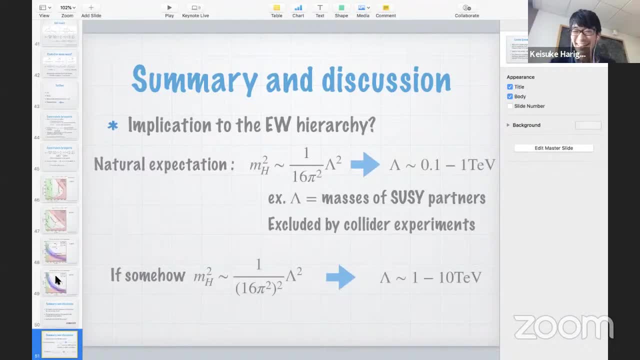 Thank you very much. Any questions from the audience? Gosh, I didn't check chat. Oh, Anything, nothing's important there, Ah, but they say that my mistake in the full screen. Oops Is, Matt has a question. Question about something entirely non-technical. 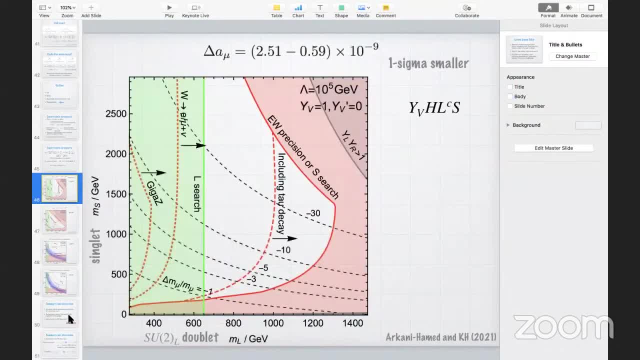 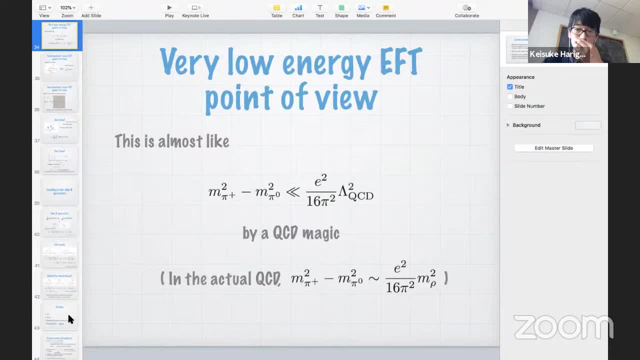 But your reference to QCD and the pion mass splitting, I just didn't understand what you were saying. Yeah, that's what I just wanted to say. Also in the QCD, if you just look at the quantum correct the diagram. 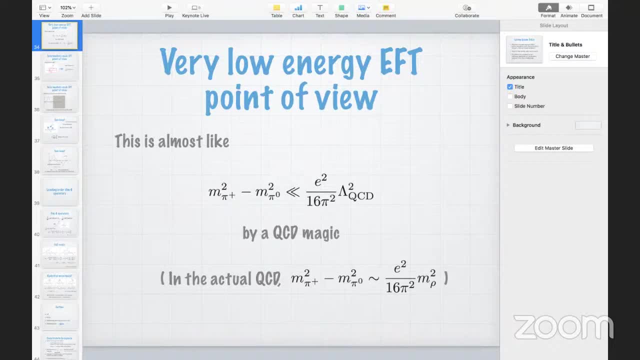 By lambda QCD you mean the cutoff on the effect of Lagrangian. Yeah, yeah, yeah, yeah, Okay, So it's a technical point rather than a numerical point. Yeah, yeah, yeah, Actually, yeah, I just 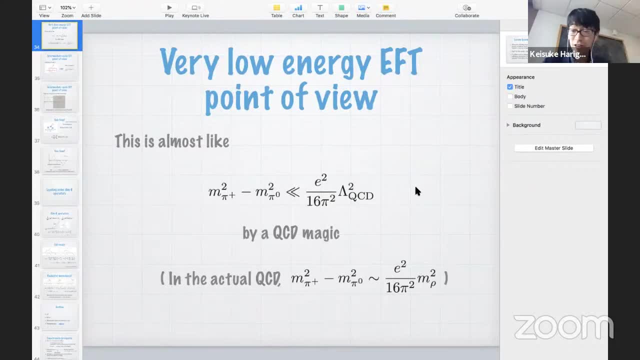 I didn't imagine the exact number. Yeah, just, I mean I mean cutoff. Yeah, Like a Romanian mass or new resonant scale, But when you say that, you're saying that the pion mass, but when you say it is almost like 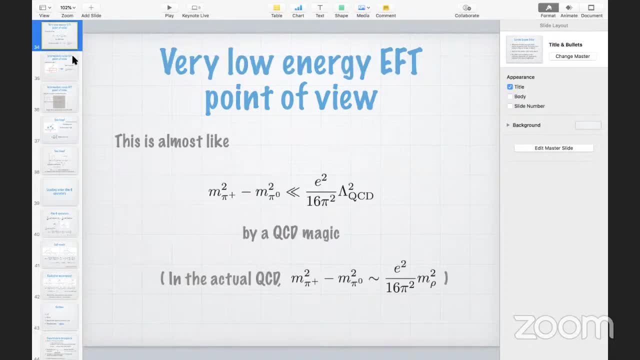 are you saying that in a similar way? there's some cancellation that? What I meant is that this is almost like when we compute the pion mass difference in the QCD-like theory and find that the mass difference is small. Of course this is not happening. 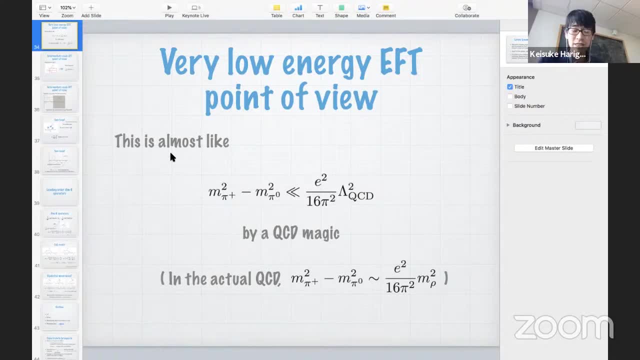 not what's happening in the QCD, But to me it sounds like this. But look M-Rosc, where in QCD is proportional to lambda QCD square. So you're talking about numerical coefficient, right, Because both are relation, are the same relation. 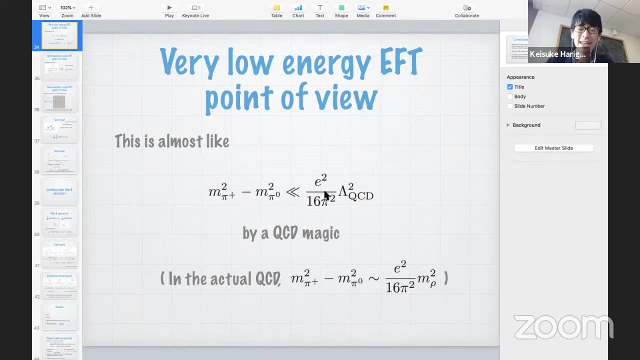 Yeah, yeah, yeah, yeah. What I want to say? this fast equation, of course not what is observed, No, no. But then your point is that mass of rho, which is proportional to lambda QCD, this coefficient is larger than one, right? 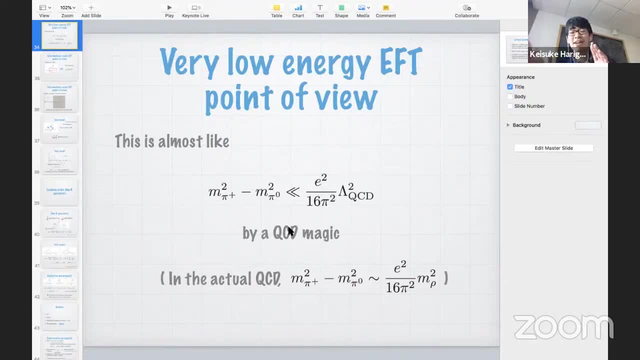 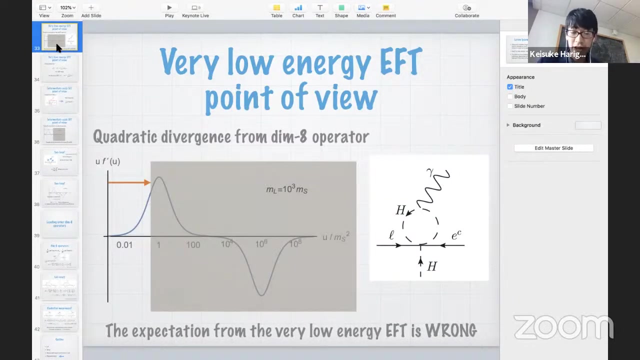 That's it. No, no, no. What I want to say is I didn't argue that this is what happened. The small correction is not what happened in the QCD. I just wanted to say that having this small correction in this theory with vector-like fermion, 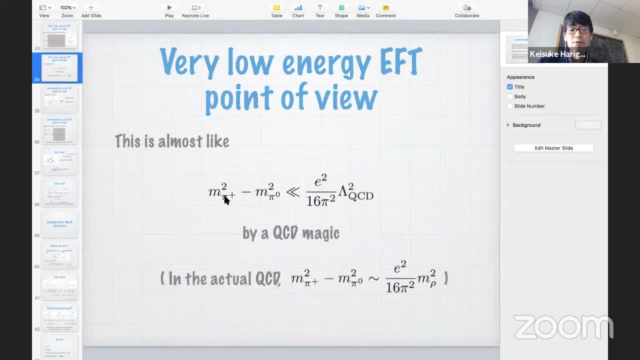 is to me almost like that, the pion mass difference or the pion. it's small. I mean, it's not actually small. I just wanted to say that it's like It's confusing here. I think what you're saying is that the surprise here would be: 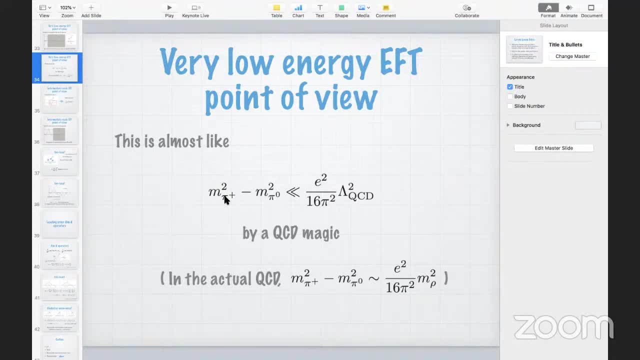 if, in fact, contrary to the fact, If, in fact, yeah, yeah, yeah. If, contrary to the fact, the pion mass putting was even smaller, Yeah, yeah, yeah, yeah, yeah, That would be. 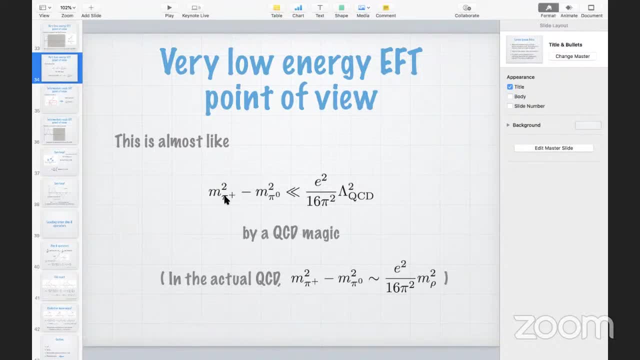 All right, all right, But it is As if yeah, yeah, yeah- You need to rewrite this line so it's a little clearer what you're trying to say- Yeah, as if it were that yeah, yeah, yeah, like that, yeah. 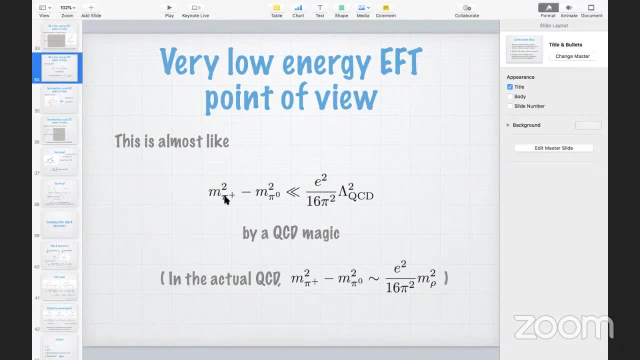 But, Matt, look, I think you would agree that it is just a numerical coefficient. It's a coefficient between MRO and lambda QCD, right? I don't know, I'm not even talking about that. I'm just saying that if we find that, this mass difference, 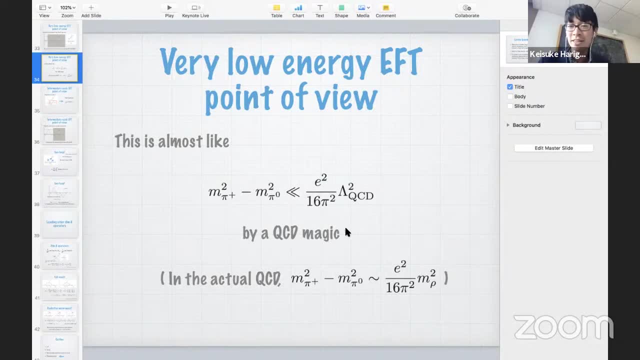 is much, much smaller than this naive expectation in the QCD. we will be surprised, But of course that is not what is happening in the QCD. In other words, Akari, he's saying QCD in the real world. 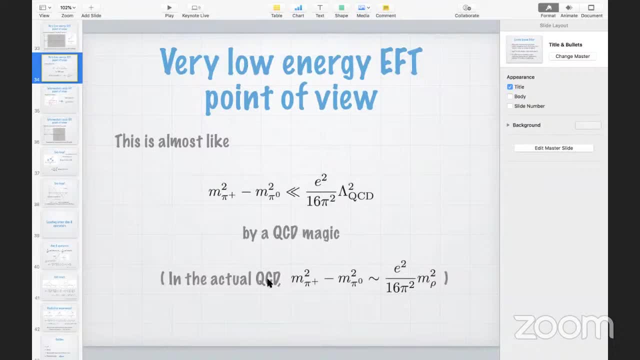 QCD satisfies the expectation that you would naively have. I see, I agree, Yeah, yeah, yeah. As if you went and measured the pie in mass splitting and discovered: Yeah, yeah, yeah, yeah, yeah, yeah, Okay. 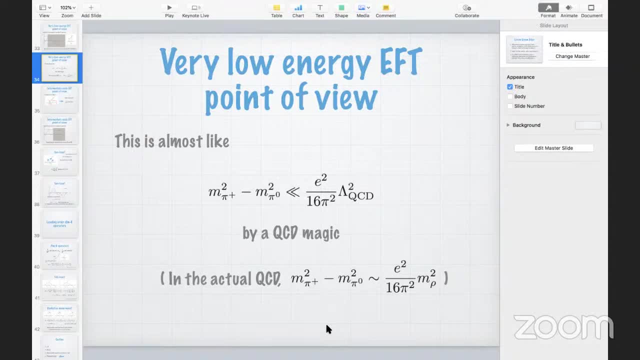 I agree with this interpretation. Yeah, I agree. But look, moreover, say, in QCD some rules, for example, no relation between lambda, QCD and MRO. We are calculating. No, I mean it's. 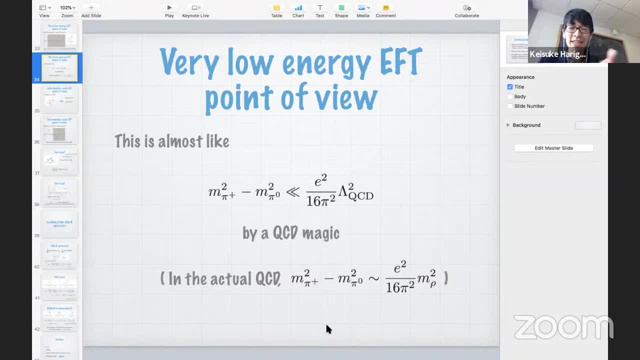 In this lambda. I just mean, that's the new raison, rather than just that dynamic landscape. Yeah, yeah, So I had a question, Keisuke Hi, The place where you were showing the integrand which was canceling between the two contributions. 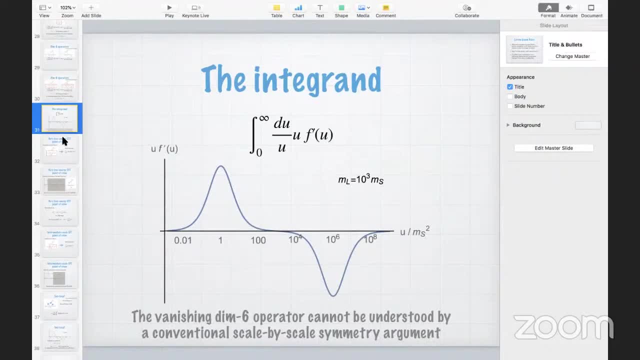 This one Right. So this is from the full UV theory right. Full UV theory Integrand the full UV theory Right. So maybe you said it and I didn't understand. Can you identify what are the features of the UV theory? 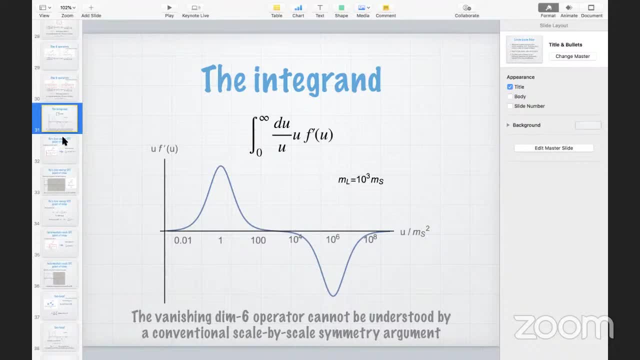 which give rise to such a Strange, surprising fact in the low-energy effective filter. Because this will kind of tell you this naive expectation right, That when you do power counting and you say this is the contribution but it's not correct. 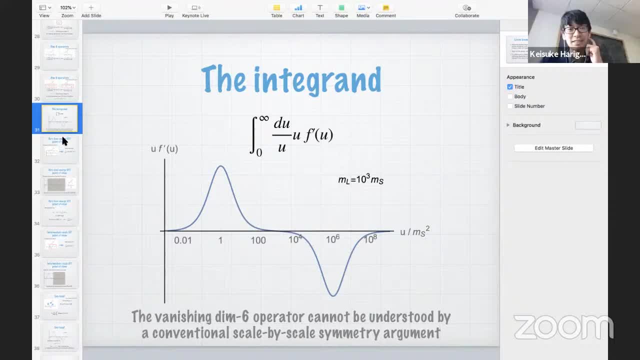 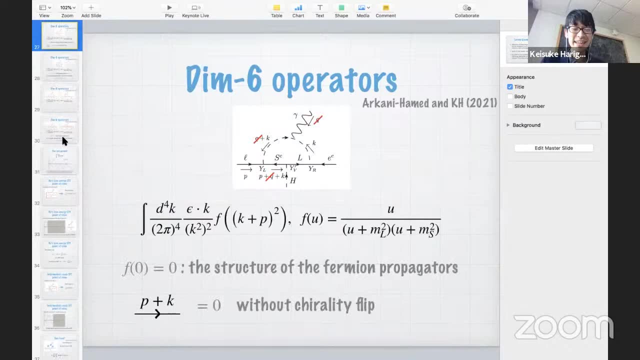 What kind of UV theories will fool you? Is there something you can identify with this toy model? or Ah, generically? Yeah, exactly, Generically. again, if the correction is proportional to the total integration of a total derivative, we will always have these. 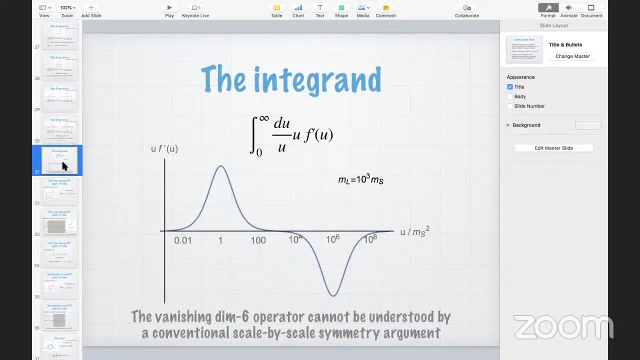 So that is true, but something I mean that's technically true, because that's how you're getting a UV minus IR contribution, And then you also have to have arguments to say why they're both zero right. So you had some parallelity argument. 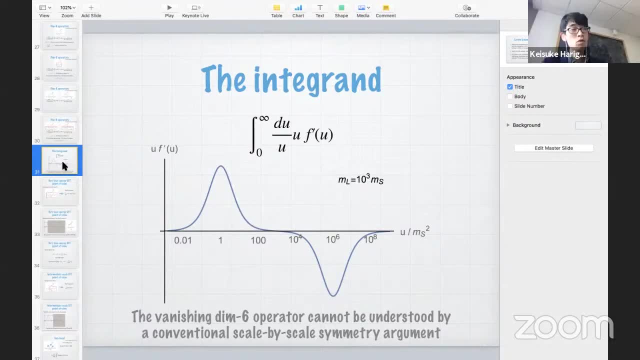 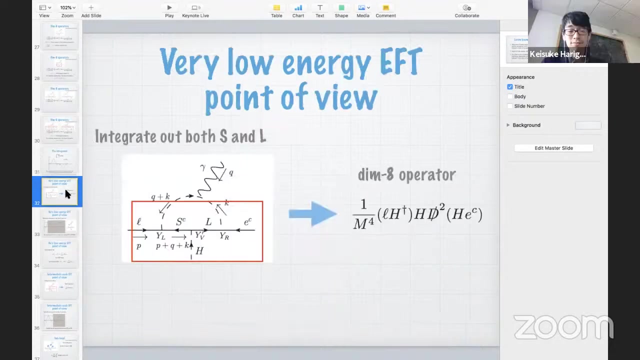 or the structure of the integrand Both zero. Let's see, But it is not that one UV and both UV, Because you call it UV and R. but it is artificial. It's artificial separation of scale. Yeah, yeah, If it's still heavy Fermian scale, right. 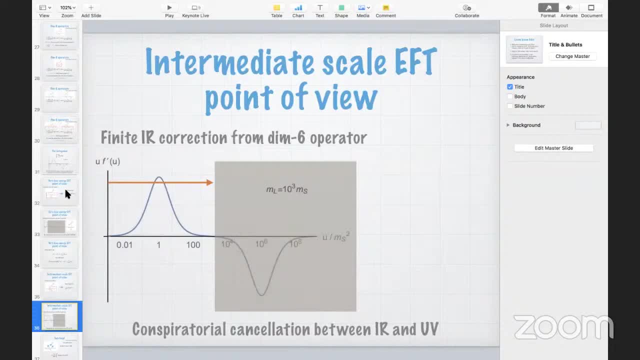 So in this way, it's about how much is UV contribution Mm-hmm? Well, I was referring to the slide where you had F zero and F infinity, And I think you're arguing that one is zero just because two powers in the denominator. 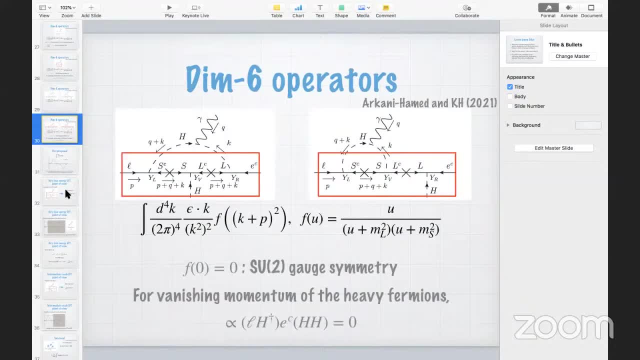 in the function U and the other one was zero because of chirality. right That if you set the momentum to zero, Ah, this is not because of chirality, Because of this identity of SU. Sorry the SU, Yeah, this is not coming from chirality. 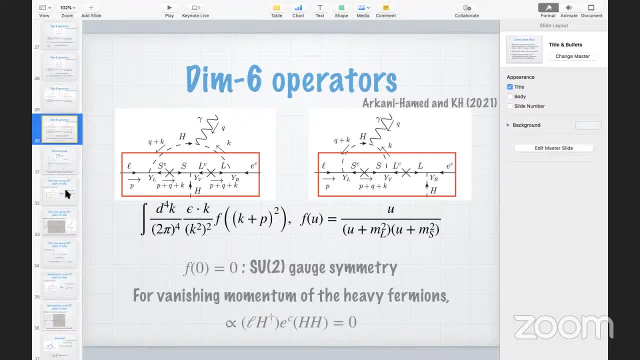 Okay, But the I mean In general. But my general question was the integrand being a total derivative is a bit opaque. Is there something more open that one can think about in these toy models which will Uh-huh? 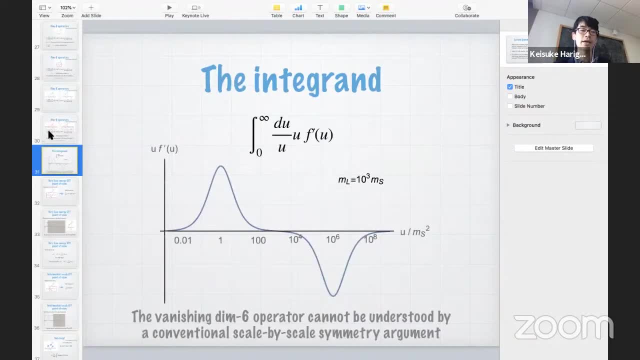 I don't have any idea if you have any other example beyond total derivative. No, Looking at this, it depends which way you're calculating diagram. When the integral is total derivative, you can use a different way of parameterizing momentum, and then this cancellation will be immediate. 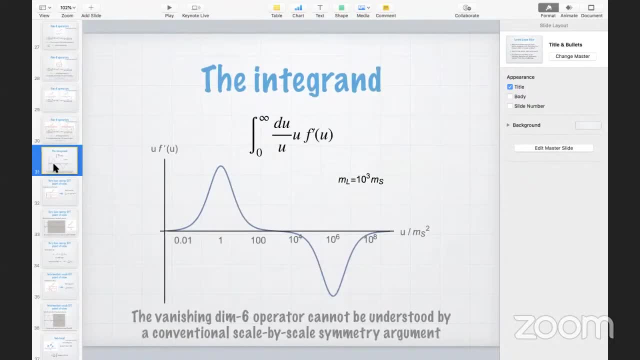 So this kind of technically dependent statement. However, the point itself that it is zero, it would be still true. I mean, what I'm trying to say is that it could be in much simpler way if you will do it a little bit different technically way. 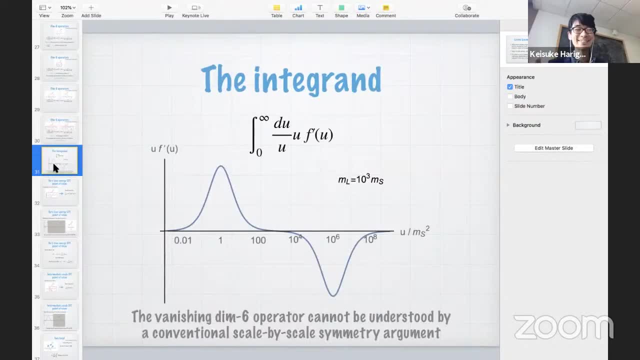 That's what I don't understand. Well, I mean, the integrand isn't physical right And the answer is physical. So you have the potential for moving things around and making the cancellation look different. Yeah, That's what I'm trying to explain. 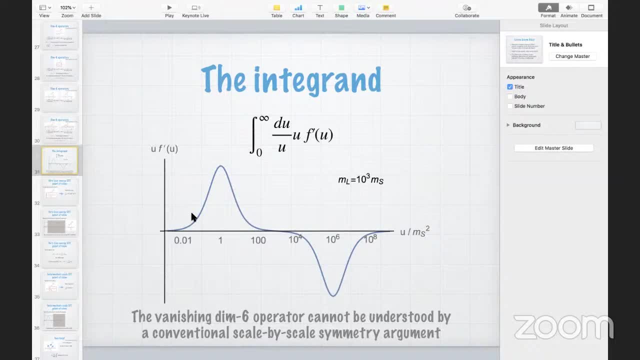 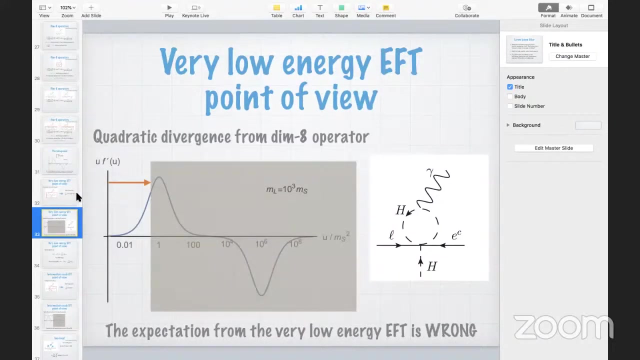 Yeah, I agree, Matt. Yeah, I think the question is well, but if you're a low energy theorist, could you set up the calculation naturally in such a way that something that was obviously zero would instead start looking quadratically divergent? 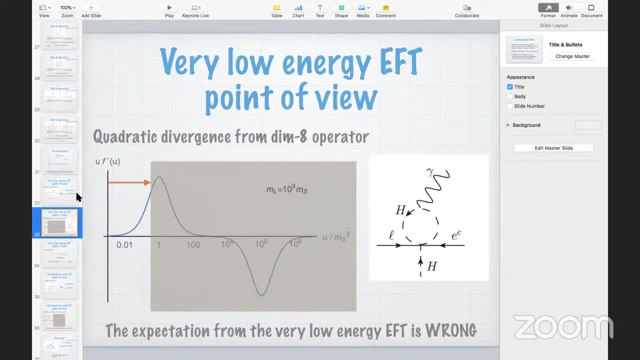 and therefore have to. So I think the problem still stands. even though your statement is true that from the UV point of view, you can make it obvious, The question is: from the IR point of view, can it be non-obvious? 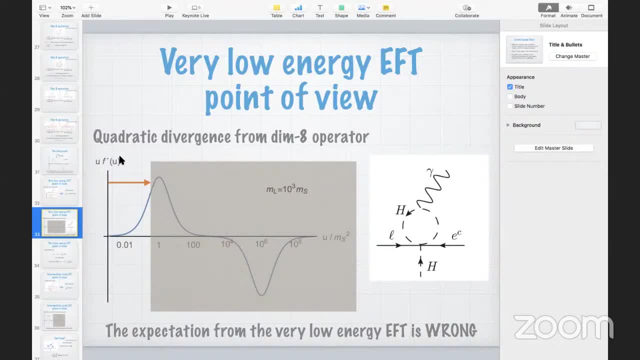 But you cannot do it without you know, kind of fixing the CV right In certain sense. Well, you know, if you say that if I do power counting for low energy point of view, I expect that theories in this class are going to have a divergence. 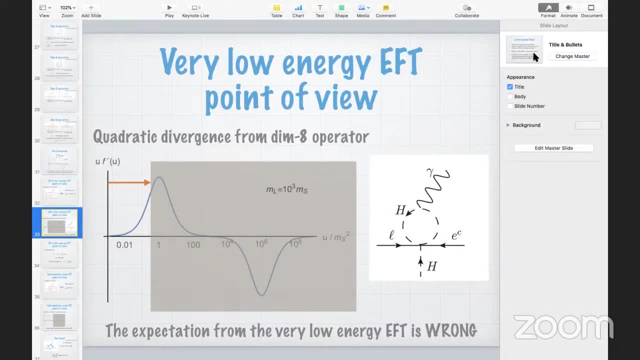 And then there's one subclass that has a natural cancellation, But I haven't discovered that yet. But I haven't discovered that UV class yet. Then, as an IR theorist, you might think that, naively, all theories in this class are going to have this problem. 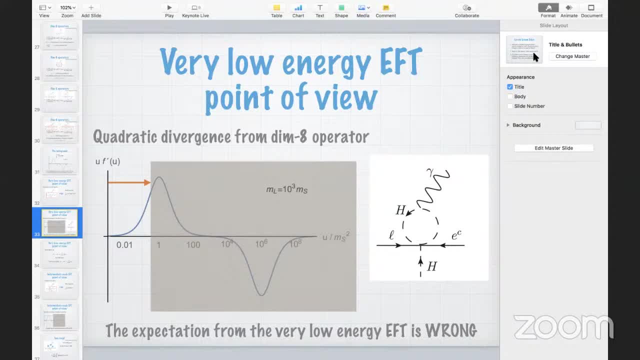 But then there's a really interesting subclass that doesn't have the problem. That's kind of what we want for the Higgs right, Because there's some class of theories which, even though you naively expect that all the arguments about naturalness are correct- 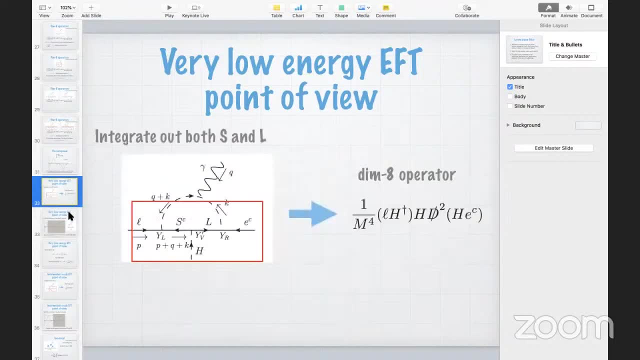 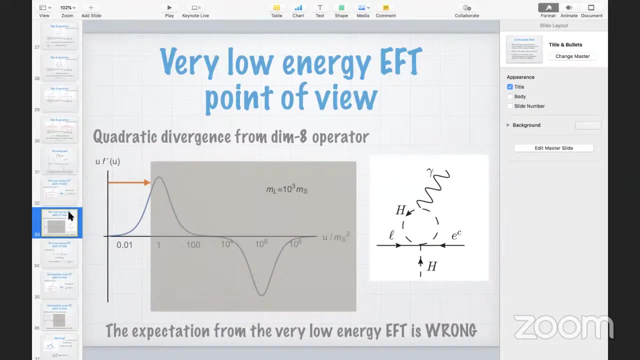 it's not a trick, obviously. No, no, no. But in this particular example, Matt, I believe that here the theory is fixed right And in this particular, in this particular example of the theory which under construction, 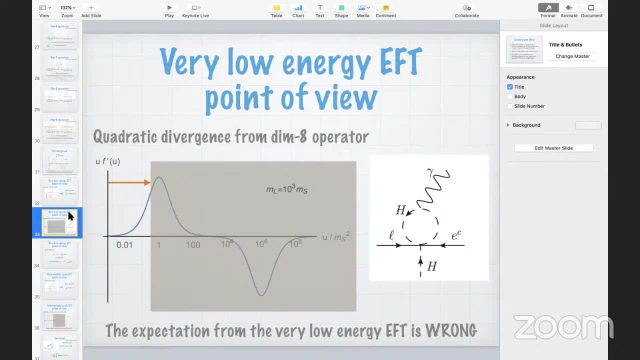 which ultraviolet finite well defined In this particular theory. I'm looking for the term which is one of, say, heavy mass square. No, I mean implying that this term is calculable, right? I mean it's not that. 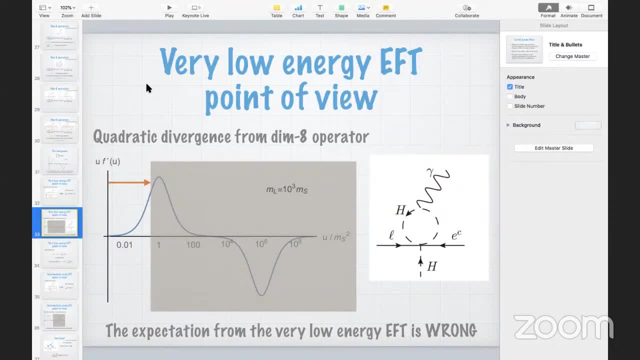 it's not defined. So when I believe that it's calculable then I can try to, because if it's finite then I can try to do it in turn. So first I am considering three level expansion in one over mass. 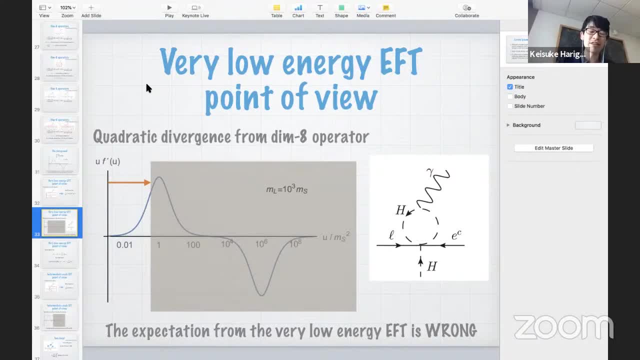 square. Even if the theory is calculable in the minute, you just use a fake field theory. it's uncalculable. You can't just look at a dimension of six. No, I can't, because if matrix element of this, 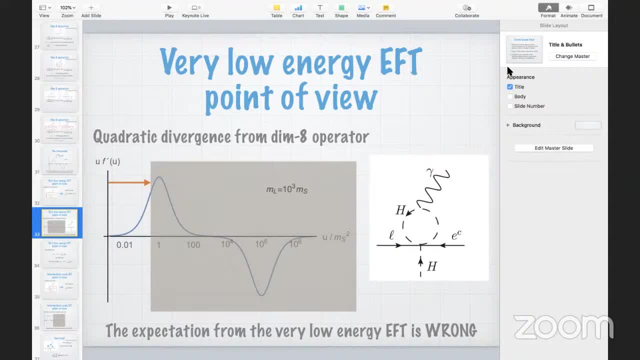 three level expansion is finite, then everything is well defined. You see, because because then I? you see it's useful, because when I'm calculating g minus two, correction from this three level expansion, if I would, will have divergences. 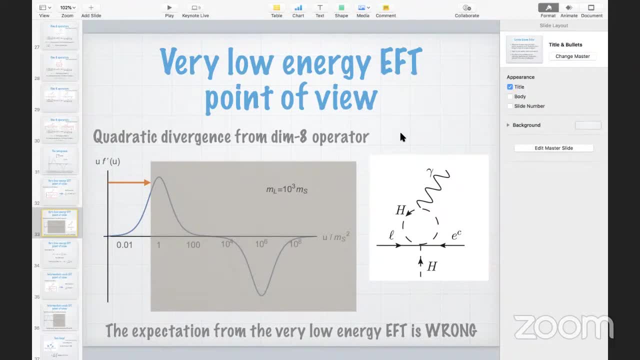 then I would agree with what you said. but there is no divergences there. I'm trying to say: this matrix element is finite, And then then everything is well defined. What I don't, what I don't understand, is why you can just say that this is finite. 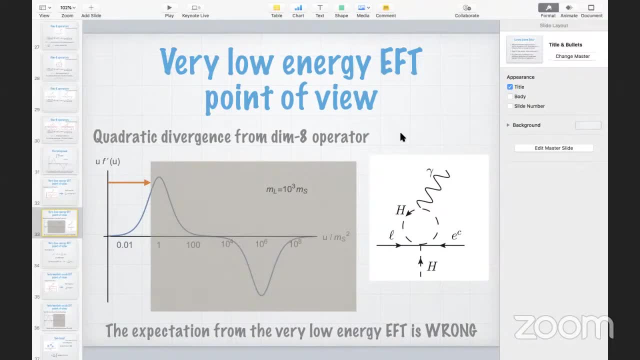 even in the I tried to complete quantum correction. No, no, no, because I, because I can calculate matrix element and see that there is no divergences for this particular operator. There is no divergences. No, no, no. 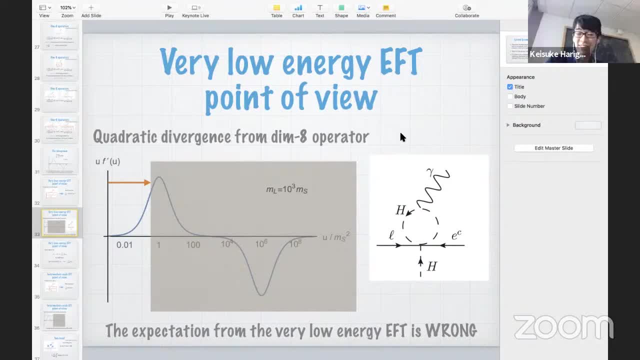 but if you start from dimension eight operator, then the divergence, then everything is uncalculable. Okay, No, let's start first of all, dimension six operator. We have one of m square, we provide a certain operator- And I'm saying that- matrix element. 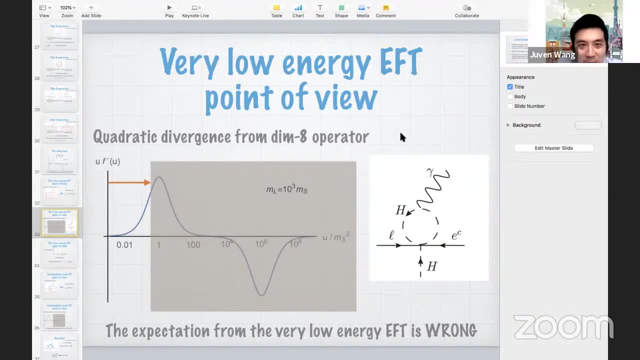 of this operator is finite. But, but wait, but I don't understand what you mean by a dimension six operator. you know, Maybe. maybe let let other people ask first and then, if Kekuke has time, we can. 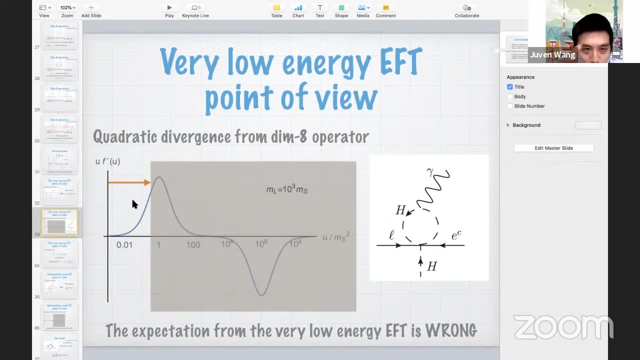 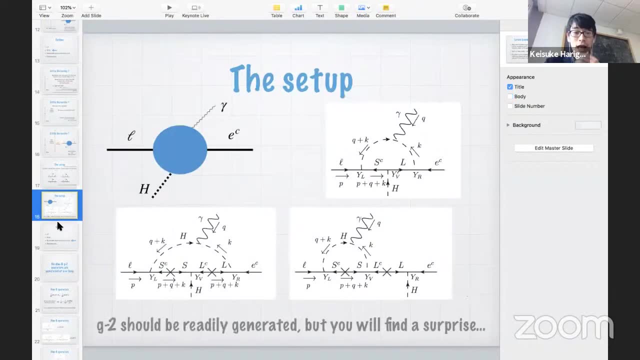 we can. I do have a question, Okay. Okay, Let me ask. sorry, Yeah, I have a naive question about global structure of your model. So we have a, we have a three generation of lepton and quarks in the standard model. 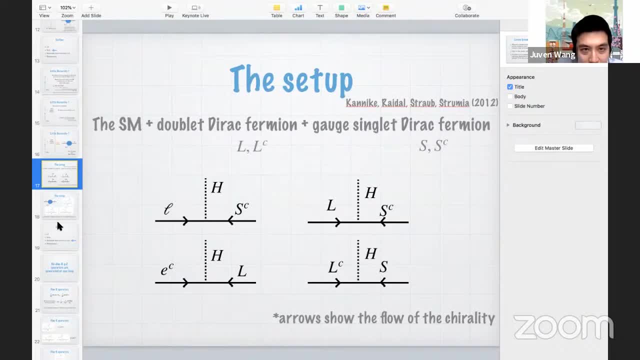 Do you how many generation of this new fermions, the capital L and S, you introduced? Just to explain to me, on G-minus two, it is enough to use just one set of this particle. yeah, okay. and then my question is that, uh, how this make your? 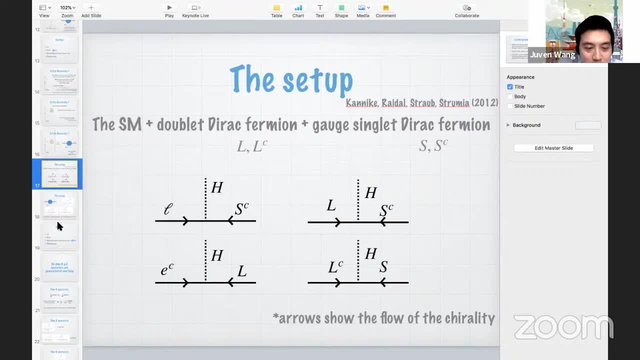 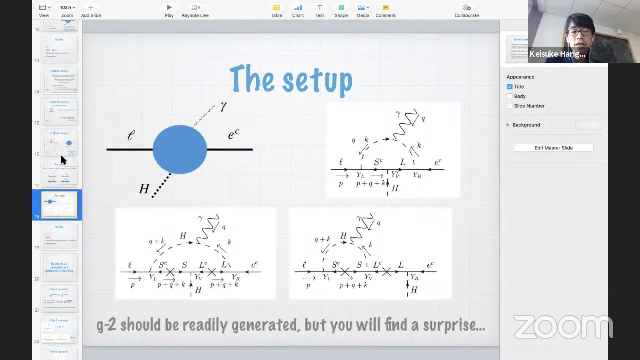 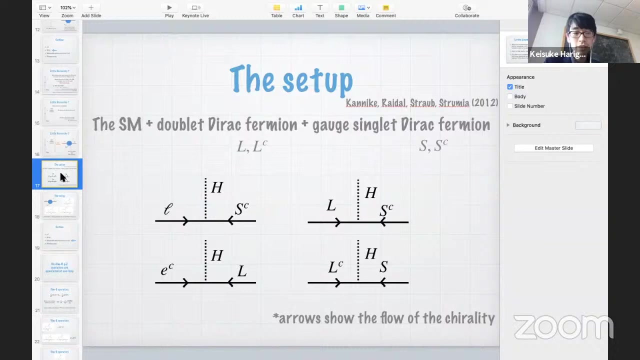 model attractive. maybe are there some other reasons maybe make your model. you believe that that makes. maybe makes make it, uh, maybe. maybe there are some fundamental reason you believe this might be an argument. whatever, this could be more interesting if we can explain the yukawa couplings radiatively. so one question is in the pattern you start model is: why is there a hierarchy? 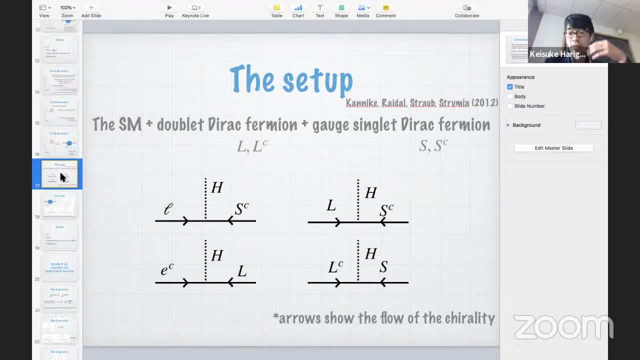 between electron. you got coupling, you got coupling and that's how you got coupling. so one idea is that you can capture your first two generation comes from the quantum corrections. so if we could succeed it in that within this kind of model, that could explain the pattern of the flavors and the model. 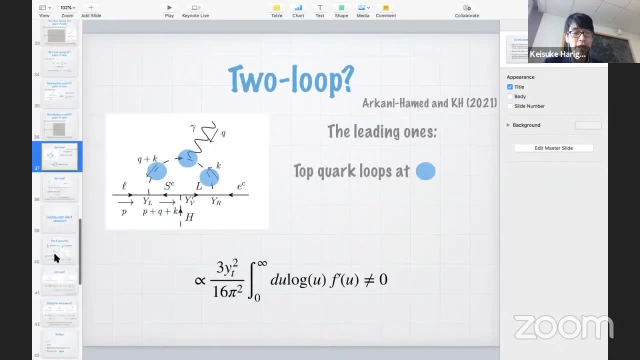 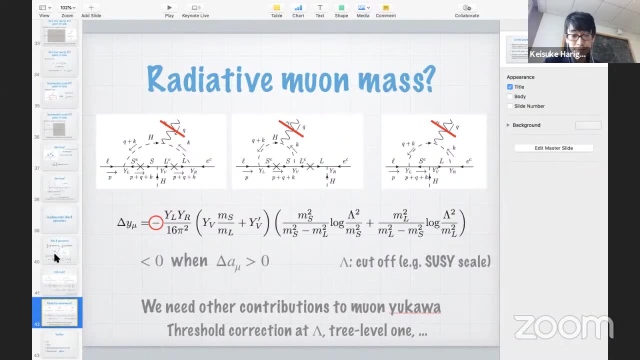 can be more interesting. but unfortunately that i explained at least from the higher correction. so we cannot obtain a correct sign of the mu yukawa coupling, so we must rely on some extra uv physics, so to to to make this more interesting. so maybe we should. we should construct a field. 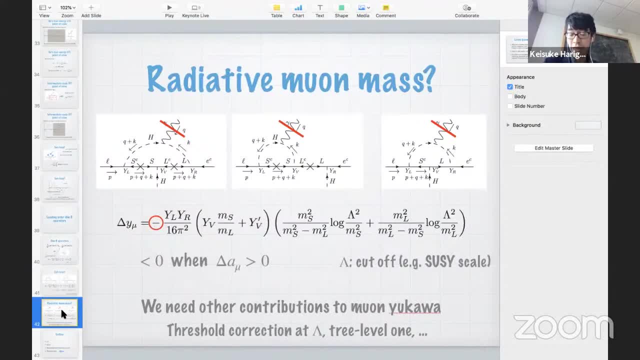 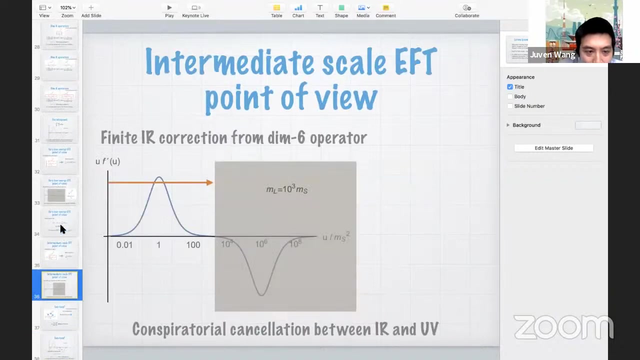 of view where actually new, correct, new math is obtained. okay, and i also have a question about: it seems like you introduced some marana marana mass coupling between the, the s s fermions. is that right? are these crucial? uh, majorana mass, what do you mean by my? because? because you have s and sc. 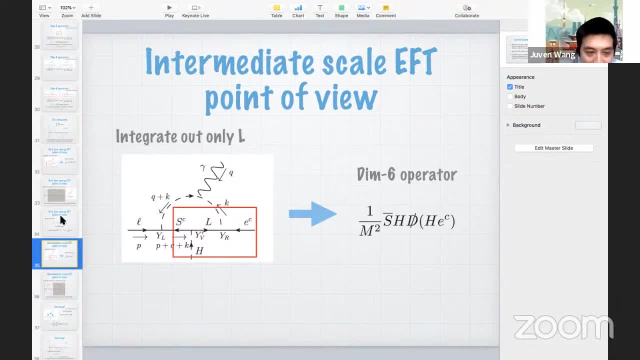 maybe coupled at least on some type where you do have s and s, c. ah yeah, i introduced direct mass s s conjugate. yeah yeah, just just the wrong mass. yeah, yeah, as if we introduce minor mass. i expect there is some quantum correction to the neutrino mass. 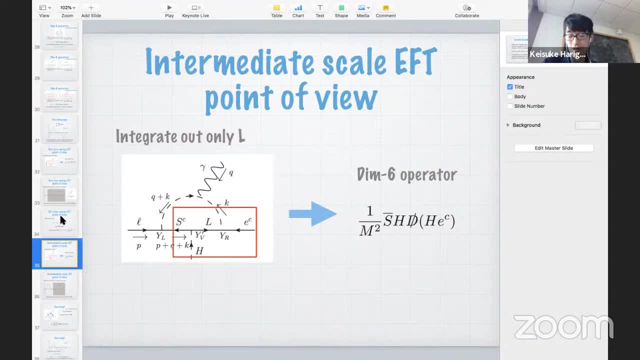 dynamo neutrino mass. so there will be some strong upper band on the just minor mass. so i i just put it to be zero. okay, all right, thank you. so i had another question, just, and it's related to the thing i was asking before. i think you showed in one of the slides. 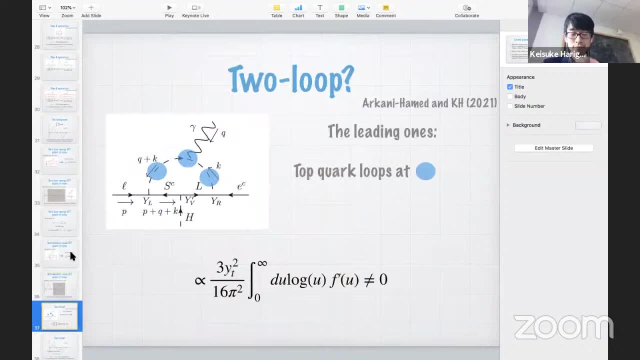 that the two loop does not have this cancellation. um, now, is it possible to twist around the uv model to make it cancel at two loops? or is it true that if you made it cancel a two loop, the one loop would not cancel anymore? like, is it like? how much can you push this accident in the ir? 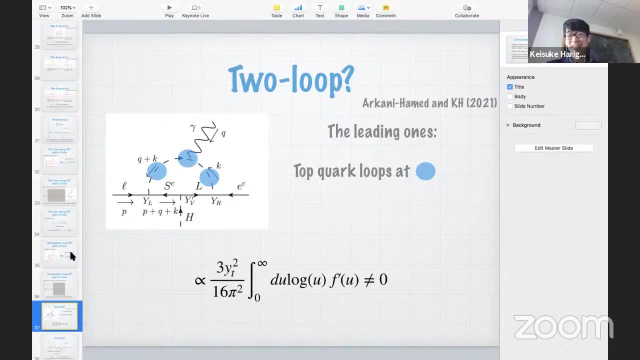 theory. have you thought about it? just, i have actually no idea if you guys like me just to do it. yeah, my suspicion is it is it will be very difficult, yeah, but yeah, maybe we should think of or think about that direction. maybe you are imagining the pushing up the, say, electric cutoff scale, new 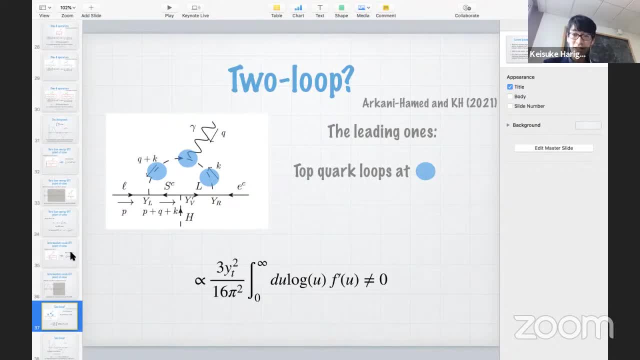 electric, say, even higher than 1 to 10 tv. so, yeah, yeah, i don't have any good idea. yeah, that's my honest answer. phenomenologically, yes, but even from this aspect of understanding the uv ir structure of field, like how much, how much wrong can we be? is there somehow that we cannot be that wrong, or can we? 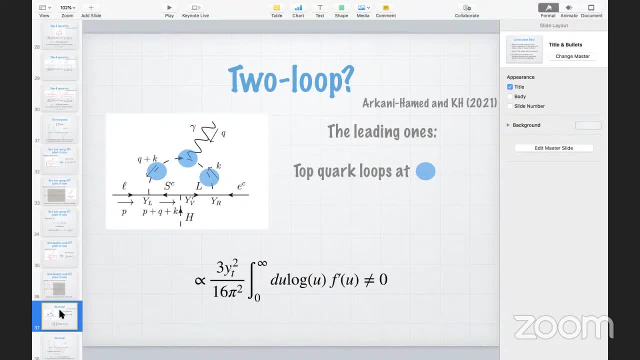 be crazy wrong and it can happen at i don't know arbitrarily high or something like that. so uh-huh. can i just make a remark on that? that means it sort of relates to the question i was i was going to ask next: you haven't given us, um, i mean you've, you've argued to us clearly that there's no. 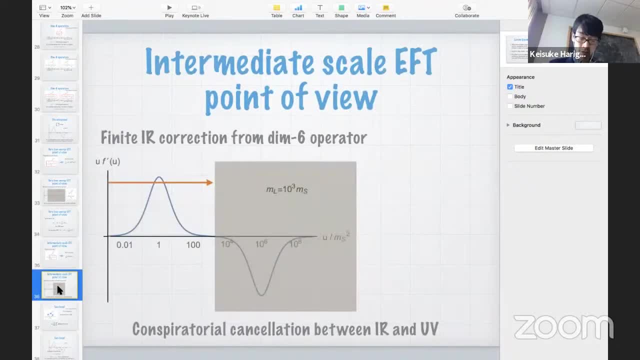 symmetry that forbids these things. right, but in the case of of little higgs, for example, there are suppressions that come from a spurion analysis. i'm sure that you and nema thought about that. you didn't find one- maybe there still is one, and- and so i think 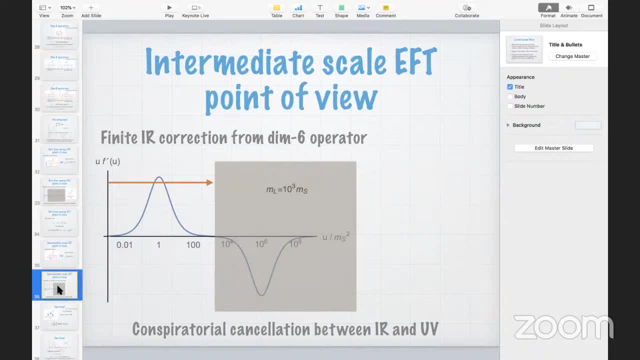 rashmi the, the key here would be to explain why the one loop cancellation occurs from some more principled point of view, and then you would have a chance of understanding whether it could ever continue. but but this, but this relates to to, uh, i think, a question which is both relevant, for i'm 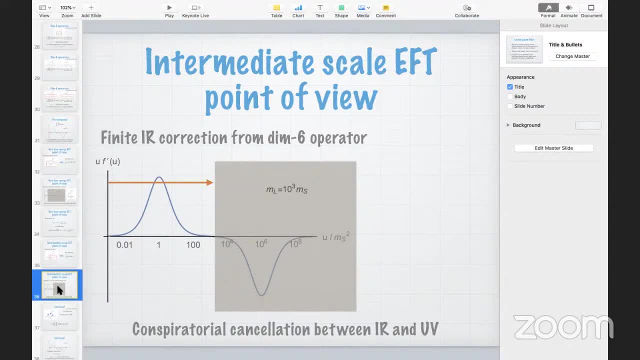 akadi and rashmi, which is, if we indeed considered theories like this one but also doing the second higgs double. we have a much wider class of theories, and we can track them from the ultraviolet, we can track them from the, from the far infrared, and think about what's happening in this subclass. 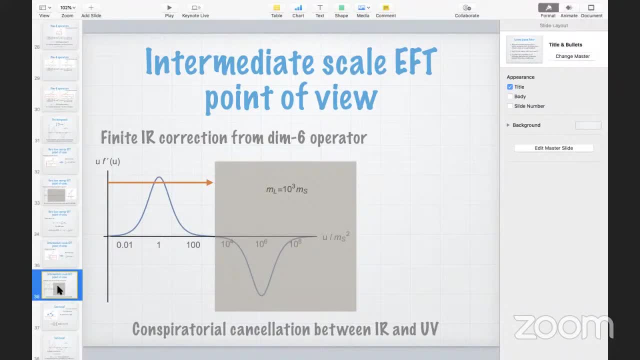 where either the second uh set of higgs is decouples, due to couplings going to zero, or their mass is going to infinity. when you discover that in low energy, in the low energy theory, something interesting happens, but we don't know why yet right. and so, from the low energy point of view, why is this subclass different from the other class? 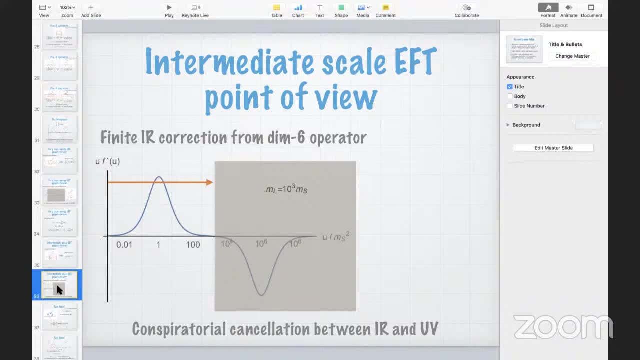 which you know, you just threw in some scalars and some and some lepons. you write down all the effective operators you should have and something happens to coefficients for a reason that is not yet determined by either symmetry or a spurion. so that's kind of where you know, that's kind of where 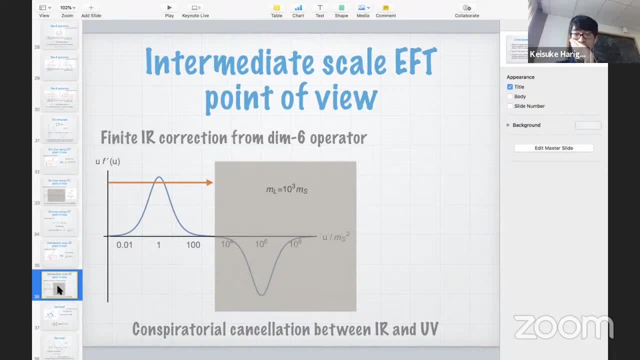 i think the attention needs to be. yeah, but, matt i, i i did try to argue actually that if you consider this, uh, okay, in this particular theory, uh, possible intermediate operator, uh, uh, i mean, which appears there like linear, uh, quadratic in in fermion field and cubic in in higgs, you are, you are finding out. 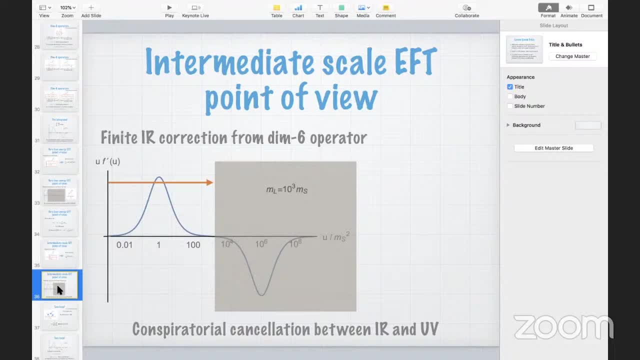 that, uh, this, uh, it's not a surprise. it's not anywhere, it's just a statement that, um. it's not a surprise that, of course, you understand that there's also a point of view, and so it's not a surprise that you know these things are very minor, and that's a proof of the fact that. 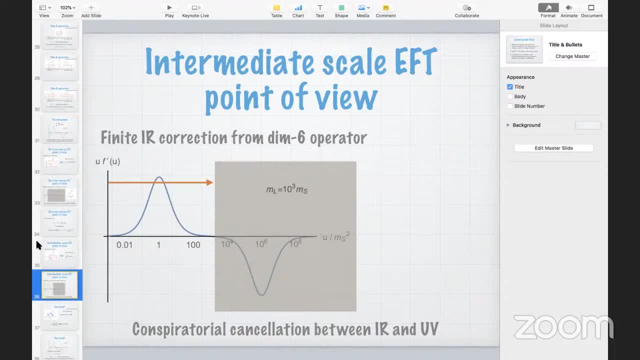 you know it can be done, but i think the argument is going to be that if, for instance, with no close ∈h, that's okay, but in this Class V theory it's going to be that if a function of uh, simply this is something that is not necessary, because it will be basically a natural reaction. 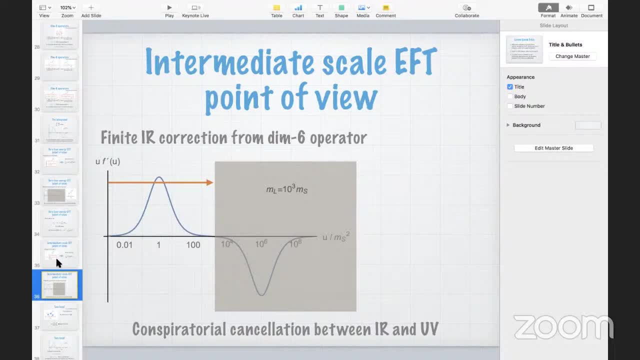 ammions contributed. because if they contributed only in the way when they are mixing this spin zero state for leptons, then you could be sure that it's not a problem. I agree that it is in a certain way I'm fixing from, but I'm fixing it at the three. 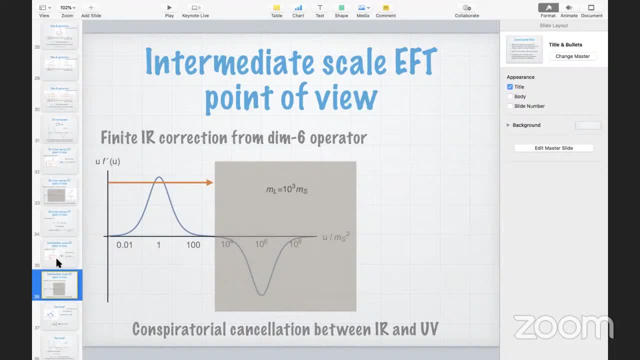 level expansion in heavy quark mass right. Moreover, when we are talking about this higher dimension operator, the physical operator we are looking for, it is dimension five operator, right At the end of the day, if we knew, I multiply by mu bar, mu right. 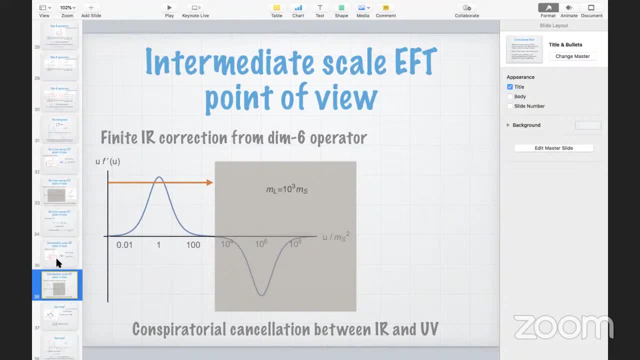 And what we are calculating? we are calculating coefficient for this operator right At the end of the day, And when, for example, you are talking about dimension eight operator, this dimension eight converts themselves into additional smallness in this coefficient, because coefficient. 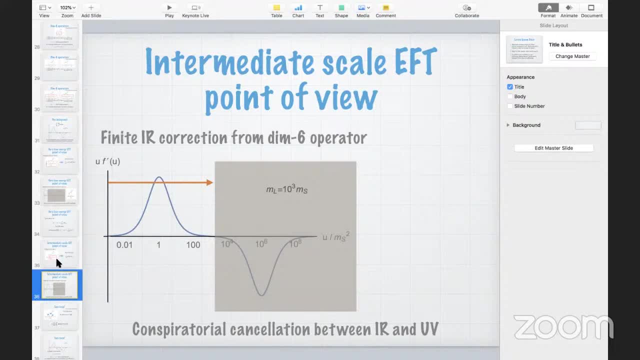 was a mu squared divided by capital M. Now it is a mu squared divided by M squared multiplied by M, double U squared divided by M squared. Okay, so in this way it is the equation: how to calculate from UV complete theory coefficient for dimension five operator right. 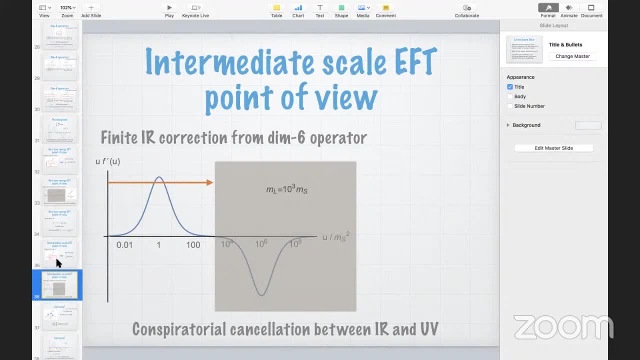 At the end of the day, And, moreover, your calculation refers to a smaller contribution, right, Not a mu squared over M squared, but an additional M double U squared, And that's why, in some way, it seems to me kind of very strange to hope that it would. 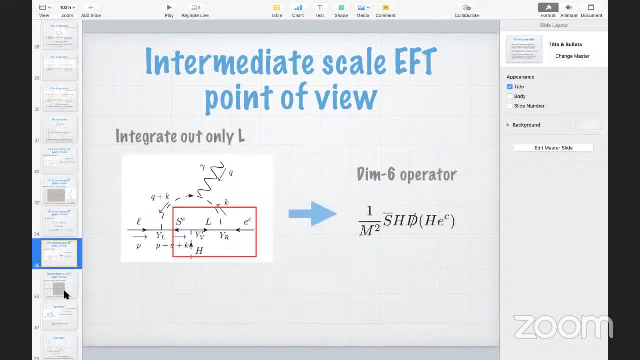 help phenomenologically, You see, because it's more suppressed. Yeah, for phenomenology, it's a direction where the experiment can be more easily discovered. Yeah, yeah, But we don't have higher signal. Yeah, yeah, Okay, but in this sense, Matt, I see your point. 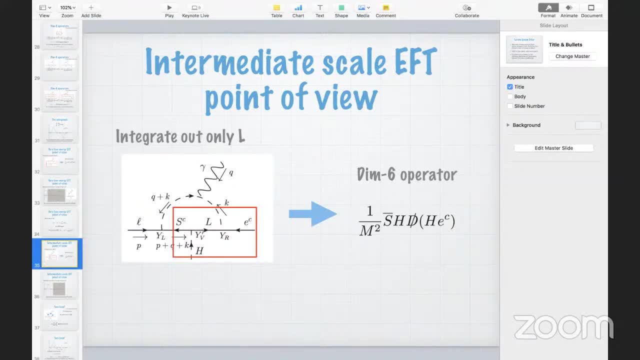 I agree, But in this way. I mean, I'll say once we are calculating this stuff, which is small coefficient for the same dimension, five operator. I'm not sure that it is this type of problem you are discussing. No, that's why. 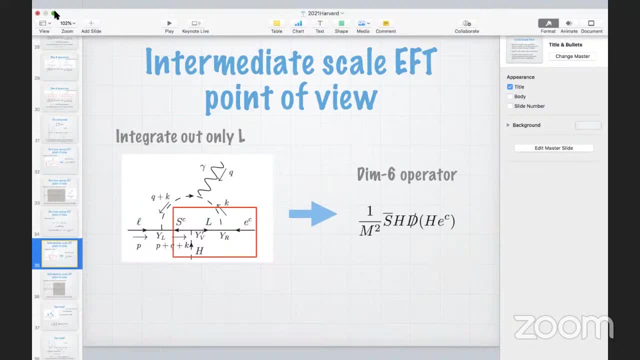 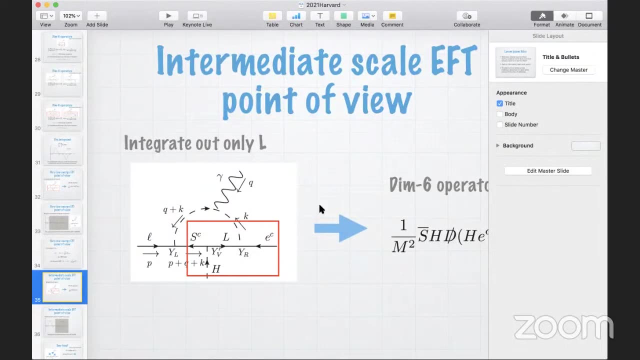 I mean, you know, there's two points of view on this talk and on their paper. One is okay, this is interesting for G minus two. It gives you a different way to think about it. The other is: this gives you a different way to think about it. 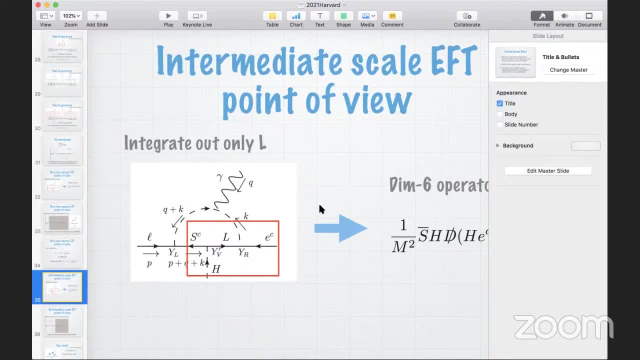 It gives you some Some reason to think about naturalness a little more carefully. Okay, I'm sort of taking the second point of view and not really learning from G minus two, And there the issue is: okay, what kind of mistakes can you make as an effective field? 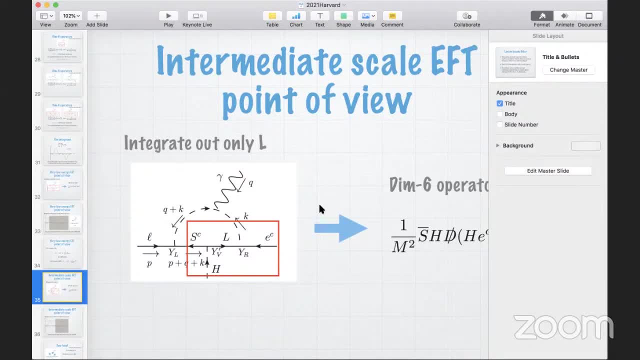 theorist by not understanding what a theory can do in terms of the operators that it can generate. I know about, I know about Spurian analysis, I know about symmetry. So is this, is this a third thing, or is it really a secretly Spurian analysis that I? 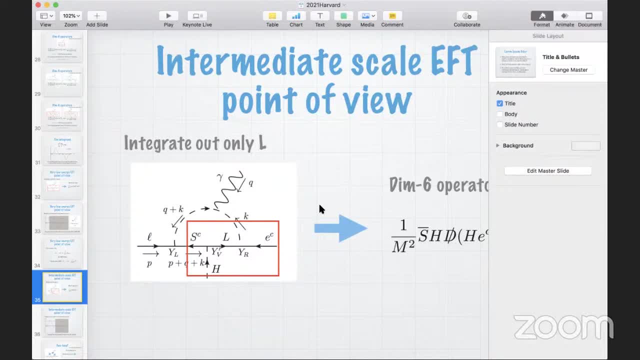 could have known already from Little Higgs. Okay, I would say I agree that it is a third thing, And the third thing being that That it is A certain class of operators cannot be generated. Yeah, Yeah, You see that in a special kinematical structure, right? 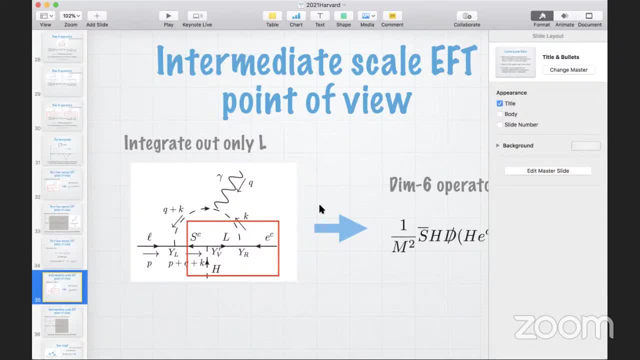 Because you are kind of bilinear in the field in a certain way, In in in Mionic field in a certain way, You see. So so I think that it's a kind of a very special case. Yeah, It still smells to me like maybe a clever, you know. slight generalization of Spurian. 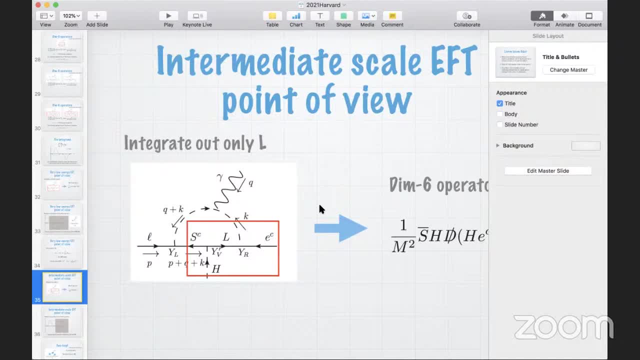 analysis would tell you that. I mean somehow analysis, Yeah, Yeah, Because you you can kind of introduce proper Spurians right, The one which would be sensitive to this. Yeah, That's, that's pretty much the. that's a good question. 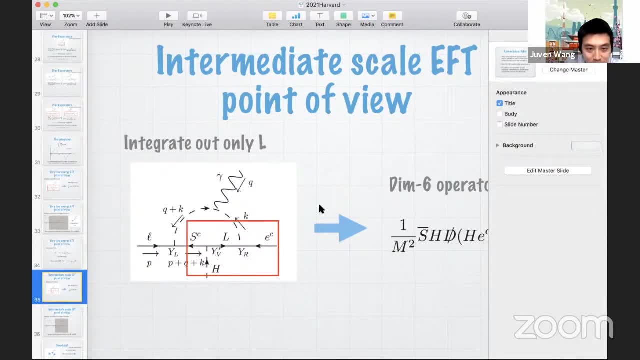 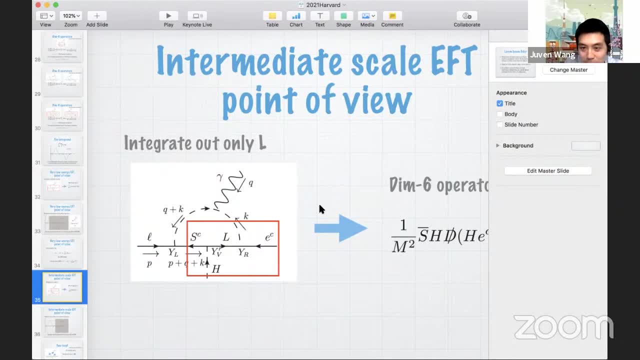 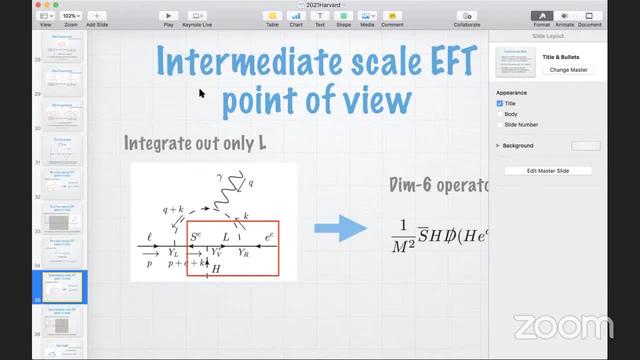 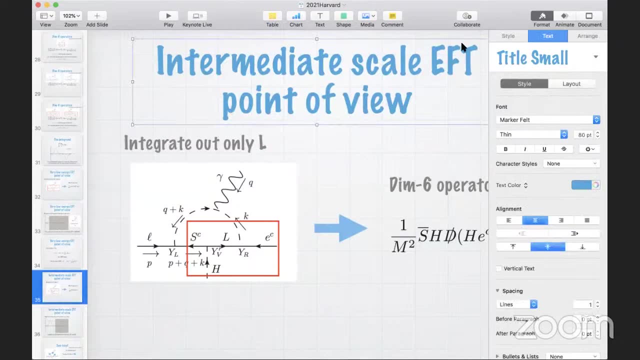 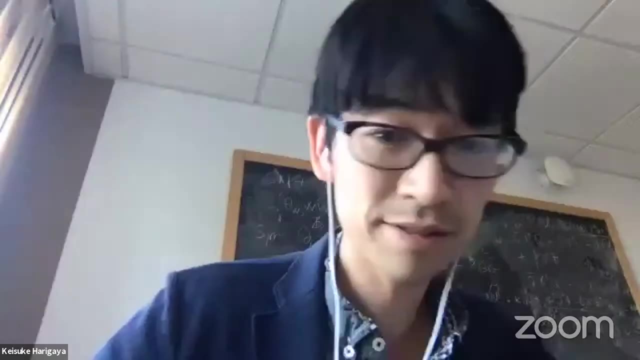 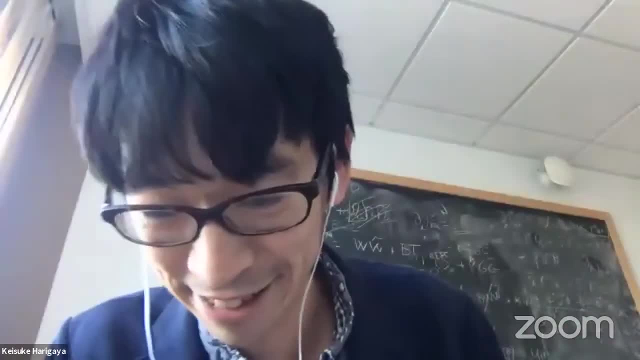